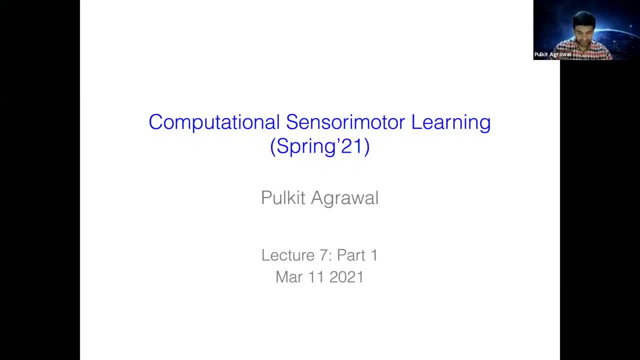 Okay, so today's lecture is going to be in two parts. So in part one we are going to be talking about asynchronous methods, about national policy gradient, and we'll briefly look at the RPO and PPO, which are some state-of-the-art algorithms, And then we will 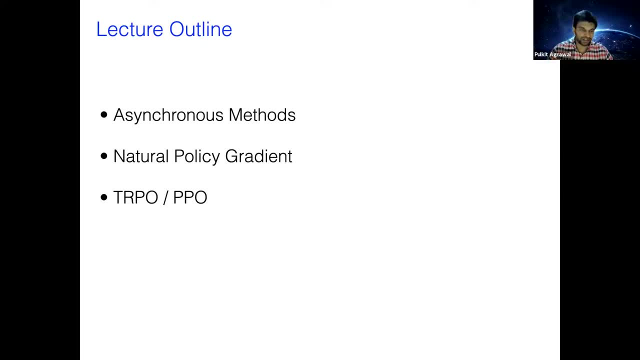 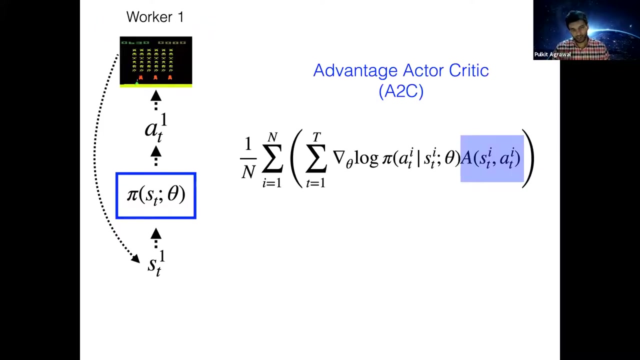 transition into the next part of the lecture, which focuses more on some practical aspects of reinforcement learning. So let's first get started with the first part. So in the previous lecture what we saw is advantage apacritic, which is written down over here where we have the gradient term on the right, and it's an illustration of the policy. 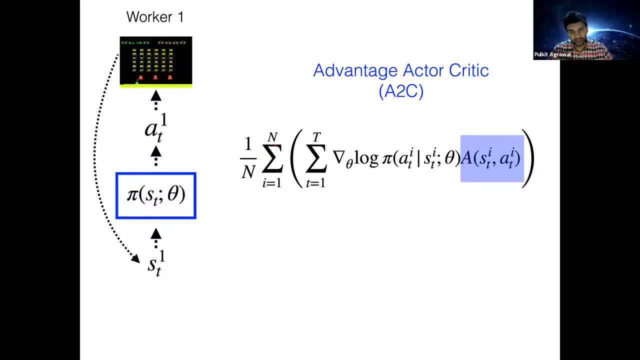 on the left And we saw how we started off with the sum of rewards And finally we ended up with the advantage function as a critic to get the gradients right. So now, typically, instead of just using one worker from which we are collecting data- it is very common to make- 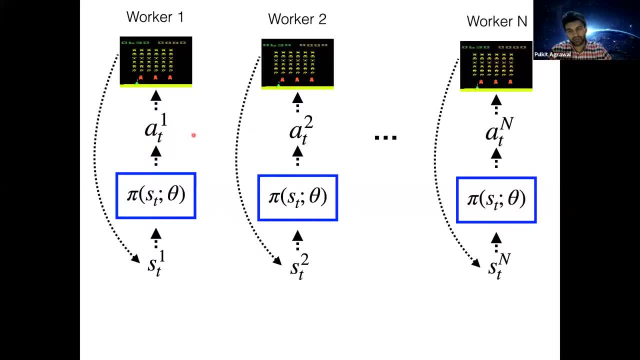 use of another worker or many more workers, right? So typically what I could do is the same thing. I can have n computers or n CPUs on which I am rolling the policy independently on all of them, but with the constraint that the parameters between these policies are. 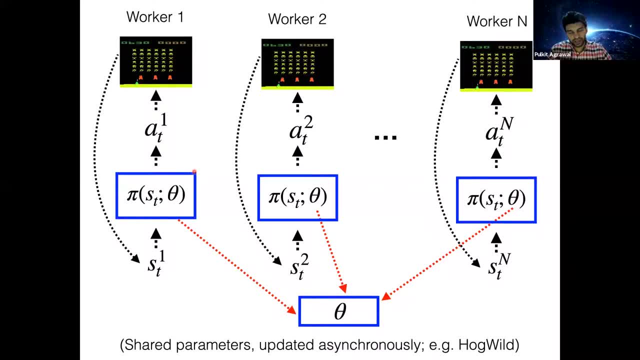 shared. So you know we have shared parameters. So each agent is, you know, executing a policy in the environment, collecting some data, updating the gradients and sending it back to the environment, And then we can also use it to do some other things. So, for example, 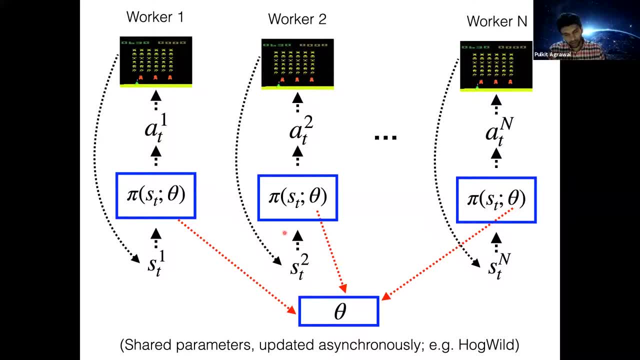 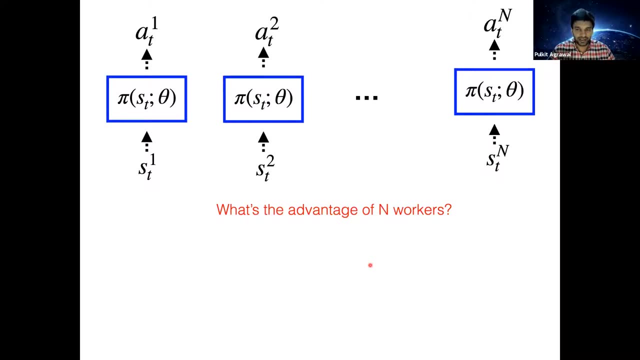 let's say, if I wanna只bs package to a central place which gets updated, and then that new weights are saying to all the workers, are all the agents which are there right? So now one question we might have is: what's the advantage of n workers? And so why not? 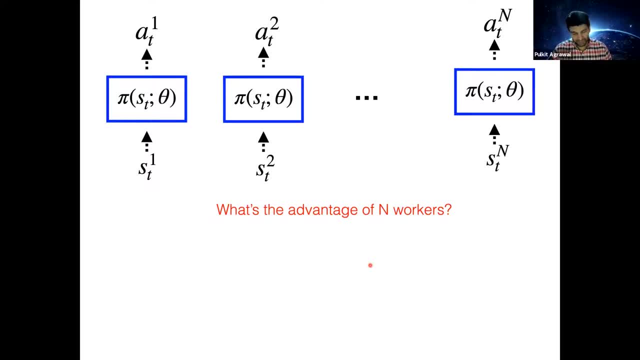 just have one. why actually have n If this is where we ended last time? Also one more question, wondering if you know anyone has any thoughts into why we, why having end workers might be more beneficial than just having a single worker. so i get one comment on the chat which says: you know, 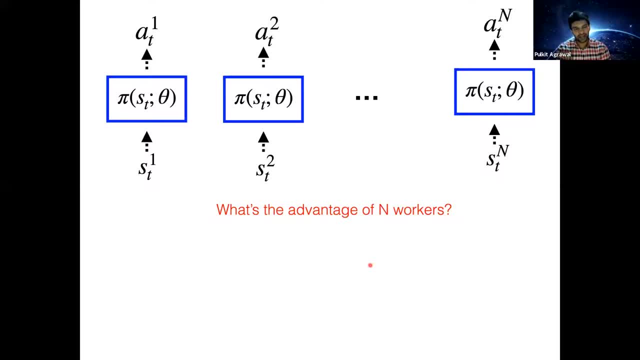 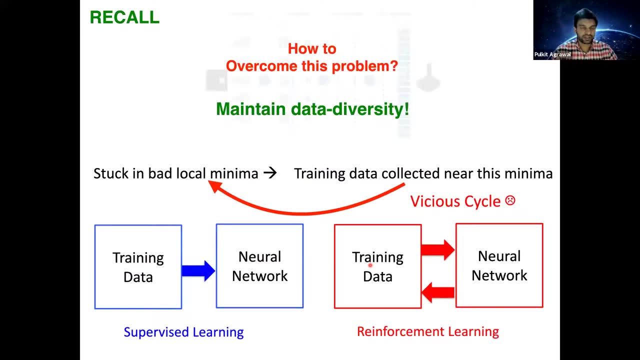 more diverse data in the same time, and i think this comment is spot on. so remember what we saw previously. right, we saw how, in reinforcement learning, it is very easy for the agent to become stuck in a bad local minima. this is because the agent's policy is responsible. 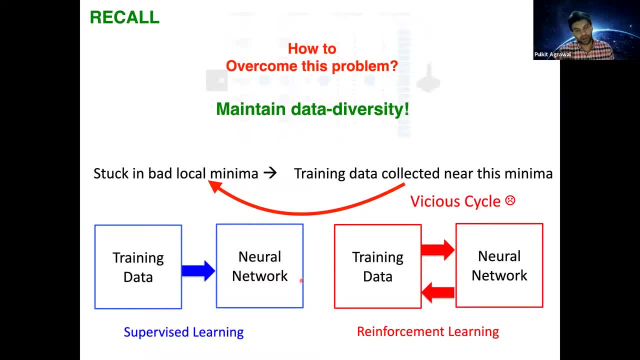 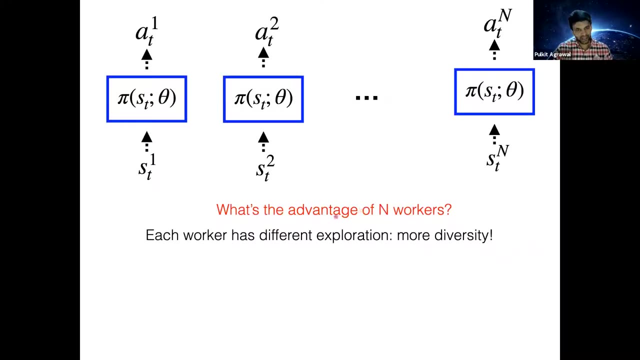 for collecting the training data, and this data then updates the policy. and one thing that we saw was how we can overcome this problem by maintaining data diversity. so, in a similar spirit, right. so when we have n workers which are collecting data, each worker has a different exploration, which means that overall, there is much more diversity. 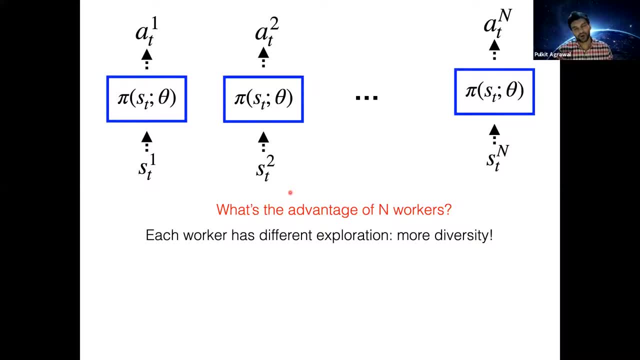 in the data so it prevents the policy from getting trapped into bad places. and to make the diversity be even more typically, there is an additional penalty which is included in the policy gradients objective, which is to increase the entropy of actions. so with that we have this modified objective function where the first term on 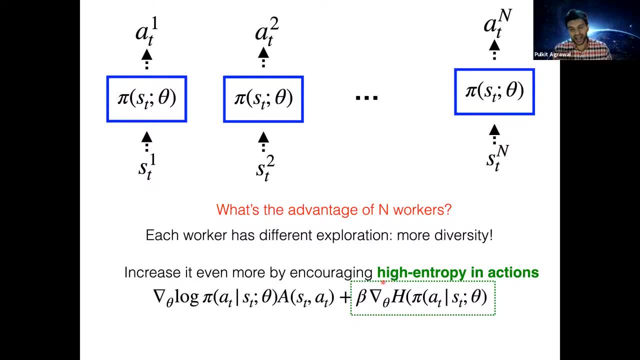 the left is the policy gradient term, and on the right- we have shown in green- is a term which is traitorous to 2 gladiators. so we already saw this in the previous serial model, the church Support Danielle. what can we show here, however? and that is: 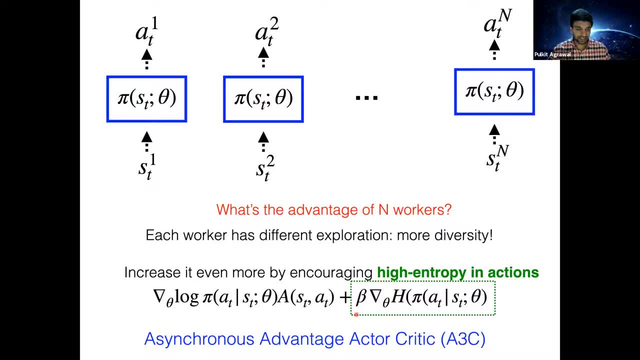 educating agile employees in Kentucky which wetlands alarm workgear versus Iterate algorithm? if you know our team very well, the setup will cause us to yell at you guys. here we are, very the parameters right and you know you can go and see how well this a3c agent ends up doing. 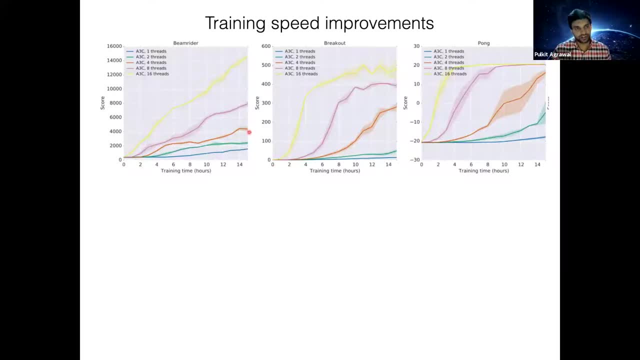 so what i'm showing is some results on atari games. there's some beam rider breakout and pong. on the y-axis is the score one, on the x-axis is the training time right and the comparisons are showing running a3c with different number of workers. so blue is one and yellow is 16. 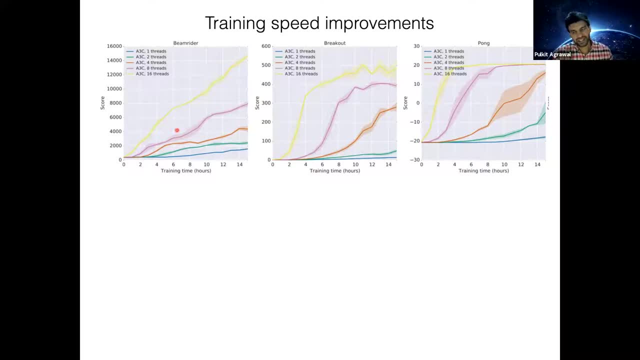 so what you notice over here is that, as the number of workers is increasing, the training is becoming faster in wall clock time. however, if we compute the data efficiency, which means that how many interactions the agent needs to take, and this is summed across, so if there are eight agents, 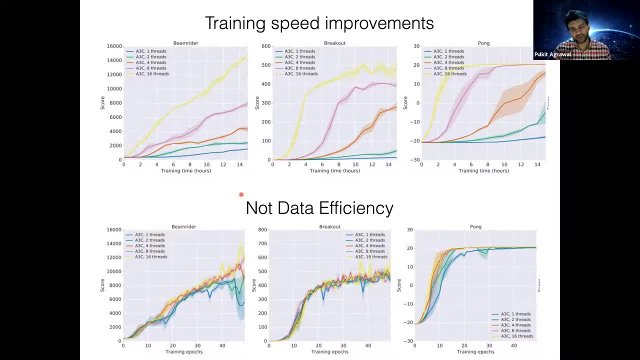 I'm going to sum across a total number of interactions across all the agents. So in that setup what you see is that you're not really gaining in data efficiency, but what we are gaining is in wall clock time. So if something is in simulation, 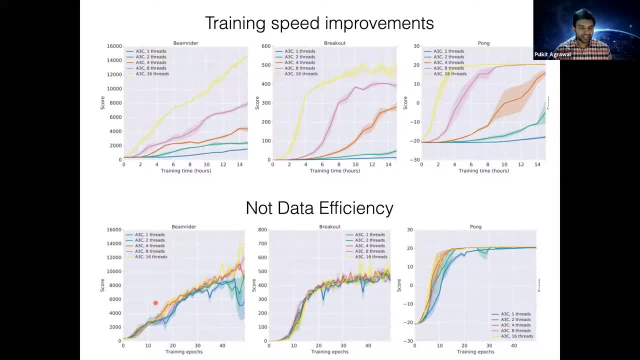 and then it is very easy to parallelize across workers and gain on wall clock time. And you know this is one big advantage which some of these asynchronous methods have over methods which do not use multiple workers. So that's all you know I will cover in asynchronous methods. 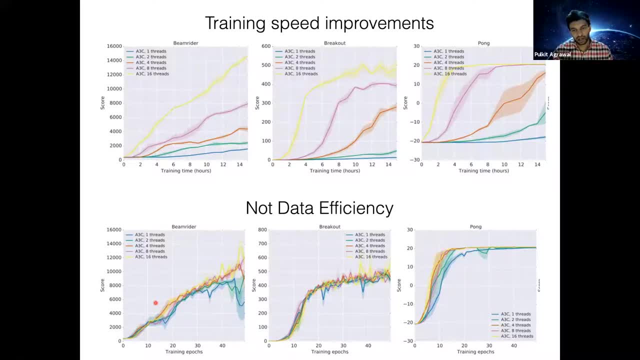 So I'll take a pause and see if there are any questions on H3C or on the asynchronous part. So I see there are two question or two comments over here. Yeah, so Dhruv asked the question. you know will, because all the actors are rolling out the same policy. 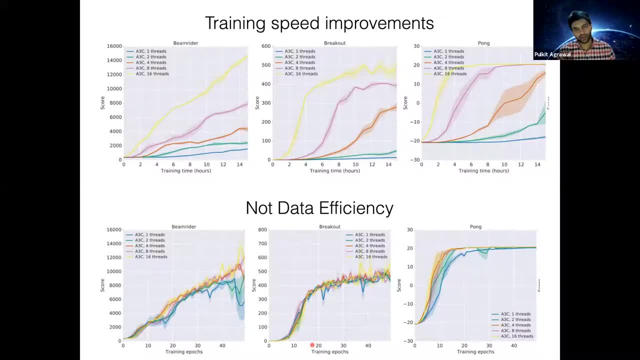 wouldn't they end up collecting the same data? So there is one more term, which is exploration, term which gets added Like, for example, we considered how we can add random noise right to encourage exploration And, in this case, the entropy term. 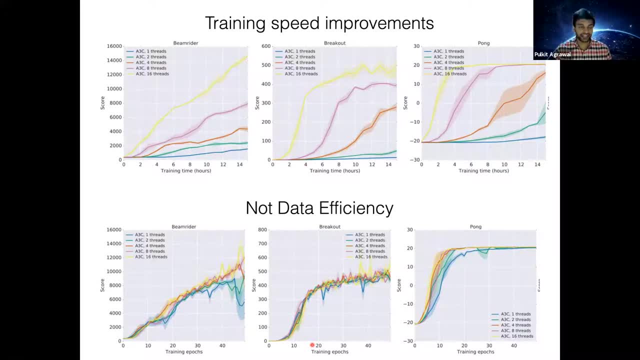 is acting as the exploration bonus or the exploration is encouraging the agent to explore. So, even though you have the same parameters, theta from which you're sampling, there's a distribution from which you're sampling And that is what encourages you, encourages different workers to have different samples. 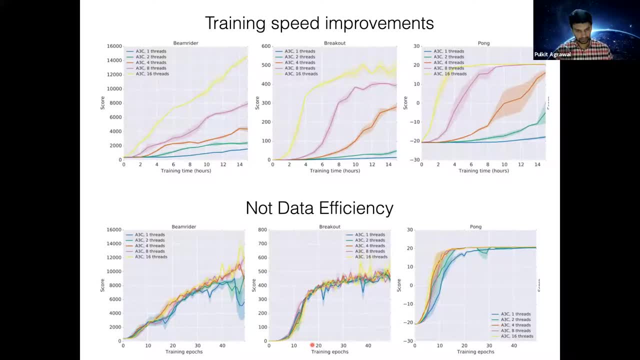 which leads to diversity. Any further questions On this part? No, Okay, Then you know. let's recap a little bit. So remember, we started off with reinforce, where we were summing up the rewards and using policy gradients with respect to that. 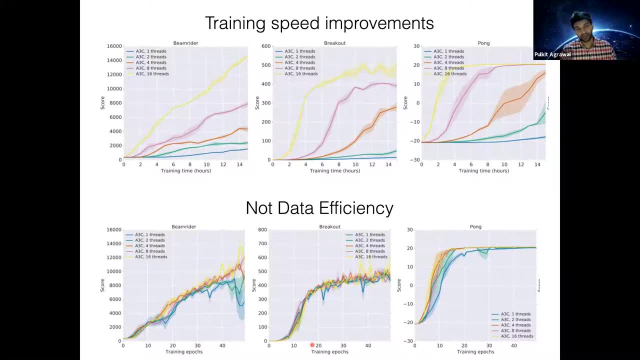 You know, then we saw how we can include baselines and we were using the value function as a baseline. And then we saw how, when we include the baseline, we end up with the advantage function And that is what led to advantage at the critic. 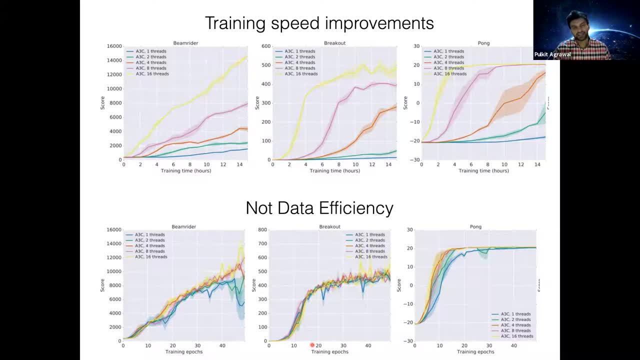 And now what we have seen is how we can parallelize the staining across a bunch of workers which led to A3C. So now, in all of these methods, you know, one thing that we're doing is we have an objective function which is sum of rewards. 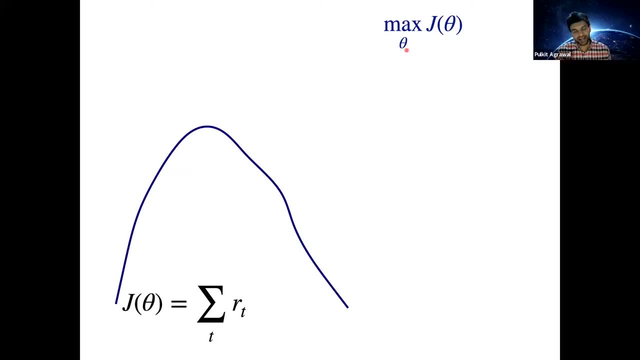 And we are trying to find the policy parameters, theta, which maximizes the sum of rewards, right, And the way we have been doing this is to compute the policy gradient. So how does policy gradient computation work? Right, We are at some, we have some value or some current parameter value. say that is theta old. 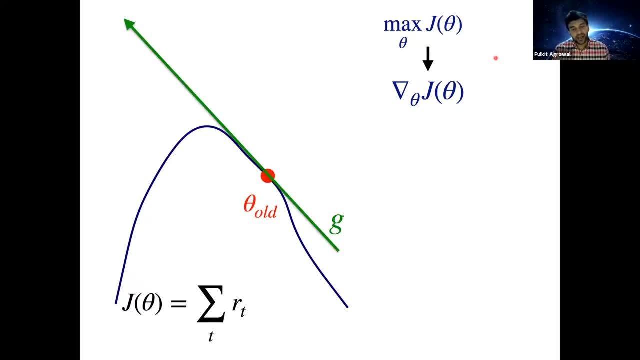 And then we compute the gradient, which is G, And then we update the parameters with help of the gradient, Where G is the gradient And alpha is my step size or my learning rate. So one question which becomes important is: how do we choose this learning rate or the step size? 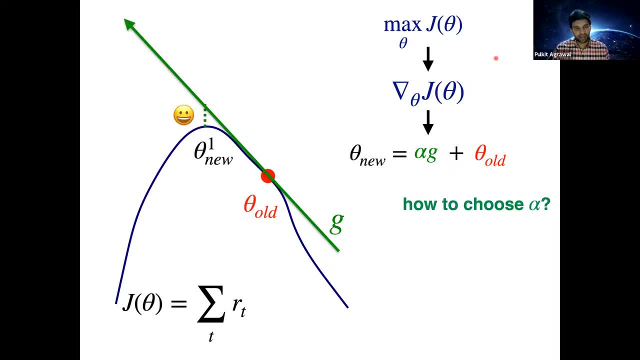 For example, you know if I move in about the right quantity I will end up getting to the maxima of the function. But if I move slightly more or slightly less, you know we wouldn't end up reaching the maxima right. 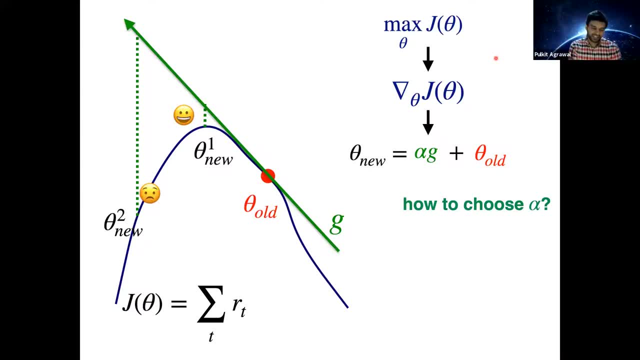 For example, this: For example, we could overshoot and end up at theta 2 nu, at which the performance is worse than what the performance is at the current parameter, which is theta old. So you know, this brings upon the question of how do we choose alpha? 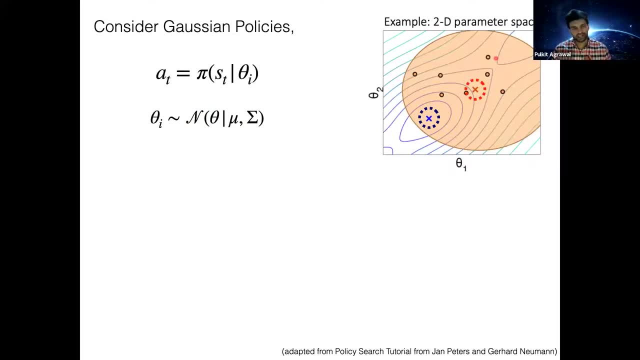 So, to you know, make this be more concrete, let's consider a simplistic setup where the parameters are the same. So you know, we could overshoot and end up at theta 2 nu, at which the performance is worse than what the performance is at the current parameter, which is theta old. 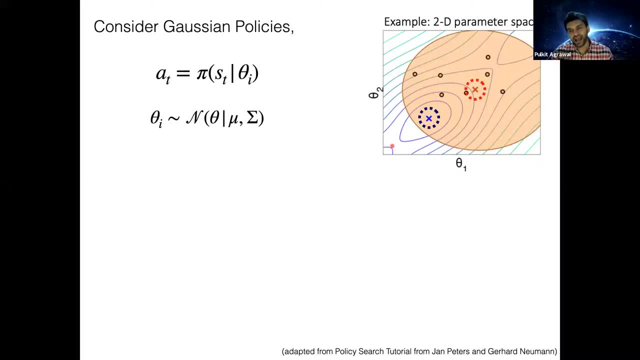 So, to you know, make this be more concrete, let's consider a simplistic setup where the parameters are the same. So, to you know, make this be more concrete, let's consider a simplistic setup where the parameters are the same. So I have two parameters, theta 1 and theta 2.. 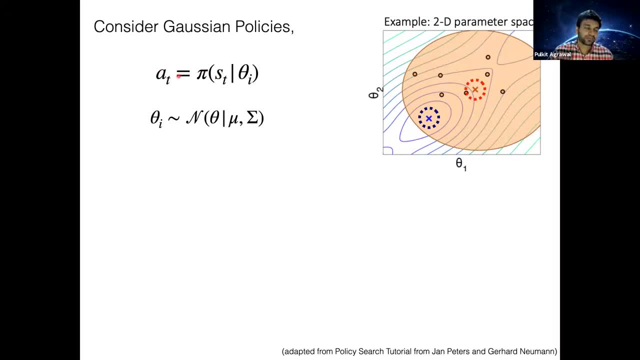 And this is the policy that I'm trying to learn. Let's assume that we are trying. we're only considering the class of Gaussian policies, right, Where what I mean is I'm sampling the parameters theta from a Gaussian distribution. So now you know, what happens during training is that we are collecting some data. 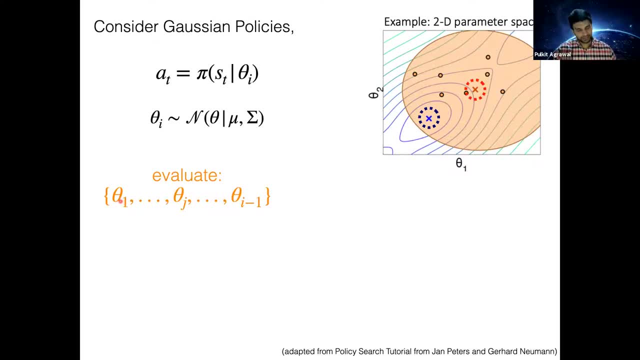 So initially I have theta 1. And then, as iterations are happening, We go from theta 1 to theta i, right? So in this plot, each of these points is showing a value of thetas that we have evaluated, And if the policy is a Gaussian policy, there are two things that we need to evaluate, right? 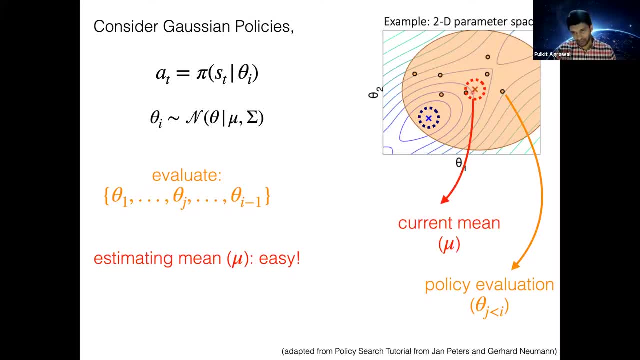 So one is the mean, which is easy to evaluate. For example, the crossover here is showing us the current mean. And there's a second thing that we need to evaluate, which is the covariance right, And it turns out that estimating covariance 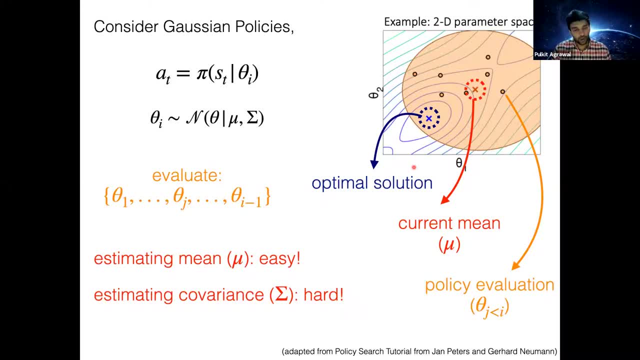 Is actually the hard part And the hope is that by estimating the mean and the covariance we can converge to this optimal solution shown as a blue cross. So we want to start, or whatever current point or current estimate is, we want to move that to the optimal solution. 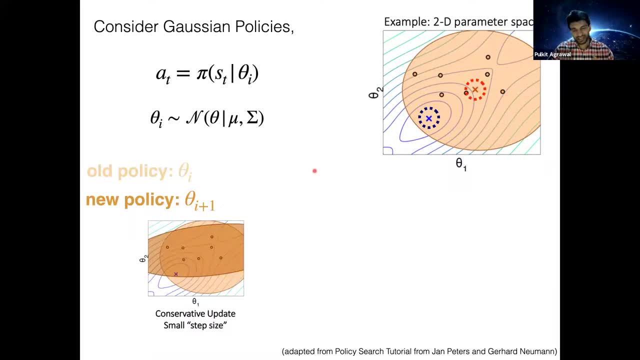 So you know. now let's look at. you know what might happen Depending on the choice of the step size And it's the learning rate. So in this plot on bottom left, what I'm showing in two colors is the old policy and the new policy. 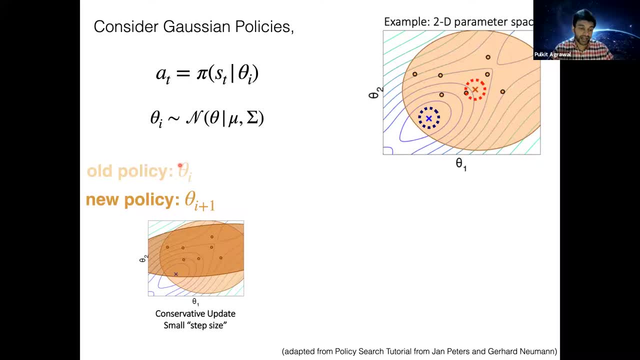 The old policy is in light orange and the new policy is in dark orange. So this is what would happen if my step size is small Versus if I have a large step size. there can be significant changes in what the policy is converging. 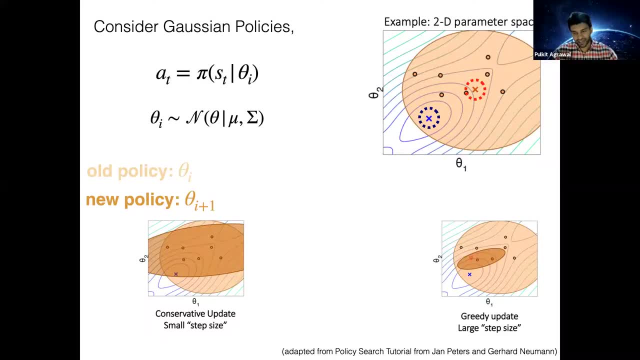 To. So In this case it is getting far away from some of the data points which we evaluated And versus something in the middle which is converging much faster than the conservative update on the left but is also capturing all the data. 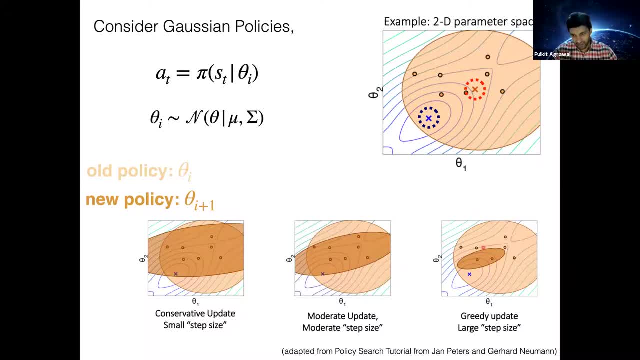 points that we have, which is better than what might be happening if we take a large step size. So when we are taking a large step size- a 2,, which means that our update is very aggressive- that typically leads to a problem: that my new parameter vector is far away from data. 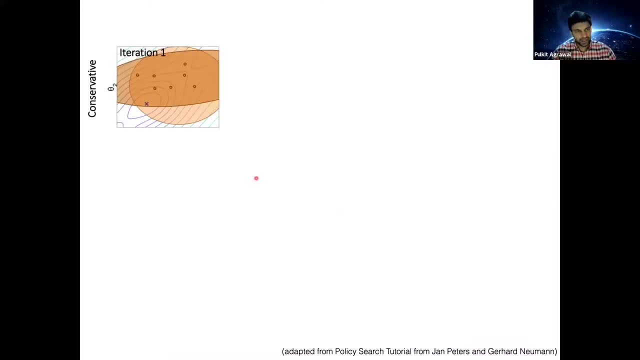 You'll see this visually. So suppose I start off with my theme. I have some estimate of the mean and the covariance denoted by my dark orange curve over here, And then I let this process continue over multiple iterations, Then eventually, as you see over here on the right, most plot. 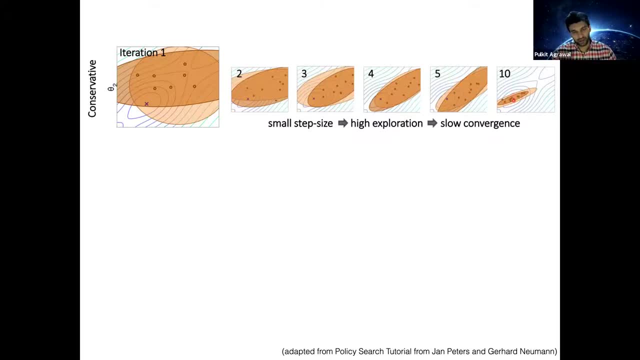 that we are going to converge to the right solution, but we're going to converge to it slowly, Versus if we move very fast, we might end up moving far away from the data points and eventually end up converging to a solution which 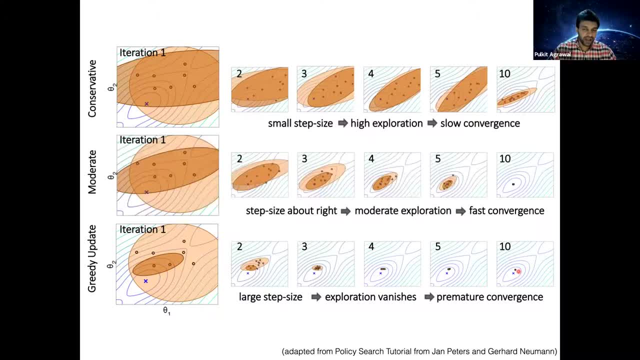 is not optimal Versus. what we want is somewhere in the middle of both of them: Neither too slow, because it's going to take a lot of time, or not too fast, because otherwise we might converge to a wrong solution. So the one intuition we're going to exploit, 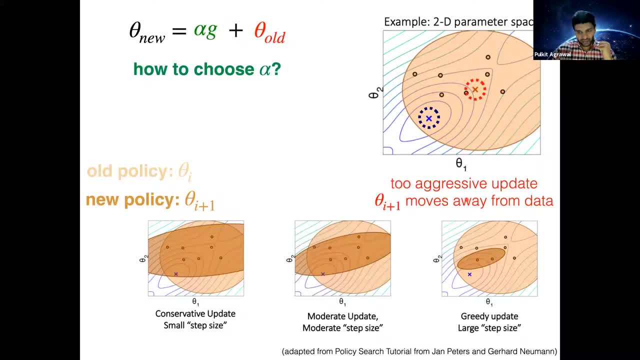 is the fact that, instead of being very aggressive, we are going to be conservative. But the whole game is that we don't want to be too conservative. So how do we choose? the right level of being conservative is what will inspire a set of different on policy or policy. 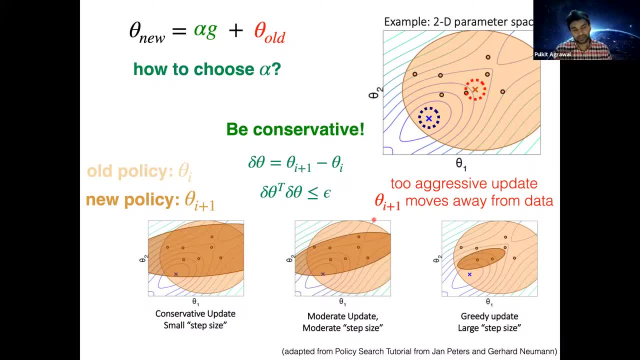 gradient algorithms that we're going to look at. So the simplest way of being conservative is to say that, well, if I'm changing this, If I'm changing my parameters, I should change my parameters by a small amount, which is that I'm constraining how far I move. 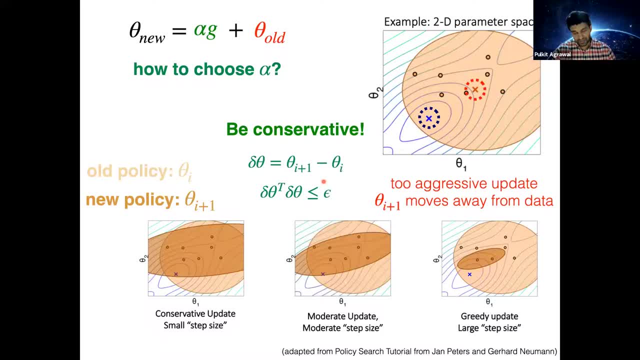 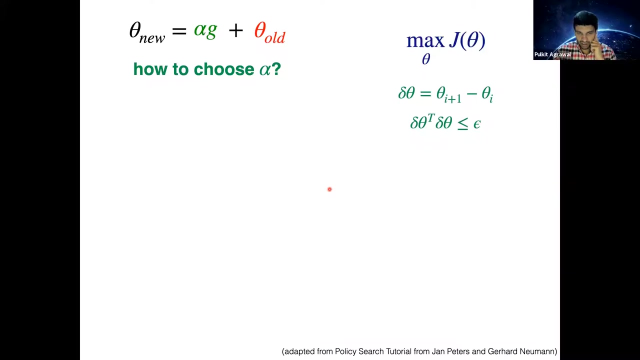 which is directly choosing step size. So this is what we do in vanilla policy gradients or even in A2C or A3C that we have discussed until now: that we can just constrain the step size based on some value that we choose. Now what is the problem with this? 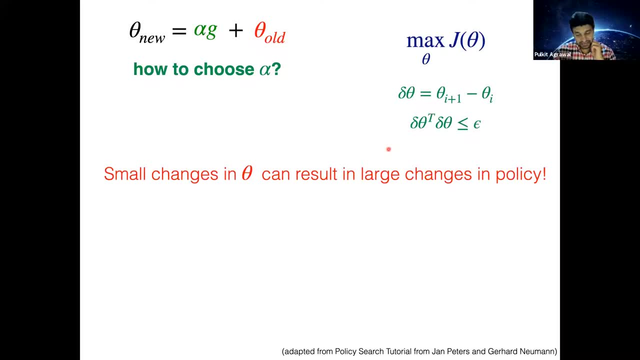 The problem is that small changes in theta can often result in large changes in policy, So I can vary. maybe my theta changes by a very small amount, maybe 0.01.. So I satisfy this criteria. But because the relationship between how, the change in theta 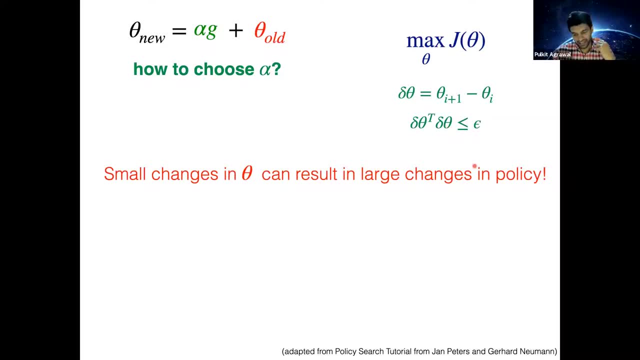 affects the policy is unknown. the policy can change in arbitrarily large ways. So the question then becomes: is what can we do to constrain the policy? So in some ways, what we really don't care about is how theta is changing, But what we really care about is how the policy is changing. 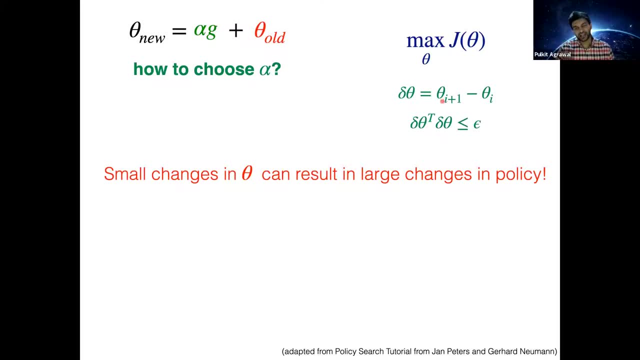 Right. So instead of defining this constraint at the parameter level, we can go on and define the constraint at the policy level. And because policies are distributions, we actually have some good measures which can tell us the distance between two policies. So one such measure is the KL divergence. 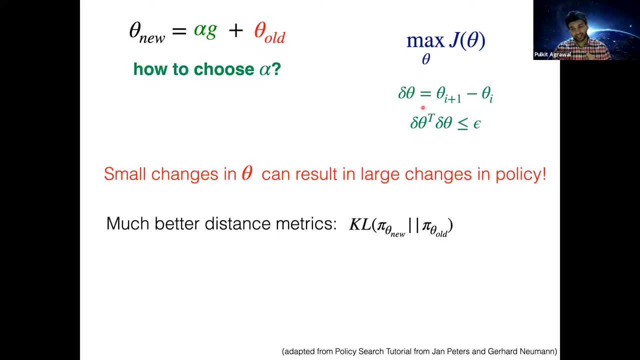 So what we can say is: instead of putting the constraint at the parameter level, maybe will it be better. Right, I want to maximize my sum of rewards, subject to the constraint that my policies are not changing too fast. So now, this is a much more precise notion than constraining the parameters directly. 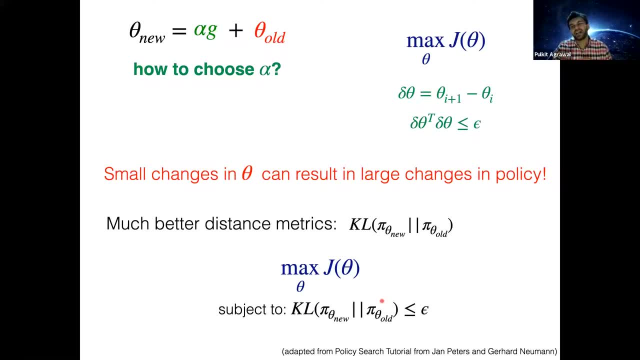 right, Because now I'm constraining how the policy is changing And if I constrain that, you know I can guarantee the policy is not changing too fast. But if I only constrain the parameters, theta, I really don't have any guarantees on how fast the policy is changing. 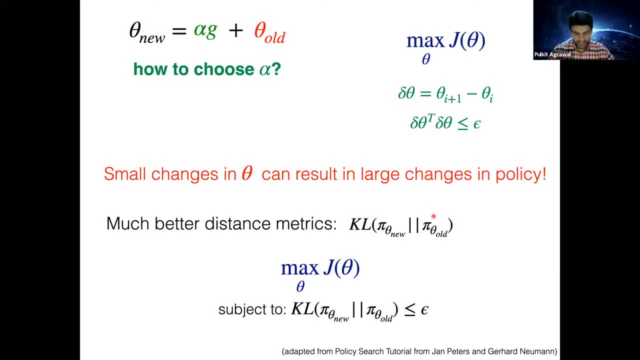 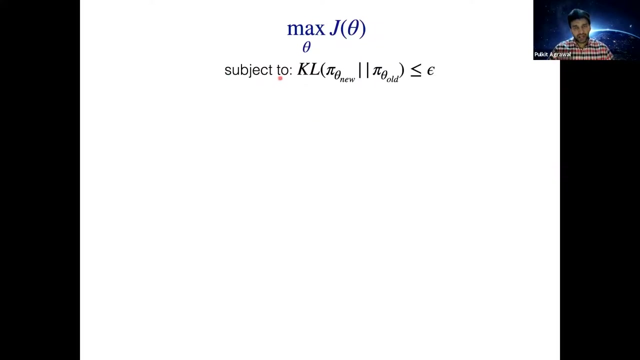 Does this make sense? Any questions at this point? Okay, So let's see where this leads us to. So it turns out that, you know, directly optimizing this constraint, you know, can be a bit tricky, So there are different ways in which this is done. 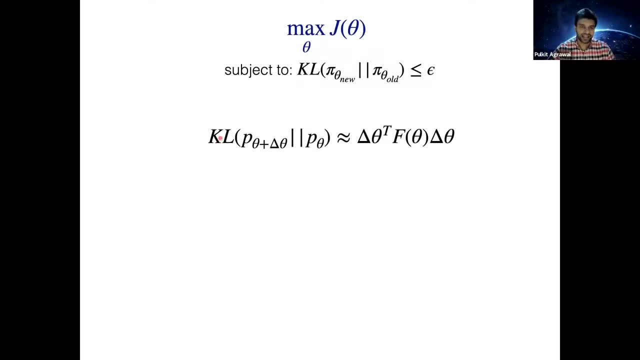 So one way is to make an approximation of the KL divergence term And turns out that if delta theta is small, then we can write the delta theta as a small delta theta. So we can write the delta theta as a small delta theta. So we can write the delta theta as a small delta theta. So we can write the. 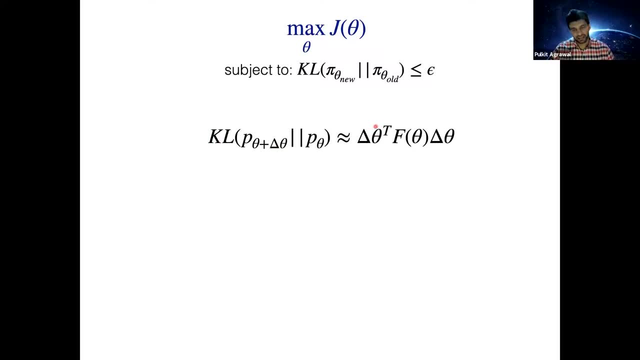 KL divergence as a projection of the parameters theta with respect to a matrix F right, Where this matrix F is also called as a Fisher information matrix, which is an outer product of the gradients right. So if I'm measuring the KL divergence between a distribution P with parameters, 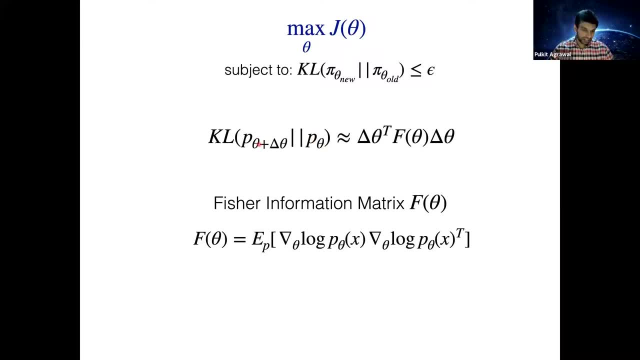 theta and a distribution P with parameters theta, then I'm measuring the KL divergence between a distribution P with parameters theta and a distribution P with parameters theta plus delta theta. Then my Fisher information matrix is defined with respect to the gradients of log of P. 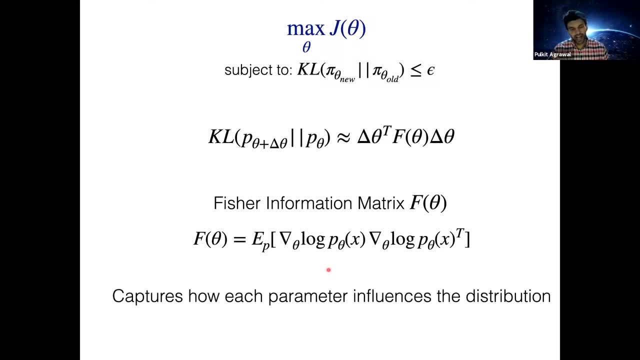 So what this Fisher matrix is encoding is how each parameter influences a distribution right. So if you look at this equation, it is telling me that if I change a particular parameter, then how much is it going to change the KL divergence. So the Fisher information matrix essentially helps me bridge the gap between how the change of 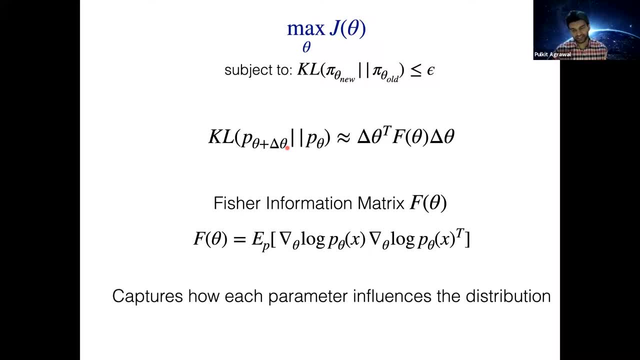 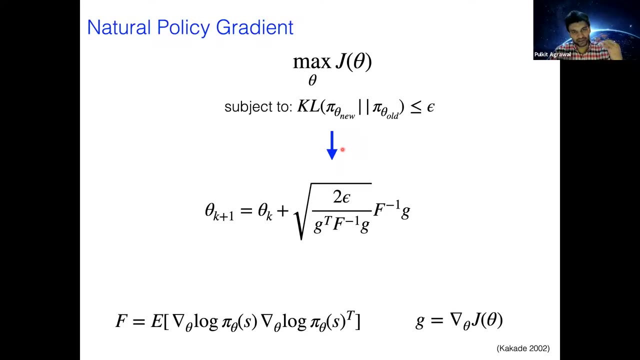 parameters is going to affect how much the policy is changing. So this approximation led to a class of algorithms which was called as natural policy gradient. Now, this was motivated by, you know, natural gradients which, uh, came in, you know, much earlier, but for all but you know, that is just a historical fact, right? 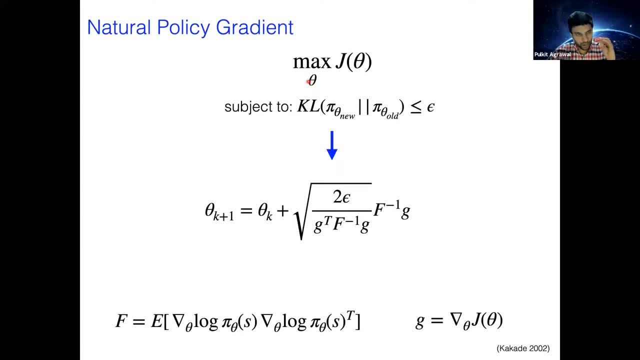 So you know, it turns out that if we use the uh, the formulation that we discussed in the previous slide, which is approximating the KL divergence, we end up with the following update: where F is same as my Fisher information matrix: 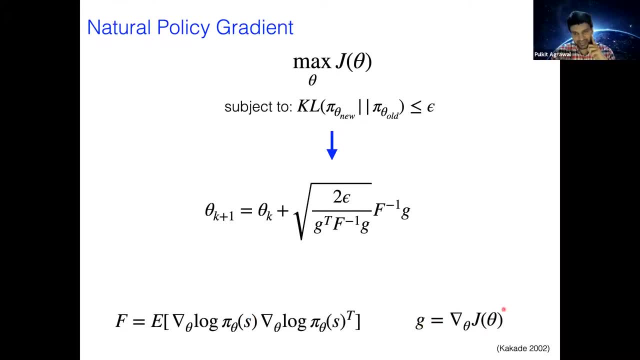 Okay, And G is nothing but the policy gradient term that we have, right. So we're here. we have a term called the natural gradient. So, intuitively, the way to understand the difference between the gradient and the natural gradient is that you know. 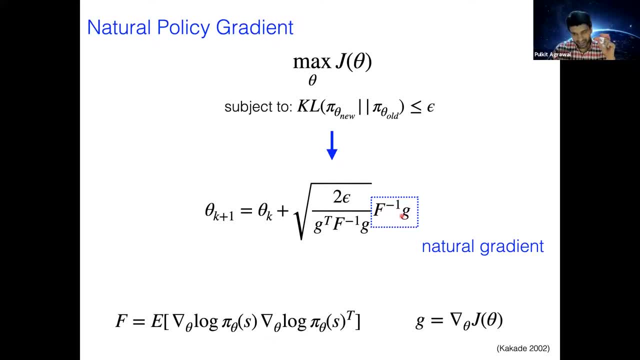 natural gradient is reweighting each dimension of the gradient, with this, the inverse of the Fisher information matrix. Okay, And what this does is it makes my parameter what. what it does is it makes my updates be invariant to scalings of parameters. right. 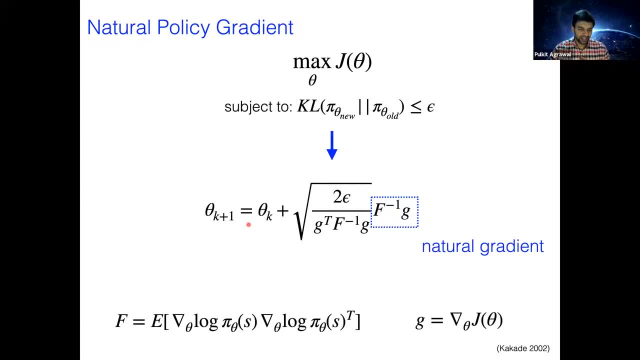 So, for example, you know, suppose if I arbitrarily changed my parameters to be, you know, double them, or I made them four times, you know in, so my gradient computation is not going to get affected by it, right? So it gives me some invariance. 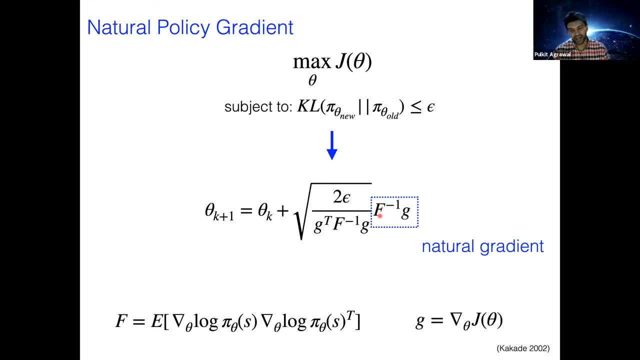 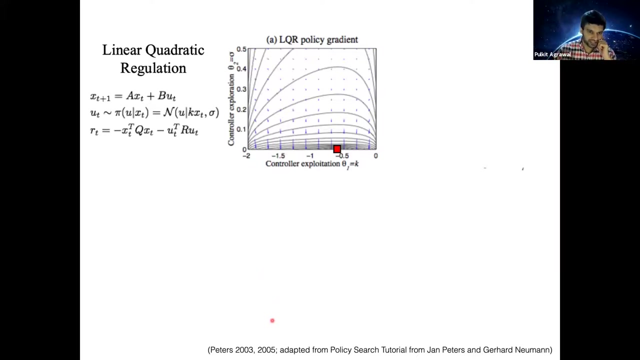 Okay, So what I'm going to do is I'm going to go back to how I parameterize my policy, and the first term over here is the step size. Okay, So now, what does this actually end up doing? right, So we can look at an example, because I'm taking this example from some work by Jan Peters. 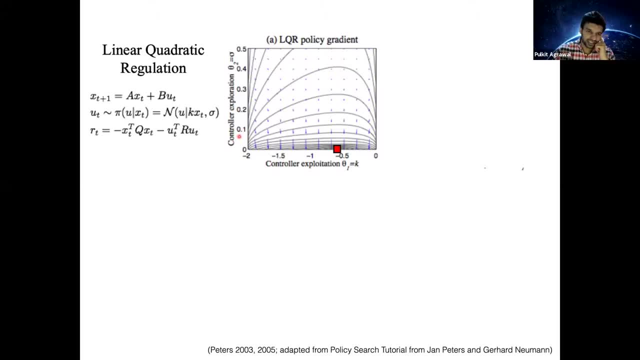 So we have a two dimensional LQR controller, Okay, Okay, So what we are showing is parameter theta one on the right and parameter theta two on the Y axis, And each arrow over here is representing the policy gradient right. So what you notice is that the gradient in this region are very, very small. 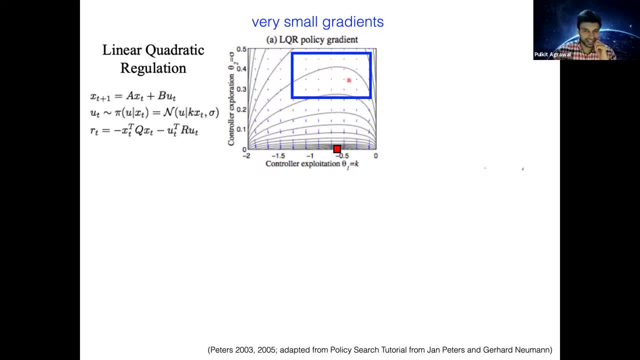 What this would mean is that if I'm starting anywhere over here, it will be very hard for me to move to the optimum solution shown over here. So, but instead, if you were computing the natural gradients, the scaling of the gradients is much better, right. 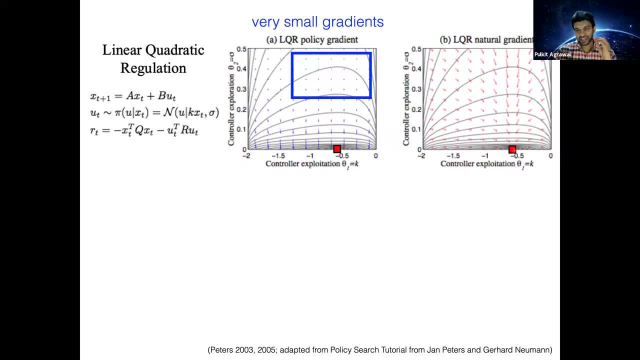 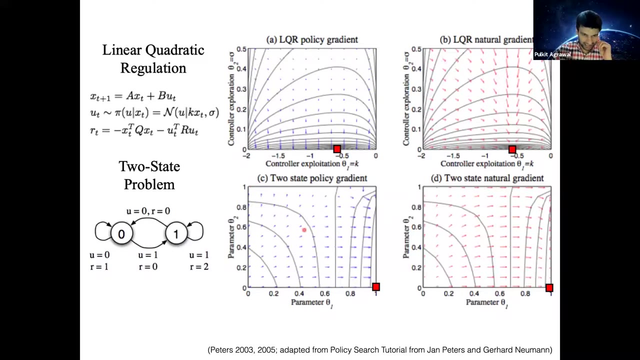 No matter where I start, I will end up converging to my optimal configuration much faster. So we can also take a second example. right, And you know, the curves show a similar behavior. right Over here on the top left, the gradients are very small, which would mean that the gradients are very small. 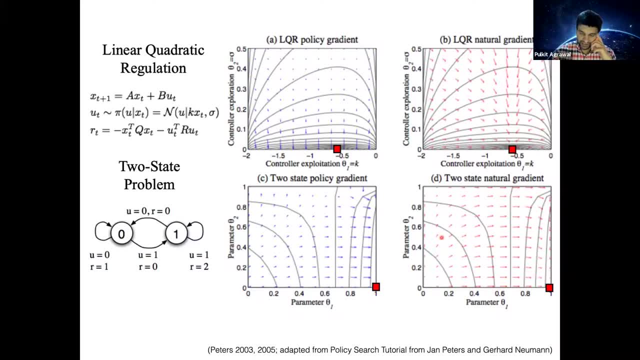 This would mean the convergence is going to be really slow. versus if I compute the natural gradient, the convergence is much faster. So what this suggests is that, instead of taking the gradient, if I do the natural gradient, it increases or it helps me converge much faster. 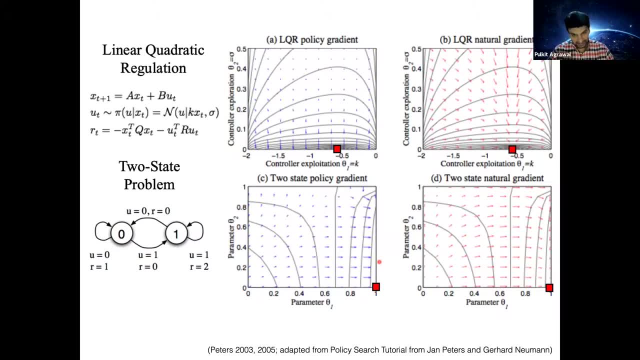 Any questions on natural gradients Or any questions? I have a question. Yeah, go on. Yeah, Hello, I thought that the natural gradient was used to make the theta update more invariant, but I thought it was another question about how fast it converges. 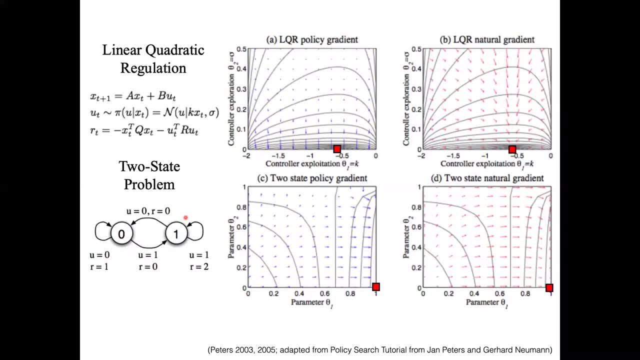 What I thought it was another question about how fast it converges. What? What do you mean? You mean like, theoretically, can you prove anything about the convergence? Is that what you're asking? My question is: first tell me if I'm wrong, but we introduced the natural gradients. 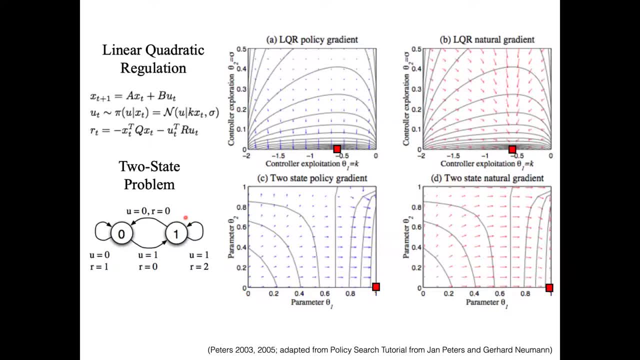 We introduced the constraint, the KL constraint, by saying that we want to make the policy invariant to change of parameters, So so, so so the okay. I think the way we introduced the constraint was to say that if my policy changes too fast, it can move away from the data and converge to a bad or a local minimum right or a local maximum. 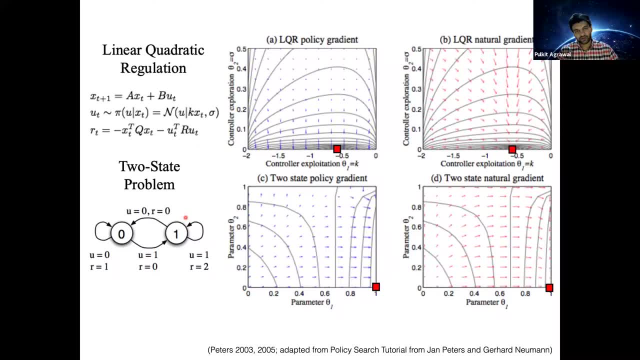 Okay, So, so what? what we want to do is to move slowly, right? So one way to move slowly is to constrain the parameters, theta themselves, right, Okay, And say I'm going to change theta by very, very small amounts, right? 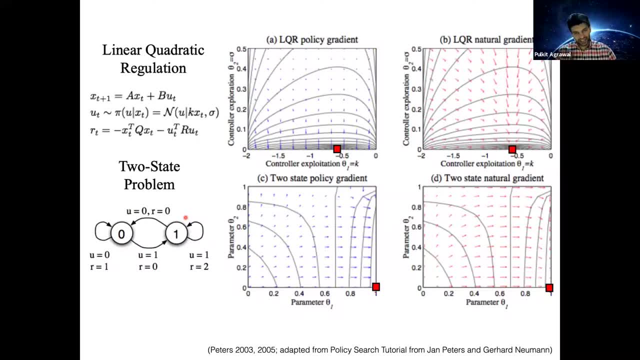 And that is how I'm going to move slowly, But that can lead to an issue, right? The issue is that for some dimensions in theta, you can move by very large amounts and they would cause very small changes in the policy. And some other dimensions of theta, if you move by very small amounts, they can cause a large change in the policy. 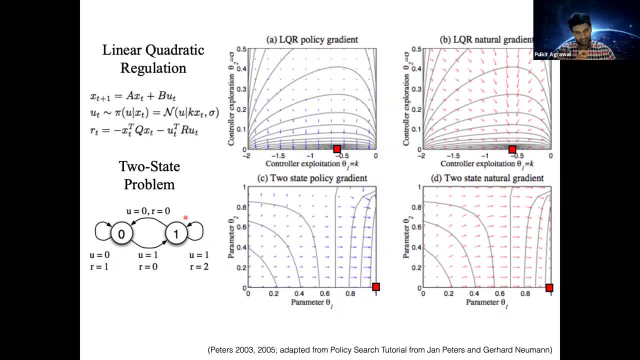 Right. So because the relationship between you know each dimension, like what is the scaling in each dimension of how so. so, for example, you know a distance of one in dimension one can change the policy by 10.. And a distance of one in dimension two might only change the policy by, you know 0.1.. 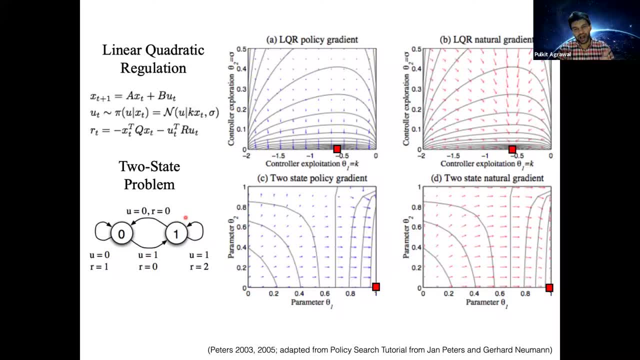 Right. So I don't know in each direction by what amount I should be moving. Okay, So this is because I don't know this relationship. So now, instead of putting constraints on theta, I can say: well, I'm going to put the constraint on the policy itself. 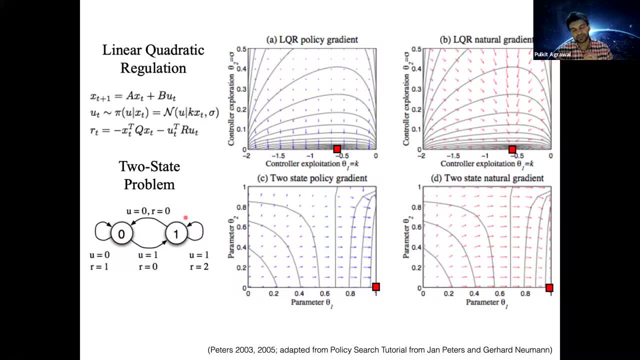 So the policy should not change too fast, Right? And if I put that constraint, then naturally what we come to is the KL divergence, Right? So I can say: instead of constraining how quickly parameters theta are changing, let me constrain how quickly the KL divergence is changing. 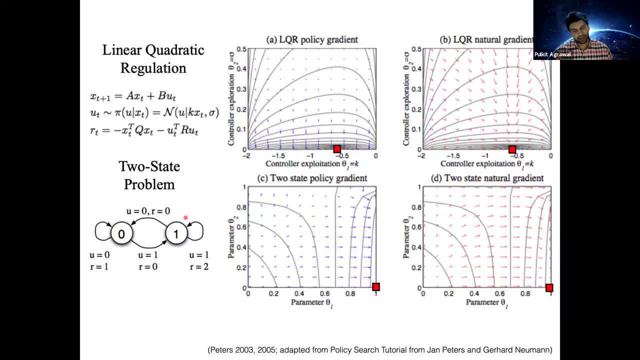 Right And natural gradients are an approximation to the KL divergence. It turns out that they also have another interpretation, which is that we become scale invariant. What that means is- you know what I said- that if I change my parameter like parameter in one dimension, my policy will change by 10.. 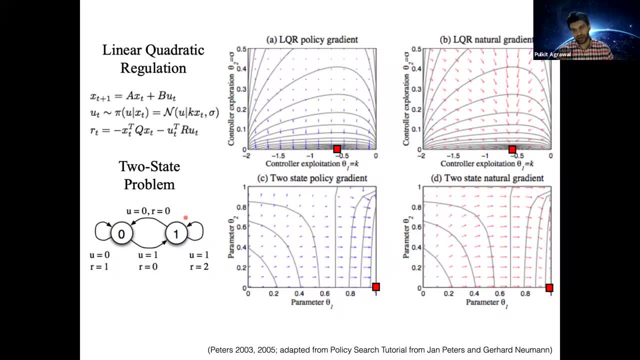 And if I change the parameter in another dimension, my policy will change by 0.1.. Now that will go away, Right, If I change my pattern, if I now compute the natural gradient and if I, you know, step by a particular amount in the natural gradient direction, then my changes are going to be similar. 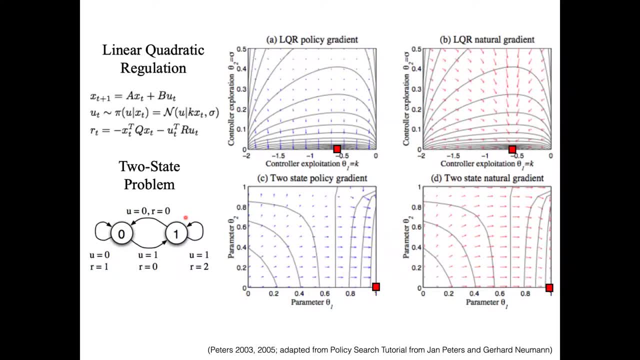 Does that answer your question, Jules? Yeah, Thank you, It was very clear. Thank you, Okay, Any any more questions? Nope, Okay, So, okay. So let's see you know what you know. so we made an approximation to the KL divergence. 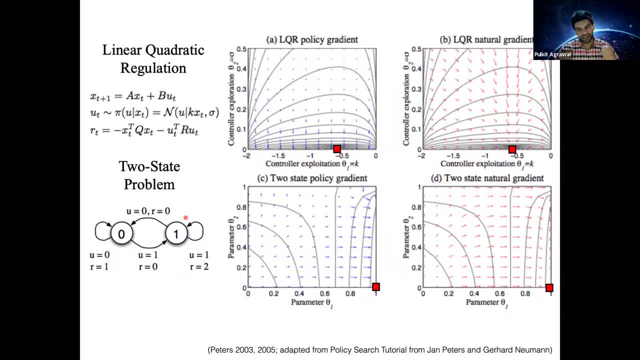 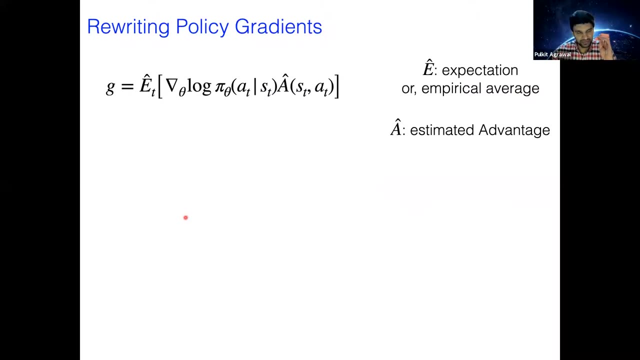 Right. So now, next, what we're going to see is: well, if you do not approximate the KL divergence the way we did- But we're going to look at some, at some you know other ways of optimizing the KL divergence. So before we do that, I'm going to 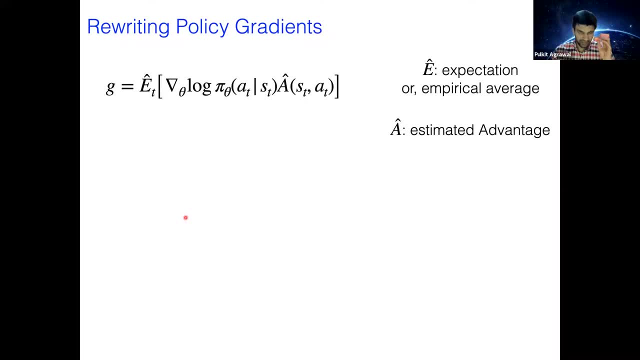 rewrite policy gradients, and the reason for doing this is to be consistent with the formulation that you will see if you read. you know papers like TRP or PPO and they just use a slightly different convention of writing. so I'm just going to rewrite policy gradients in that form. first, 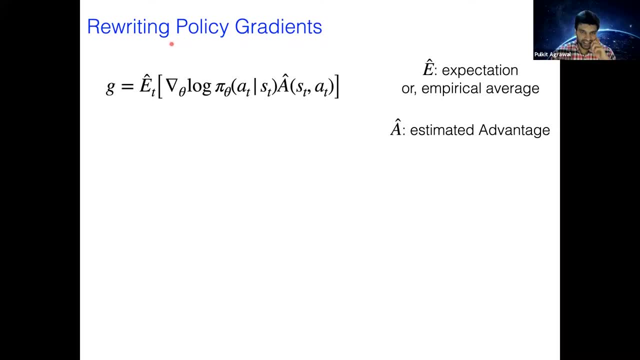 So you know, this is what we had as the policy gradient, where epsilon hat is my empirical expectation and A hat is the estimated advantage. So now you know, I can always take this gradient outside. the reason I'm doing this is just to, you know, drive home the point that 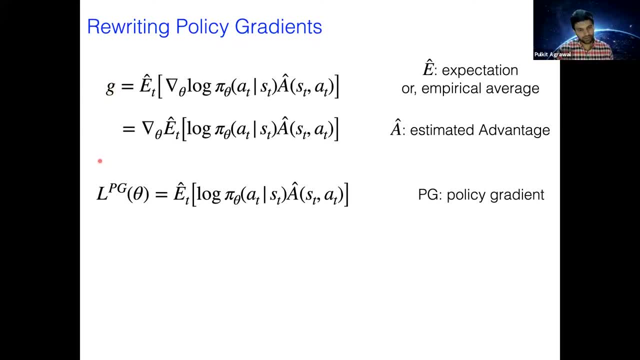 this parameter, or this gradient G, is actually optimizing the following loss function. right, Because if I take the gradient of this, this is equivalent, And so I'm going to call this LPG, which LPG stands for policy gradient. So now let's look at this term. 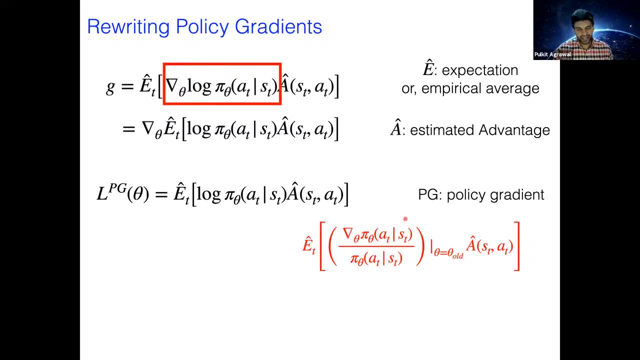 And because of the property of the log, I can rewrite this term in the following way: right, I'm just taking the gradient with respect to log right And this gradient is evaluated at my current set of parameters, which is theta old right. 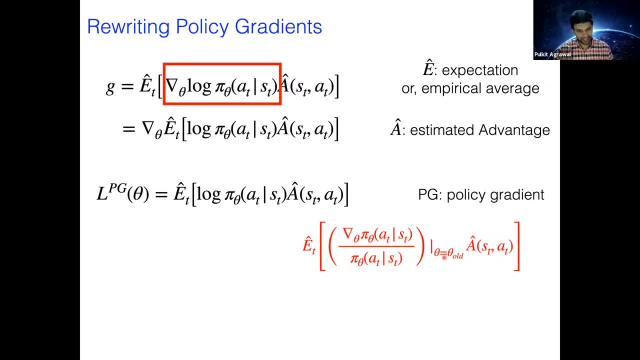 And theta are the parameters that I want to find. you know after the update. So now you know, because these two terms are equivalent. what this means is: I can rewrite this loss function in the following form: right, This log term is replaced by: 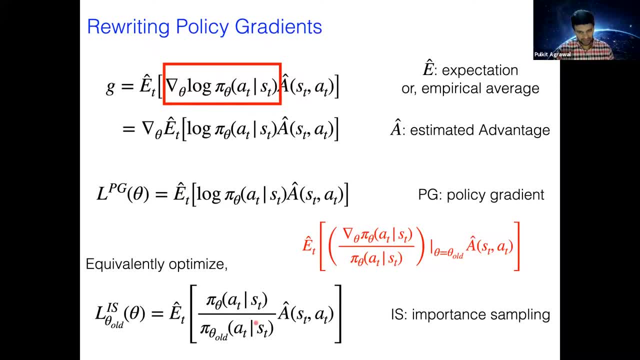 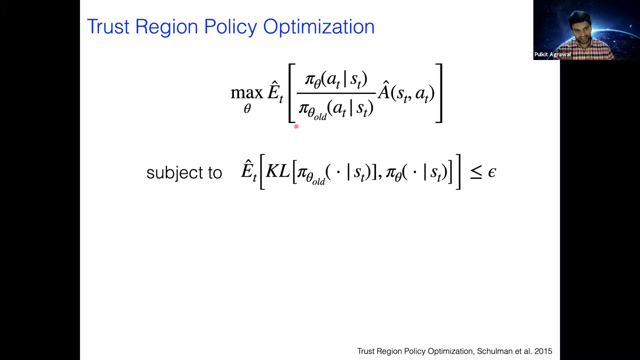 This ratio right. So this is. you know what you can think of as the importance sampling loss function. It is just rewriting my policy gradients in a different form. So now, right. So now what we can say is: well, I want to optimize my policy gradient term with the 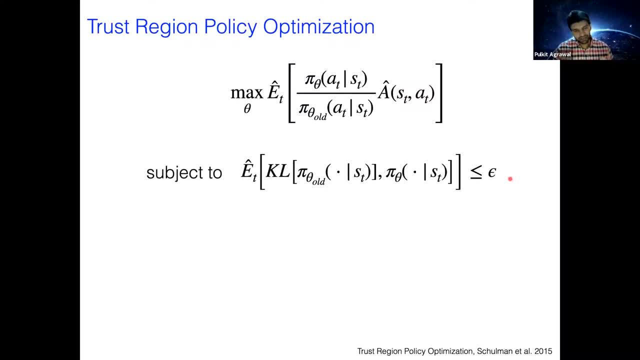 KL divergence. I want to optimize my policy gradient term with the KL divergence constraint. So in the previous slides with natural policy gradients what we saw was we had a step size that we chose and then we stepped by that step size in the natural gradients direction. 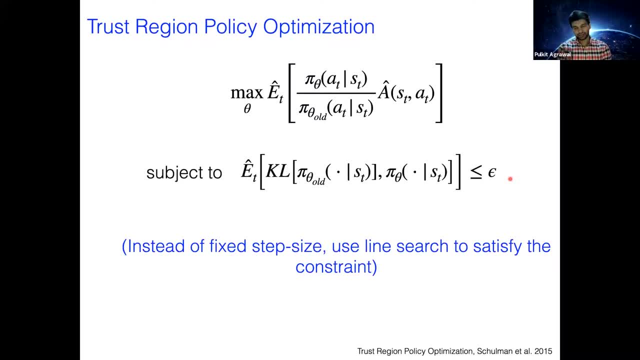 But now, instead of using a fixed step size, what we're going to do is to use line search to satisfy the constraint, right? I mean, what is line search? You know, I get my gradient And I shoot at different amounts in the direction of gradient and see for which one of those 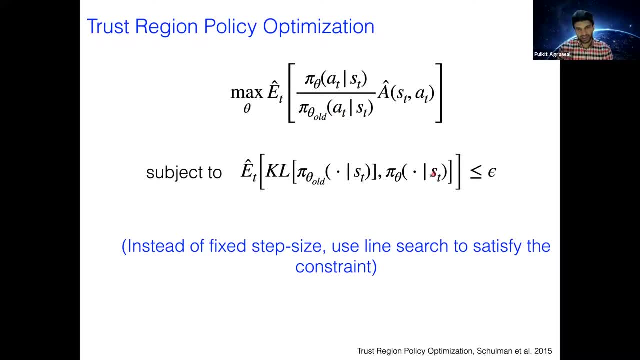 amounts is this particular constraint satisfied, And this is what you know- TRP or trust region policy optimization ends up doing So. the critical difference from natural policy gradients is that, instead of using a fixed step size, use line search to satisfy. So the critical difference from natural policy gradients is that, instead of using a fixed 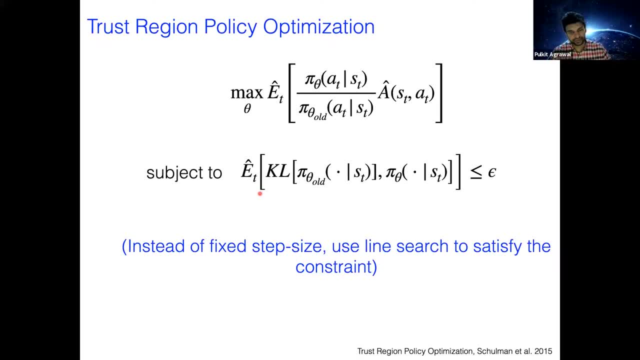 step size, use line search to satisfy That constraint. So now you know we can go and look into some. you know other ways of putting this constraint. Let's- let's just investigate this concept a little bit more. So, instead of putting the constraint in the following way, I could also rewrite my objective. 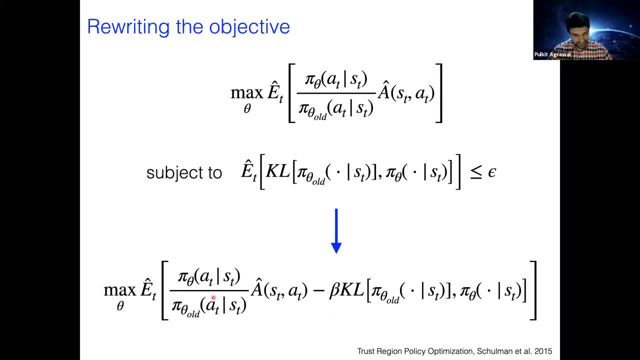 function and directly try to optimize. Okay, my like a joint loss function which is the policy gradient term plus the constraint term. so now, what are the pros and cons of v1? like the version on the top and the version on the bottom. so, version on the top, doing sgd is quite non-trivial. and why is it? because i have to. 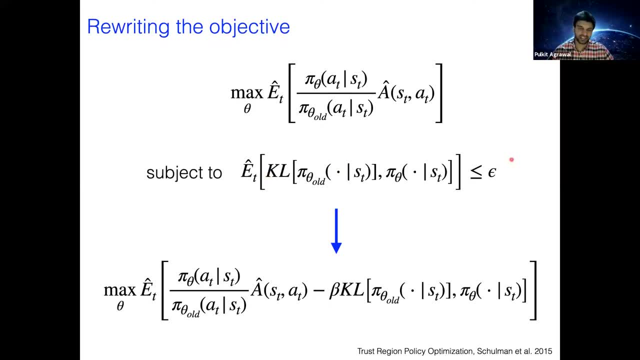 impose this constraint and if i'm doing a line search, that means that you know i for every example in my batch, you know i'll have to do, i'll have to, you know, search um till the time i'm satisfying the constraint right versus, if i just add the care divergence. 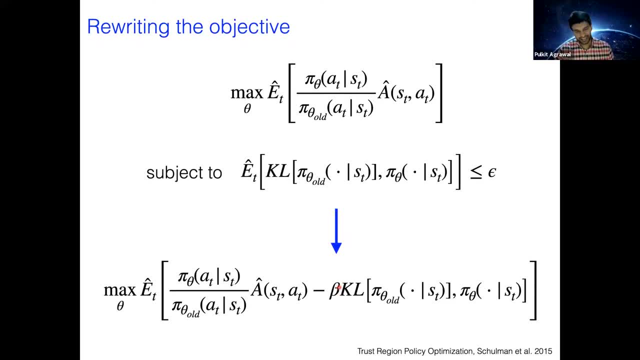 turn in my objective function. i can just use sgd, you as is so, but then you know what i'm going to lose is the guarantee that my care divergence is actually less than epsilon, which is guaranteed if i am willing to do an explicit line search, which is going to be computationally be more expensive. 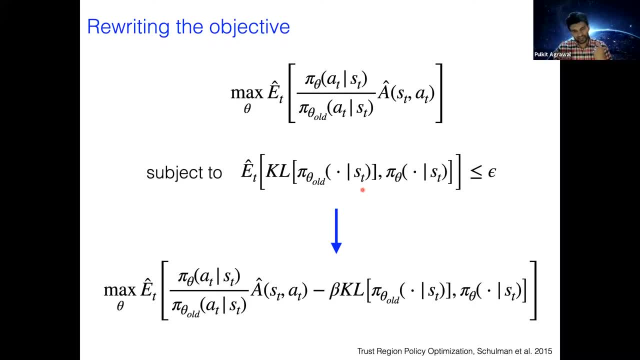 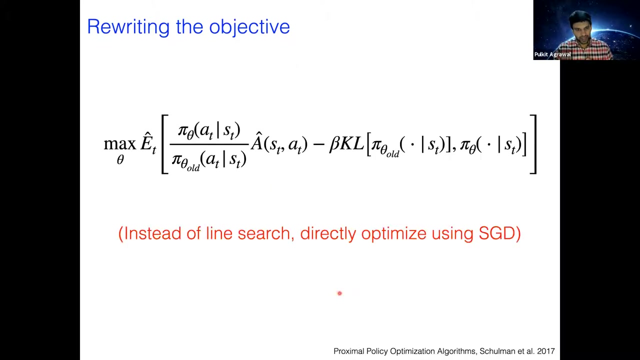 so, because of you know this one reason we're going to to increase my computational efficiency, i'm going to try to go to a different formulation where i put the care divergence term directly in my objective function. so this evaluation was, you know, performed in one of the papers and what we'll do is, instead of 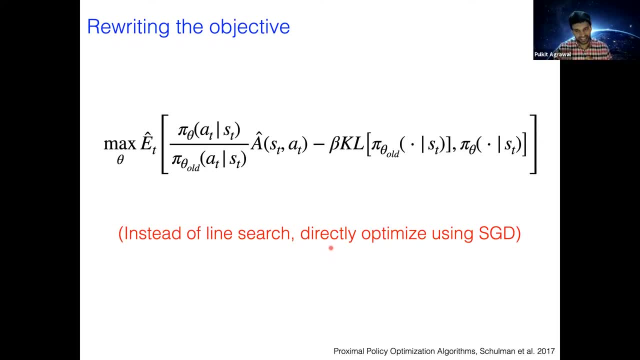 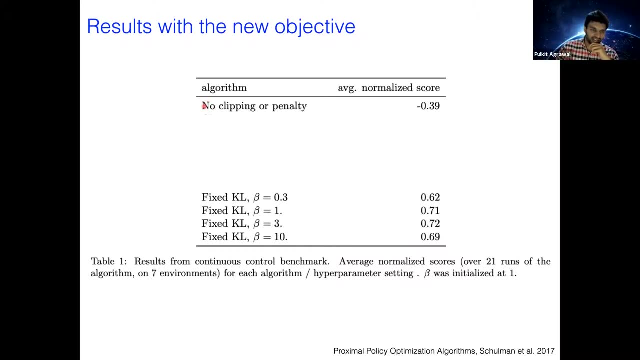 doing line search. we're going to directly optimize using sgd and the results look as following. so this, the first line over here is showing you know, no clipping or penalty, and the rows over here are showing if i use a fixed arterial divergence loss. so these results are on seven environments. 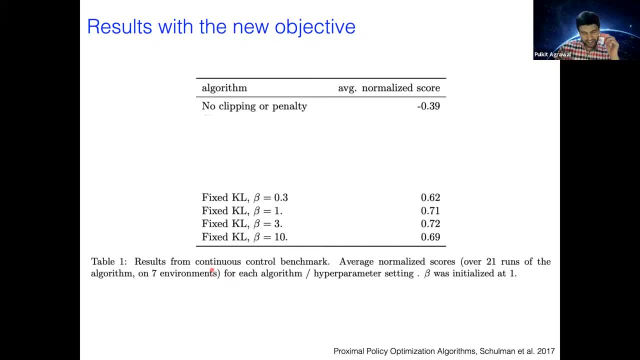 and from the continuous control benchmark right, which is a bunch of environments which have the Acrobat, the cat polea, cheetah Walker and so on and so forth. So this is some of what we covered in lecture four. We covered, you know, some of these benchmarks. 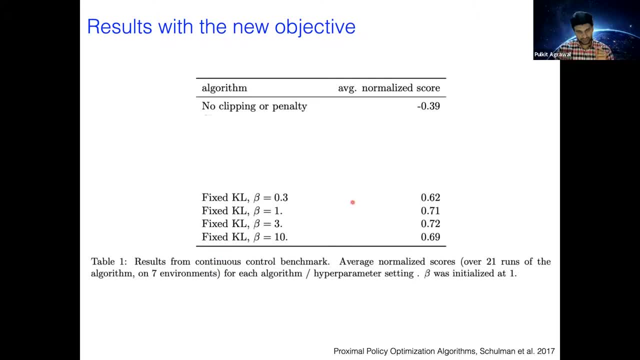 So what we see is that, you know, having the KL divergence constraint is much better than having no such constraint, right, Because my rewards are much higher. Then, instead of having a fixed KL, you know, one can also adapt the KL as the training is happening. 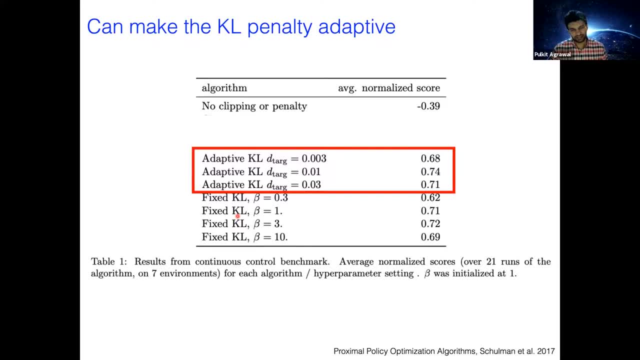 And sometimes you see some benefit right, But the benefit is not really that significant as opposed to having a fixed KL divergence right. It helps, you know, sometimes a little bit. Now the PPO paper you know talks about you know, 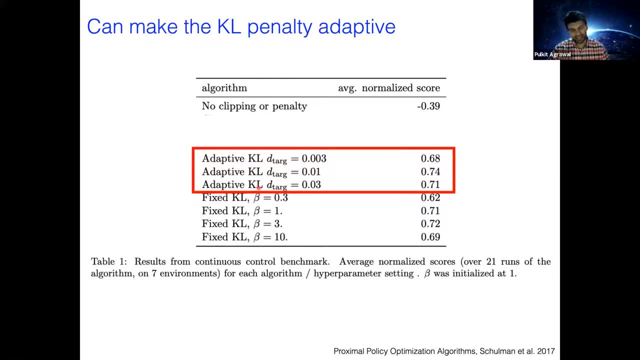 both in the fixed scale and the adaptive scale and they have a discussion in the paper. because practically speaking it is adaptive scale does not help, I'm going to skip. you know how they adapt it And if you're interested you can read the PPO paper. 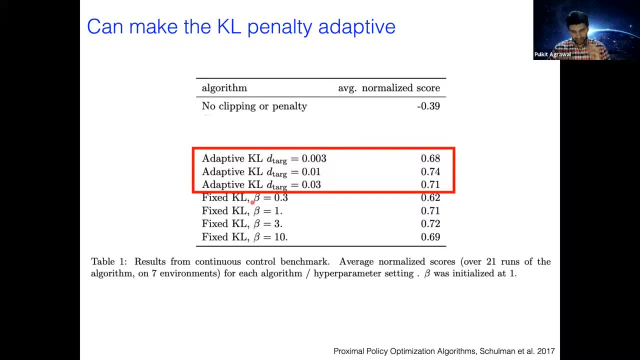 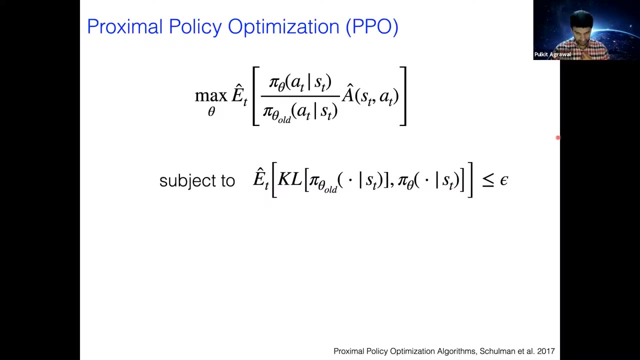 But so what they found was that, well, fixed scale and adaptive scale are two ways, but actually what works even better is to do clipping. Now, what do I mean by by clipping? So remember what I had is. this was the objective. 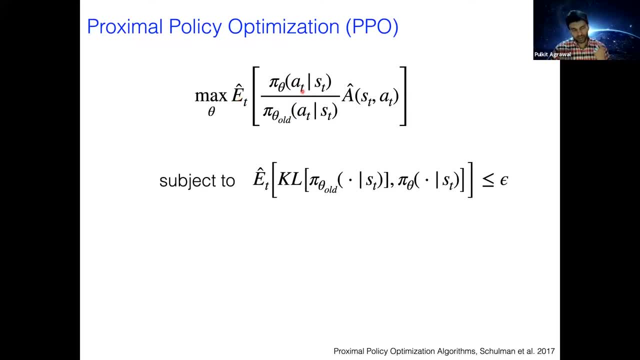 I was trying to optimize. Now again, to be consistent with the notation in the paper, right, I'm going to rewrite this term, which is the ratio of the actions with my current policy and my old policy, as this term RT right. 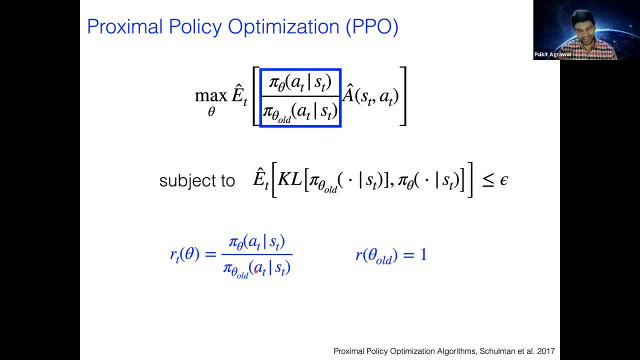 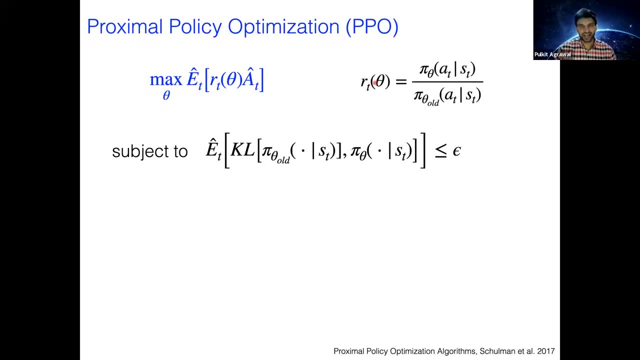 And R theta of old is equal to one, which is expected. All right, So now we're just modification or this rewriting. you know my objective function looks as following: So I have my ratio term and I have my advantage function. So now, instead of using this K divergence constraint- 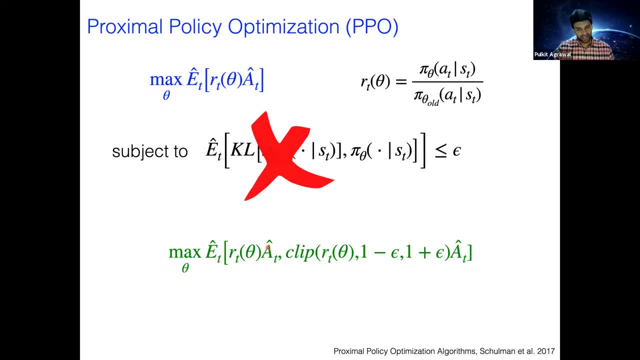 what we're going to do is we're going to clip my, the product of. you know, this ratio and the advantage function right. So if you look at this expectation, it says: take the expectation of this term, RT 80,. 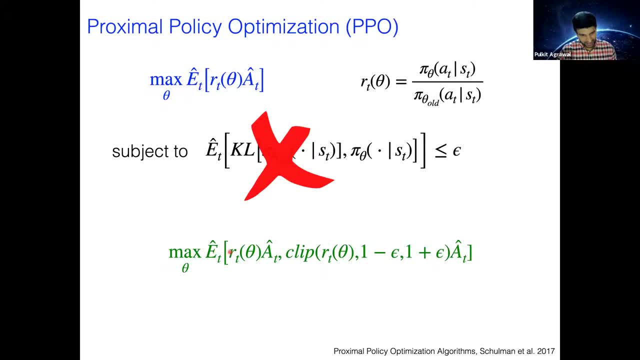 or say there should be a min term over here, which is missing. So it's min over this and the clipped version right. So what this means is that when I'm clipping that, it means that don't let the ratio of mine. 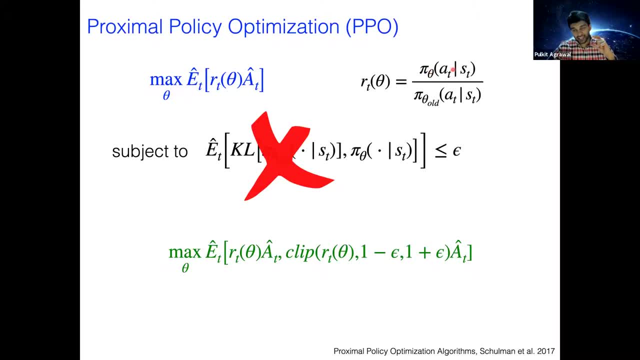 of the policy or the probability of the action from the new policy and from the old policy change too much, right? Because if this is going to change too much, then I'm going to clip it right. So this clipping enforces that, my policy, that I'm finding. 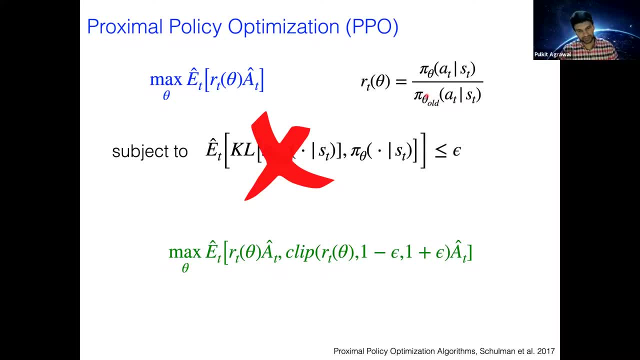 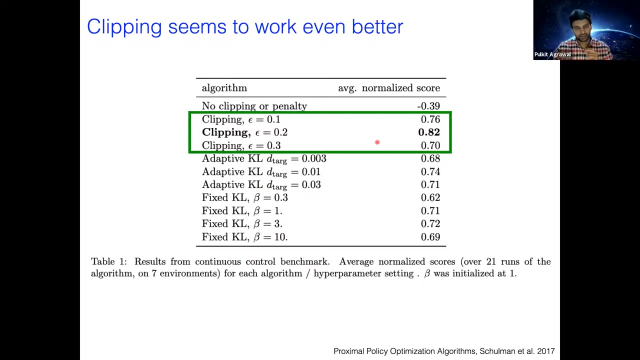 is close to my old policy. So instead of doing the case the divergence term to constrain how my policy is changing, we can use this clipping function to modify how my policy is changed And empirically, as we saw before, what they found is this clipping is working much nicer. 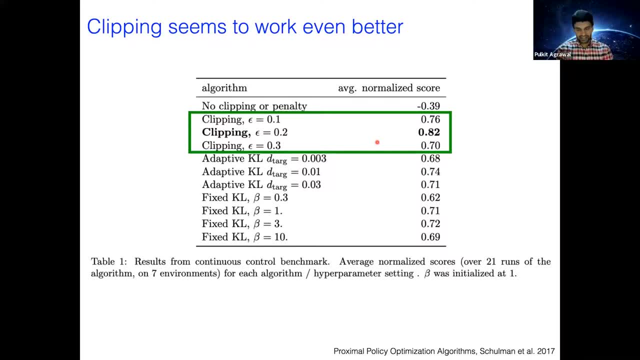 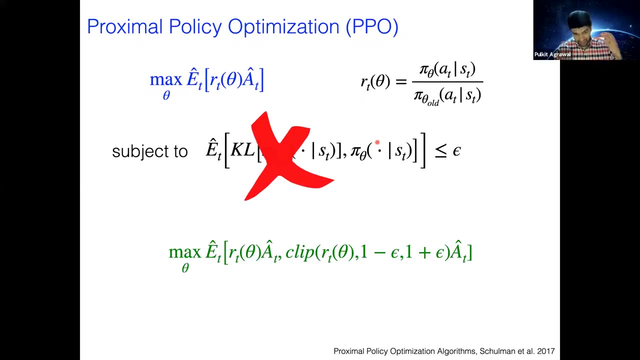 than using the care divergence term explicitly. And then this is what gave the algorithm you know, proximal policy optimization right. So everything else you know remains pretty much the same. So you can think of. you know, we wrote down the objective function for H3C. 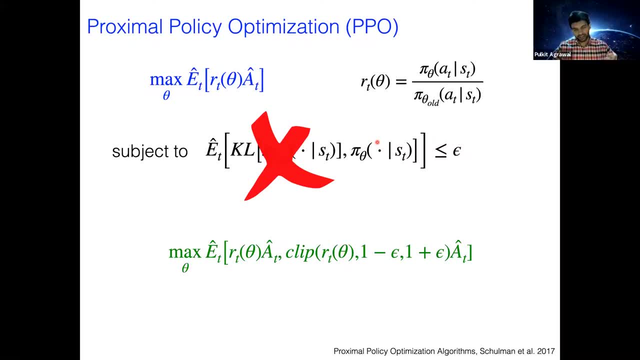 which had the policy gradient term plus the entropy. So the entropy term still says. the only thing which changes is we replace the policy gradient with this clipped term, right, Then the other details are: you know exactly as is, And you know, then you know. 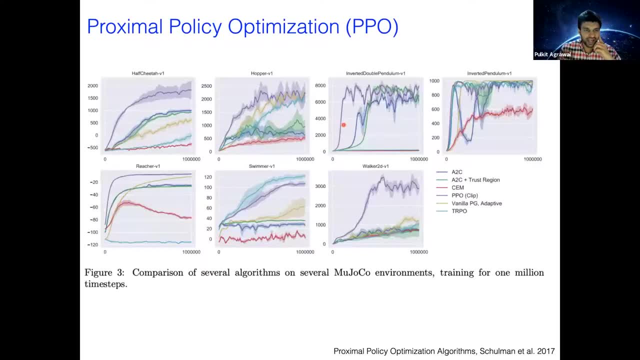 they found this clipping penalty to work better and you know they had results in which they were comparing across these different environments. So, as you see, you know what they consider is, you know, vanilla policy gradients, which is in yellow. 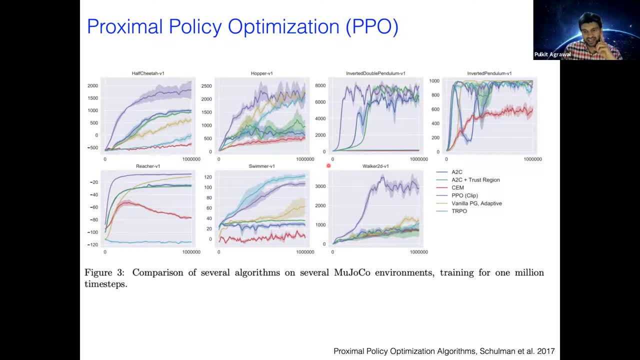 then they have A to C, which is shown in blue, then they have TRPO and finally PPO, which is in purple, And what you see is, you know, across these benchmarks, at least in most of them, PPO is outperforming TRPO. 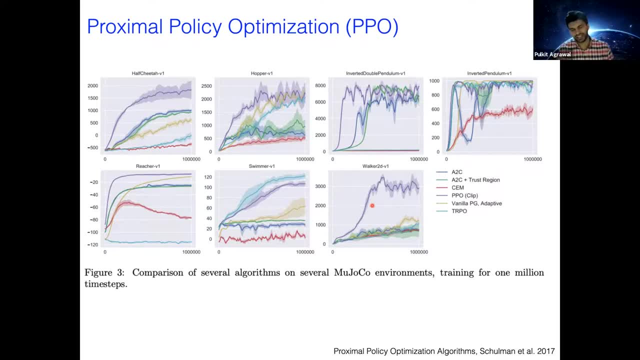 So you know, practically the advantage that PPO gives is that in TRPO you have to do this line search which becomes slow, versus in PPO you can't. you don't have to do line search, You can directly optimize the objective function. 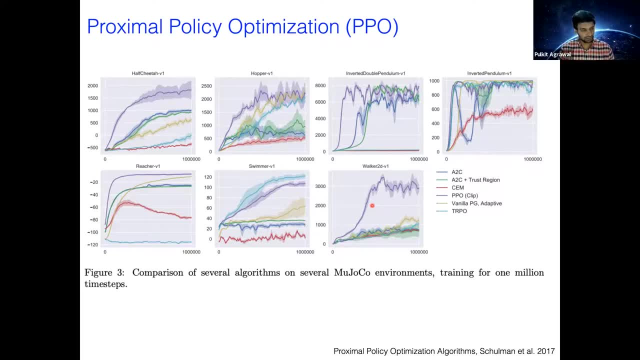 using SGB and that makes it, you know, much more practical to use right And the PPO paper, you know, claimed that, you know, PPO outperforms TRPO. Now that comes with a grain of salt that we are going to. 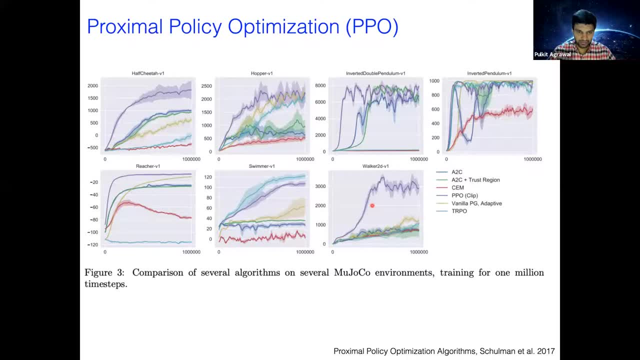 look you know in a few minutes, but before you know we look into that. I will pause and see if there are any questions That people might have. I see one in the chat. So TRPO uses care divergence and PPO uses clipping. 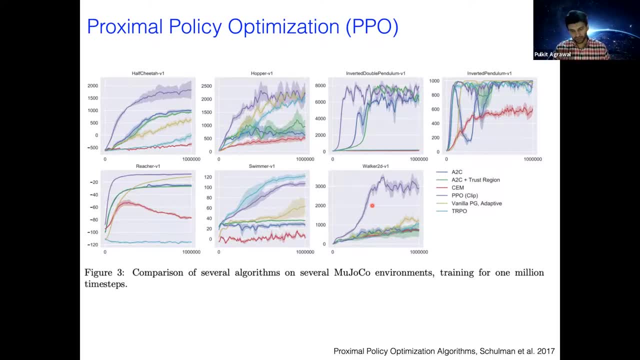 That is true. So I think the the buildup is as following: right, We have our vanilla policy gradients. When we say, well, to choose alpha, we need to be clever. So we will introduce a constraint, which is the care divergence constraint. 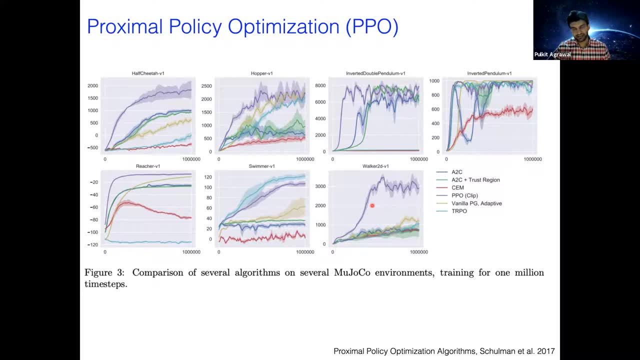 And one way to approximate the care divergence leads to natural policy gradients. but natural policy gradients was using a fixed step size. Then the intuition was: well, the step size doesn't needs to be fixed. Maybe I should make the step size be adaptive. 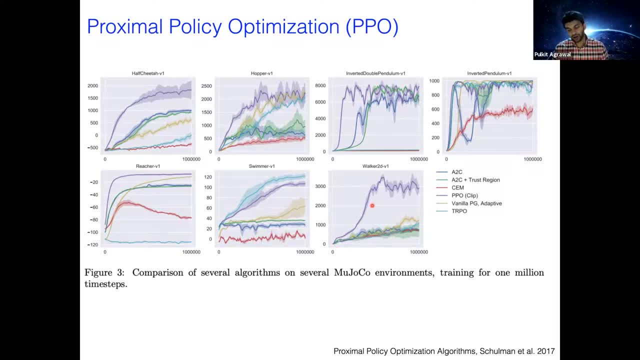 which is what led to TRPO, was because of adaptive step size. The problem is that it becomes slow and cumbersome to implement, so that you know it doesn't need to be a fixed step size, And so that led to TPO and TPO. 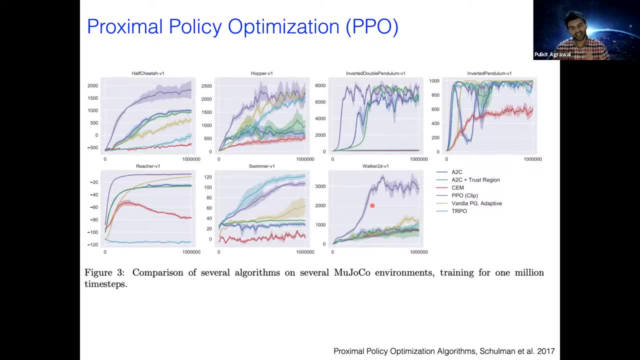 when they were doing their empirical evaluation, what they found is a clipping to work better than care divergence, right? And therefore they said: well, let's use clipping, which has the same effect as the care divergence, And this was what was presented in a 2017 paper. 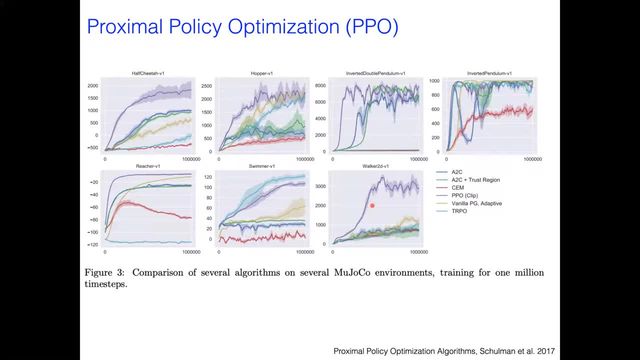 All right, Thank you. I have also a question. Could you explain again: how do they come up with the idea to using the clip? If I understand well, it was just at the beginning to avoid the line search, to be more practical. 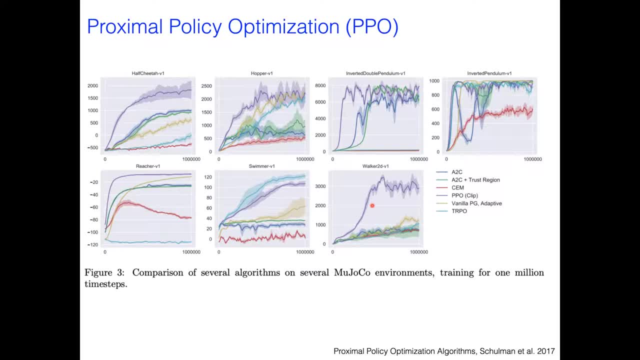 and then they realized it was also more efficient, or So they realized that it is leading to better performance. But it is by chance, or So it's an empirical evaluation that they did So, if you actually go and read the paper right. 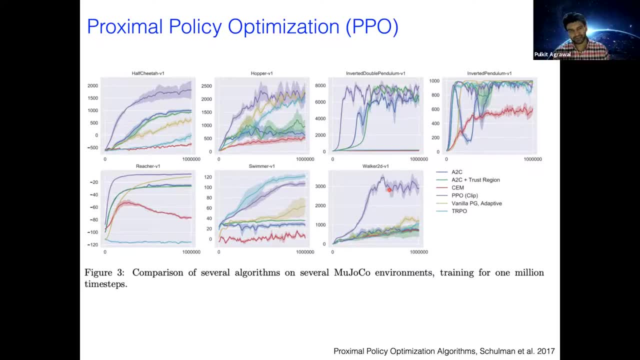 what you will see is they say in the paper that you know TRPO uses, you know, one objective function, which is to minimize the care divergence. We are going to investigate different ways of constraining how quickly the policy can change. 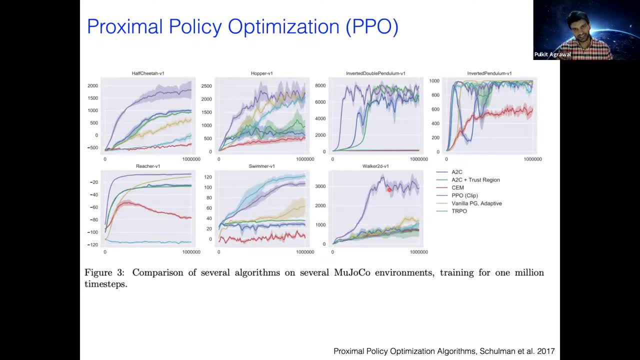 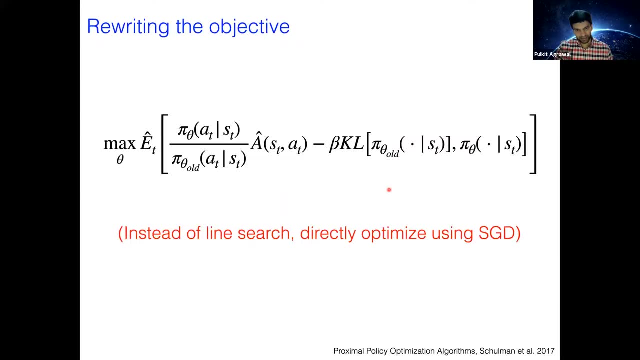 Right, So they did. so what they did was they, you know, instead of doing line search, they directly tried optimizing the kl. you know, they directly tried optimizing this objective function. they evaluated this one. then they said, well, you know, maybe the kl divergence, that the term beta should not be a constant, but it should be changing. 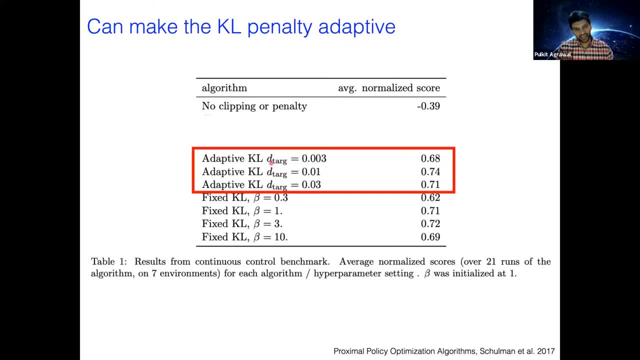 so that is what led to the adaptive scale and they also tried clipping right and you know, so they pretty much they said i'm going to try three things: clipping, adaptive scale and fixed scale- and the paper is pretty much just evaluating these three things. okay, because i i see the 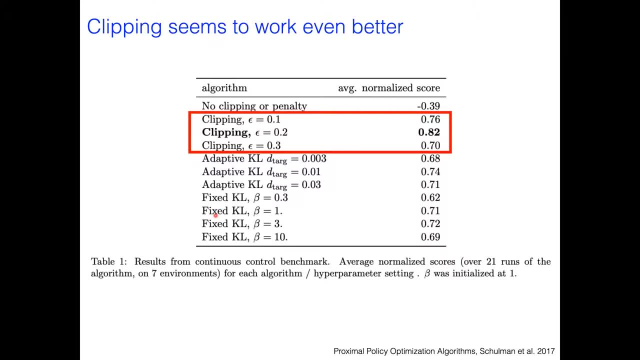 link between, uh, switching from the fixed scale to adaptive scale, but switching from adaptive scale to clipping. i don't really see the link between. so, so there is. so there's one one which is at a high level, which is that care divergence is essentially trying to enforce. the policy should change slowly, right, and you can think of clipping as another way. 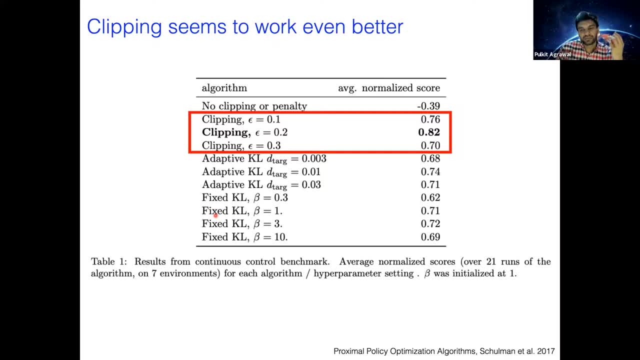 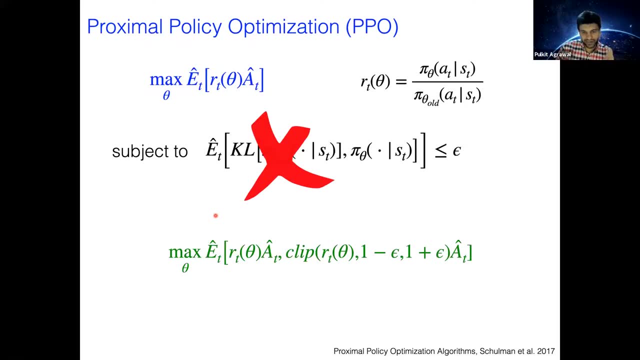 of ensuring the policy is changing slowly. okay, right, so i think that is the you know, like the high level link. now is there a one-to-one derivation? no, you know, there is not a one-to-one derivation. okay, thank you. right, and you know now, i mean, we'll just see you know in just a few minutes that. 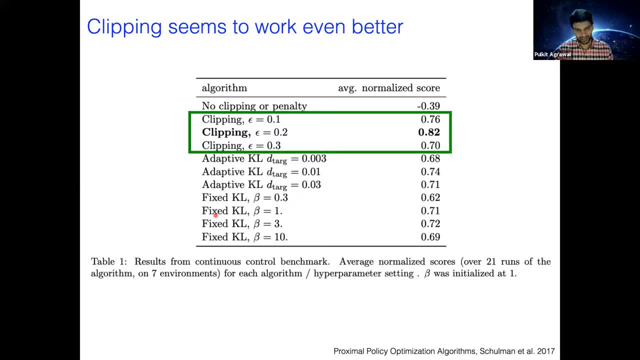 you know it actually turns out it's unclear if clipping actually biases anything more than care divergence. so but you know we will come to it in a bit. but you know, before you know i move ahead. you know, i'm just. you know if there are any questions. 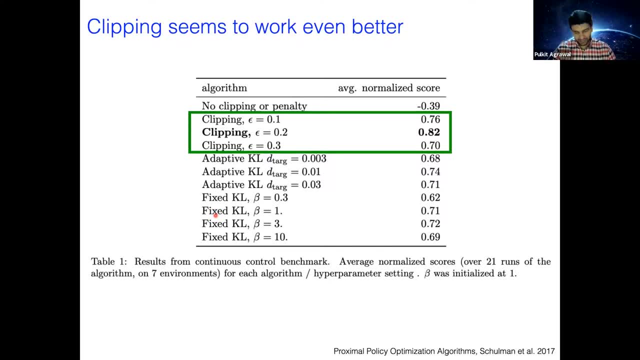 any doubts at a conceptual level of what happened from the start of the pandemic to the end of the pandemic, to the end of the pandemic. so i will be happy to answer them. so i will be happy to answer them from policy gradients to natural policy gradients to trpo, to ppo. i'm happy to answer them now. 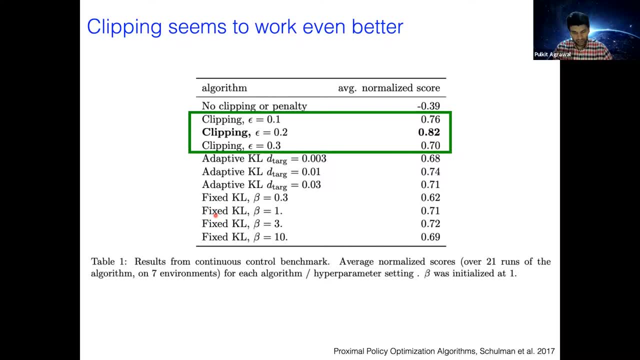 okay, well, it seems like there are no questions, so. so what i covered are these algorithms at a conceptual level, so that you get an essence of what is the main idea behind the structure of a pathway to организate these algorithms. you know a bit of this. we are going to do. 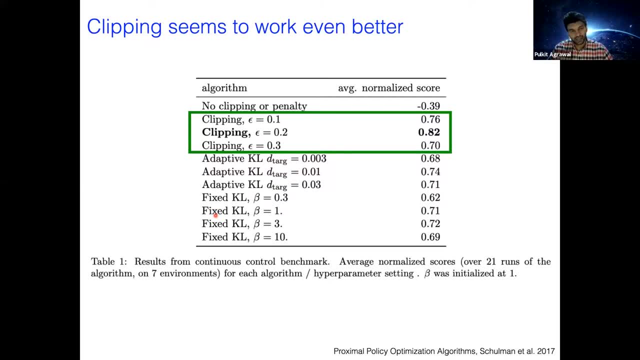 in. you know one of the assignments. now you know. if you want to get you know more in-depth knowledge about trpo and ppo, i encourage you to read the papers and i hope you know, with the background from this lecture, reading the paper will be much more easy and you know. 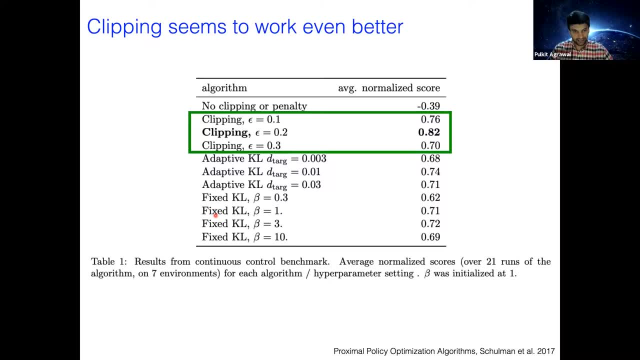 if you really think you know we have learned much today and if you really think i can give you some good advice, you know. so i will stop talking for now. i will see you in the next session. should go into more details about you know how the care divergence term or constraint is applied. 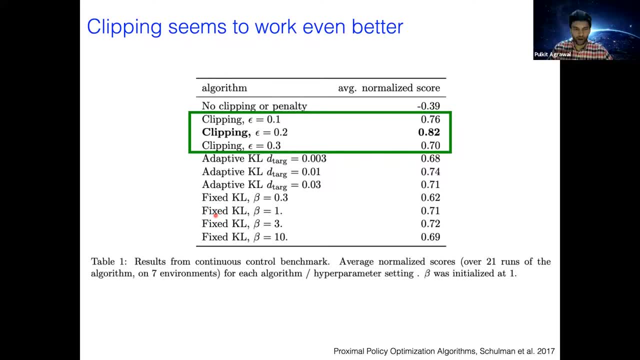 you know, feel free to provide. you know that in the feedback form and we you know, if there is significant interest, you know we'll be happy to cover it in more detail. but i think we have communicated the core conceptual idea in what goes behind national policy gradient, trpo and ppo. 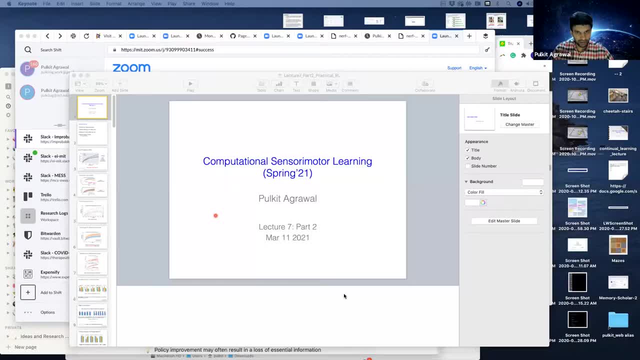 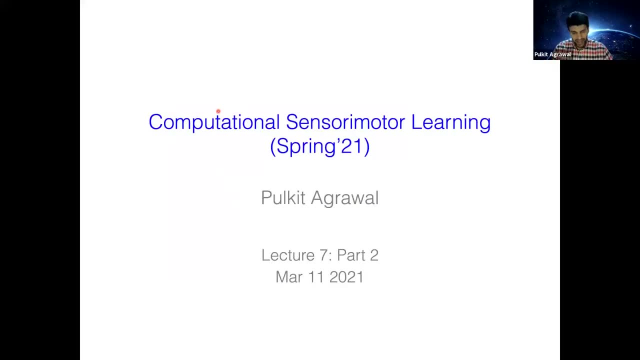 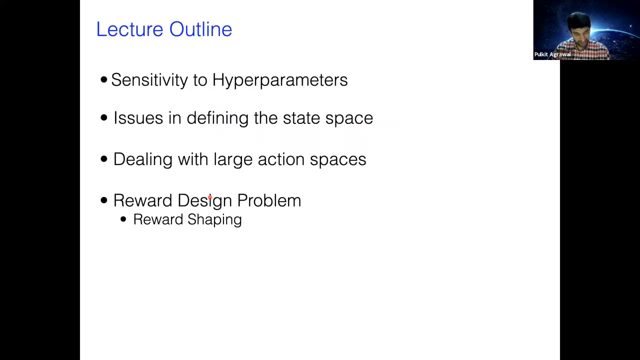 okay. so well, if there are no you know questions, i'm going to switch to part two and you know, in part two we are going to look at a couple of things. so the first thing we're going to look at is, you know how these, you know reinforcement. 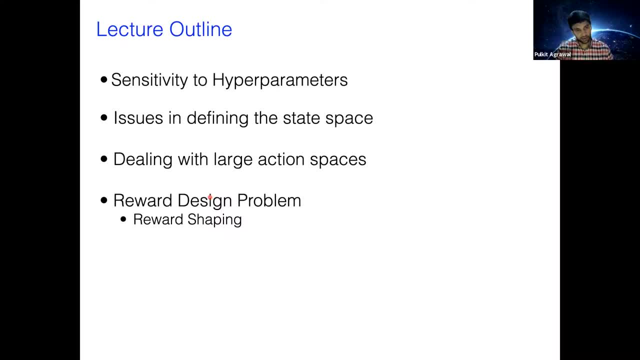 learning algorithms are really sensitive to hyper parameters and also the issue of variance and how it practically shows up. you know, then you know, if we have time, we are going to go into issues and define the state space, how to deal with large action spaces and touch upon the reward design problem. 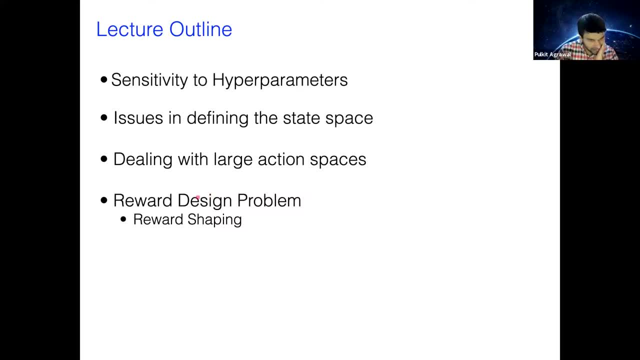 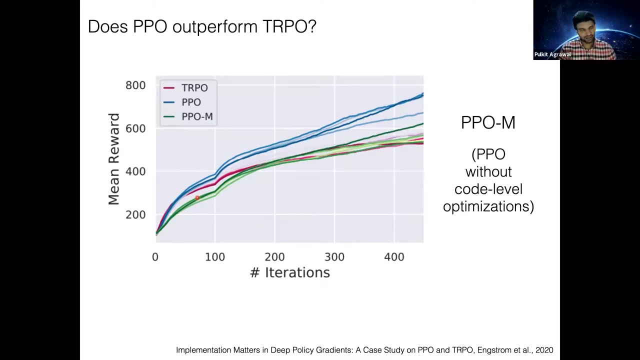 but maybe some of the you know the, maybe the last two bullet points you'll touch upon the next lecture. so let's, you know, start with sensitivity to hyper parameters. right, so you know the question, you know which we were ending the last, you know, the first part of this lecture was, you know, does clipping actually outperform? 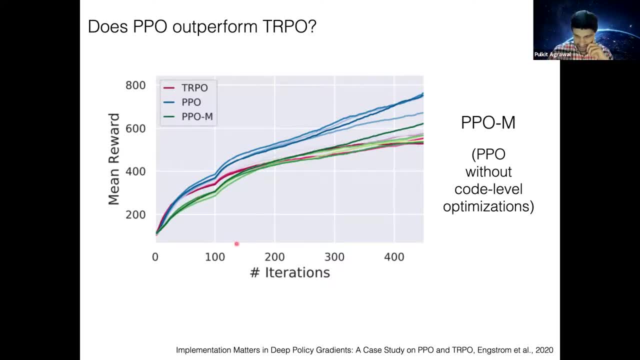 rather than a little bit, and so we have to look at the kind of ups and downs in the different ways that it takes to manage, you know, or to manage the data, and- and this is something that we should be at the center of- we should be able to solve the basic problems. 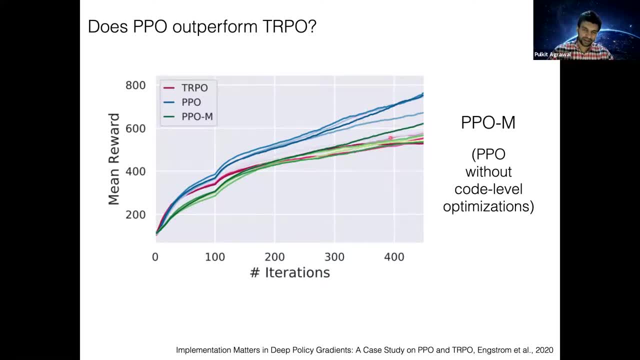 of distributed data analysis, because there's an opportunity to do it, and we've done that at the state level, and the state level will be more effective than the state level, and so our first concern is: how do we manage that? and that's a really good question, because really the question is: 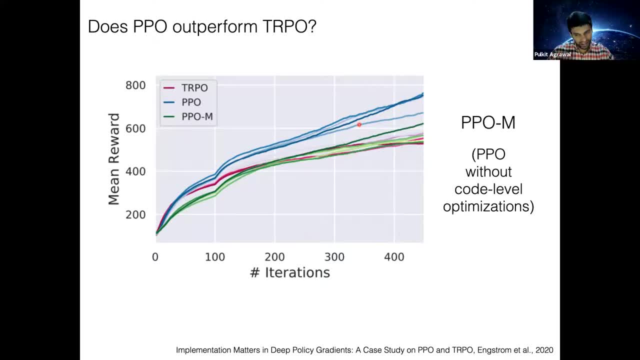 that the PPO paper also did more. So there were a bunch of code level optimizations. you know which were tricks like: how do you normalize the reward function? how do you normalize the observations? you know what choice of like learning or the 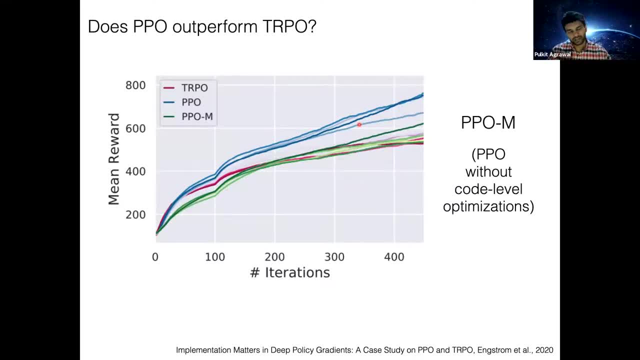 optimizer do you use? do you use Adam or do you use something else? So it turns out there were many, many such choices, Which were also different between the TRPO code base and the PPO code base. So what they did was they constructed PPOM, which is PPO, without these. 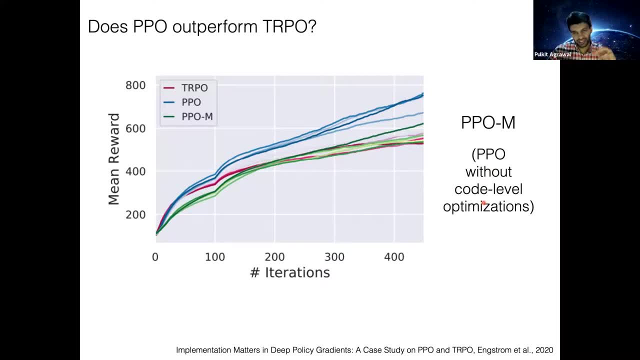 code level optimizations, right. So they removed all these extra things and then compared- uh, you know, TRPO against PPOM and what you see is that TRPO and PPOM are pretty much the same Right. So in some ways you know, maybe the advantage that PPO was having right. 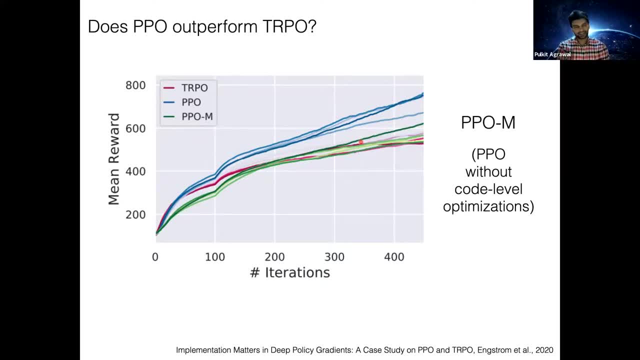 Seem to be coming from code level optimizations instead of it really coming from the clip versus the KL divergence term. So you know, as we talked about, you know this clipping was a heuristic that you know seemed to work well. but further investigate, and you know then what happened practically. 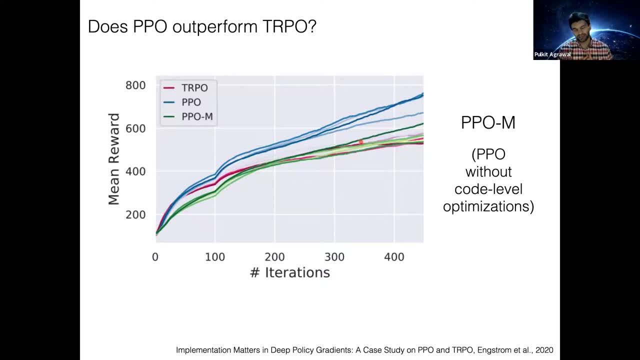 is you know people? would you know, take the PPO code and run it, but no one, I think, carefully analyzed in you know a couple of years that you know. was it really the clip objective which was changing things or some other things? 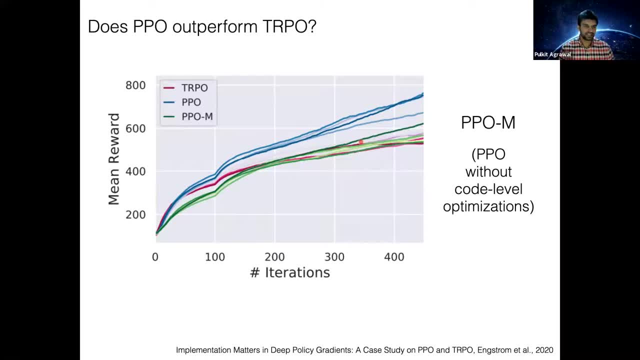 Yeah, Yeah, Yeah, Yeah, Like the way you normalize, which was affecting performance, right. Then this 2020 paper is, you know, really questioning if flipping is doing better than just putting a KL divergence constraint. So yeah, 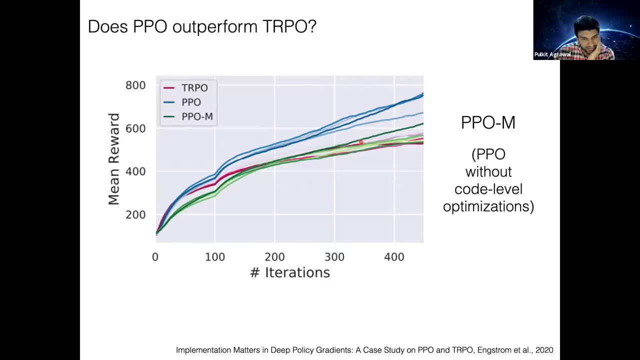 So I think the jury is still out there, right That you know. it seems like both of them- KL divergence and clipping- do pretty much you know similarly to each other and in some ways you know you'd be a bit disappointed. 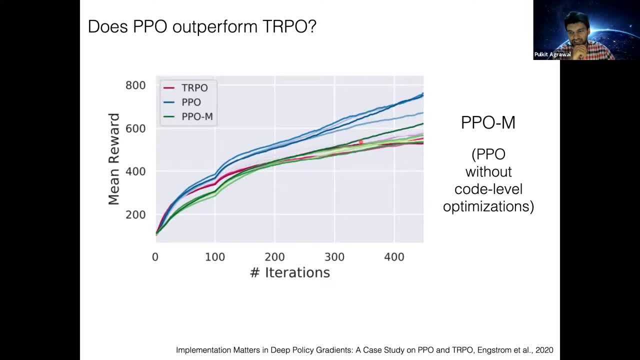 that you know why. why is it you know that these things are not found earlier, that you know these code level optimizations can make a difference? I think a part of it comes from the fact that the field is still evolving and you know. 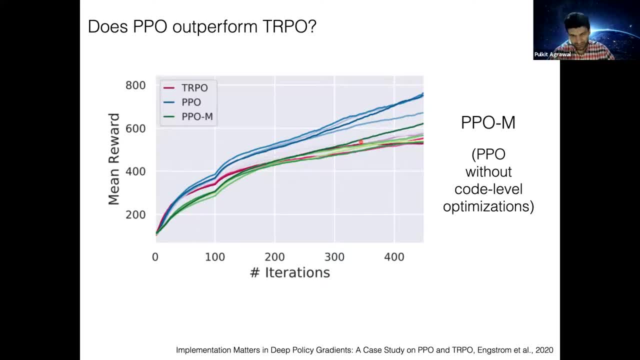 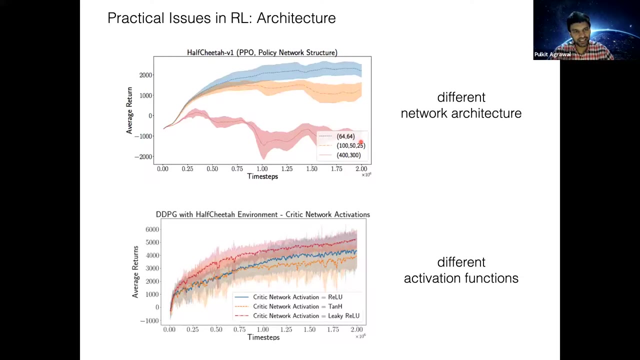 why these things are hard to catch is, you know, something we'll look at and you know, remaining So. just to you know, illustrate that you know let's now look at. you know some practical issues which end up happening when we're evaluating. you know, reinforcement learning. 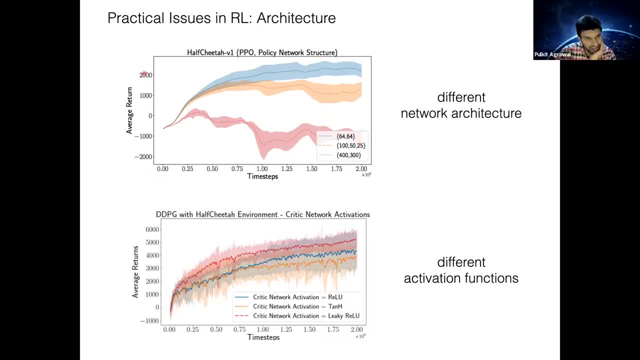 algorithms. So what I'm showing you in the first plot is this one environment, which is the half cheetah, And what we're using is three different network architectures, right, So one is 64 plus 64. Which is two layers of 64 units each, a slightly bigger network and even a bigger network. 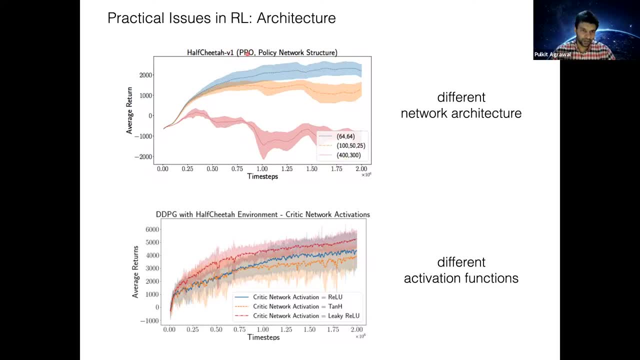 So- and this is trained all with PPO- And what you find is there is a huge performance gap between different choices of the network. So if you were doing supervised learning, you know performance obviously changes when you value the network architecture, But you wouldn't expect such a. 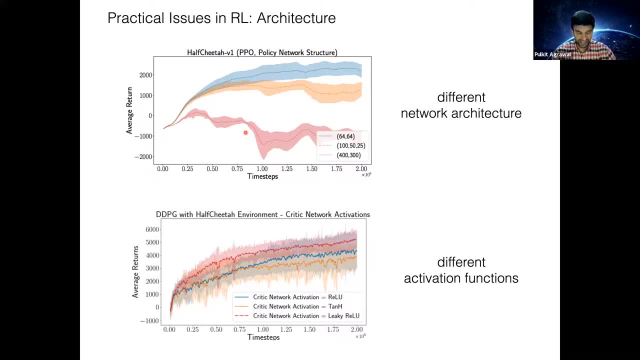 Big difference are, given that the differences in networks are not significant. So what this shows is that even the current state of the art algorithms are quite sensitive to the choice of network architectures. So these results are a couple of years old. these are the 2000, you know, 18,, 19, you. 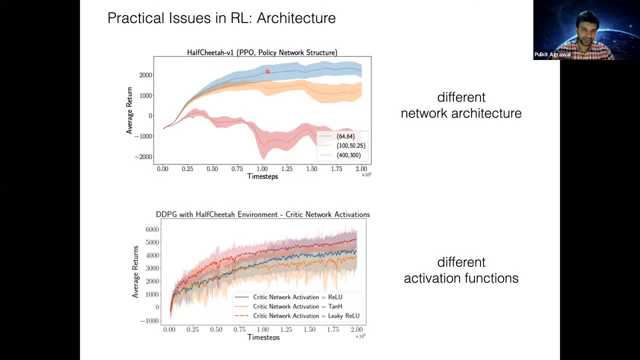 know that timeframe, you know since then, you know we have made Some progress to. you know, remove some of these issues. but you know, if you were to implement PPO, as we have discussed in the lecture until now, this is what you're going. 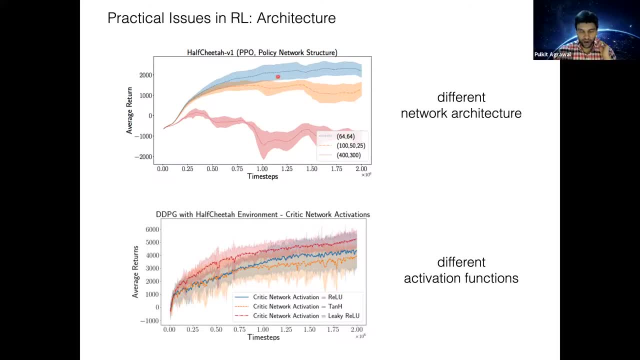 to get Right. I mean small changes in architecture can have a huge performance difference. Similarly- you know this is showing in DDPG. What I'm Talking about is the activation function. So once we modify the activation functions, they also cause a change in performance. 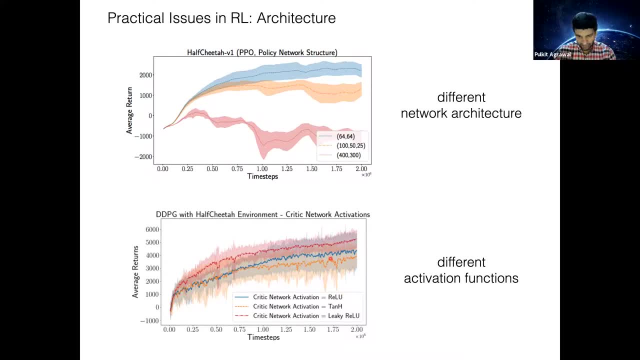 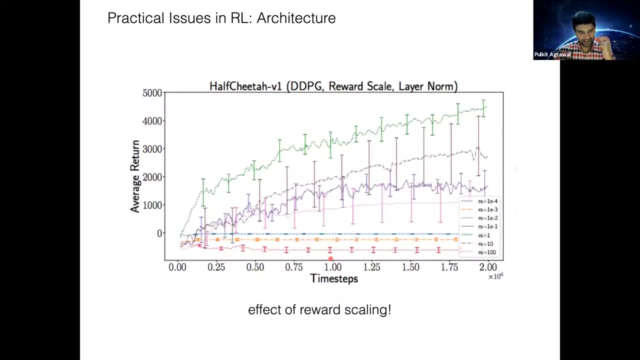 Right. So I don't seem to have a reference in the slides over here, but I'll repost the site with the reference So you can also refer back to the paper which was doing this analysis. Then, similarly, you know, there's another thing that we can modify, which is the reward. 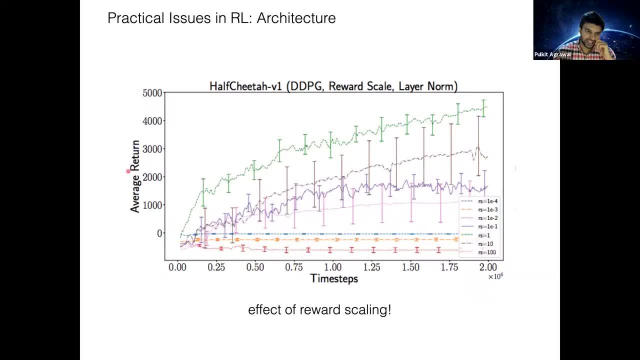 scaling. So each line over here is showing the performance with a different reward scale. Now, what do I mean by reward scale? It means that I'm going to multiply my reward by some value. So I could multiply it by one E minus four. 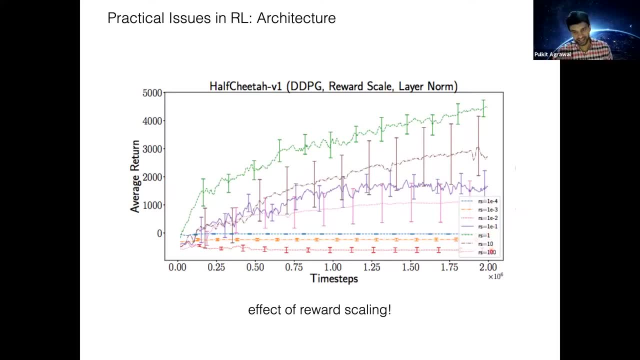 I can multiply by one, I could multiply by 10, or I can multiply by a hundred. So it turns out, you know, for this particular environment, you know, if you modify it you'll see that if you modify the scale of the reward functions, the performance can change quite. 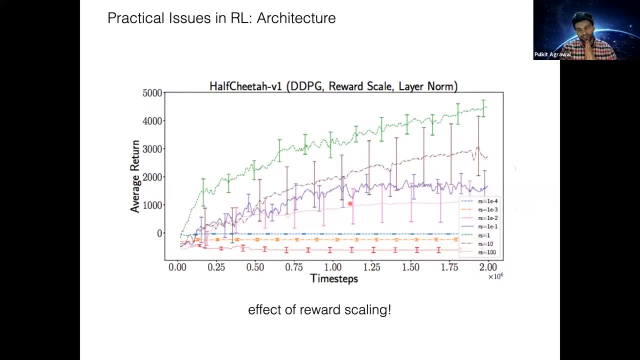 a lot. Now why would that happen? intuitively, Right, The reason is that if you change the reward function, you're pretty much changing how big the gradient is right. So if the gradient magnitude is changing, it can really, you know, push you back and 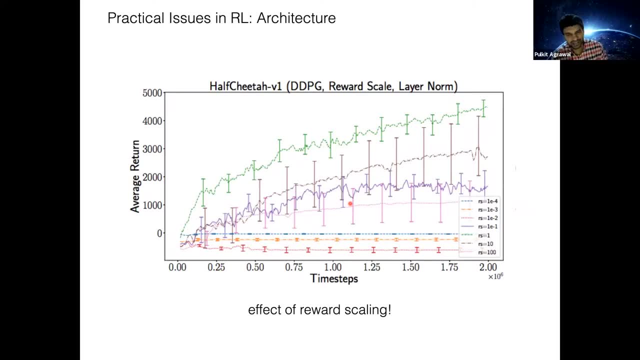 forth, Uh, and you can go to a bad. Okay, Uh, local minimum, right. So no, this is, with respect to DDPG right, Where we didn't really have any constraints, that the policy should be changing slowly. 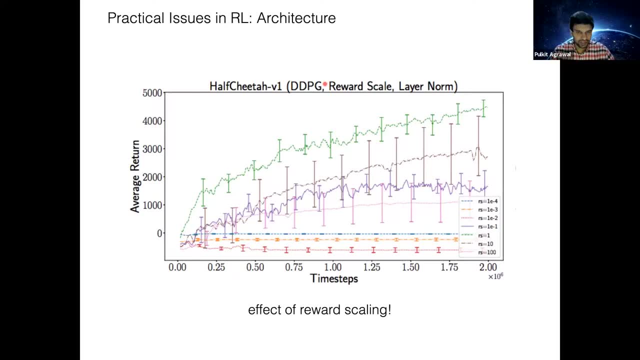 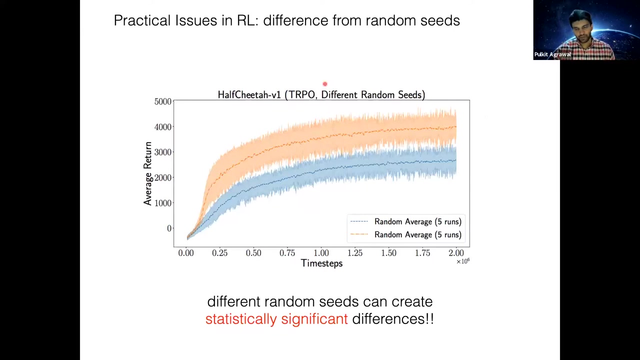 Right. So if you have no such algorithms, you know the scaling in the rewards can really affect performance. So you know the point being that you know small changes, Changes, can have a huge difference in performance. and to make things even worse, 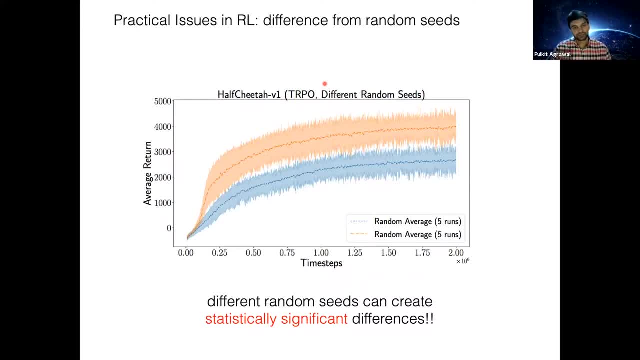 I think one thing which was noticed is suppose I take the same environment and then I run the RPO five times with five different random seats and I'm going to plot the result. I'm going to get that What I get is the orange curve. 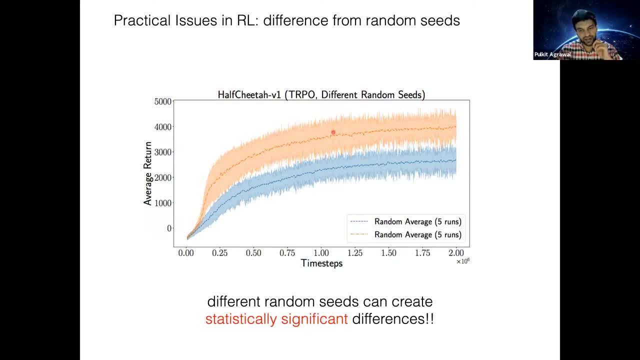 And what you're seeing over here is some variance in the performance. Then I do the same experiment. I run five more seats and what I ended up getting is the blue curve over here, with the variance that you know, with its variance, for the surprising fact, or not the surprising? 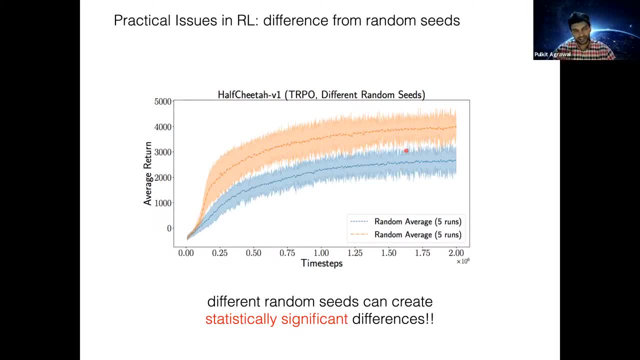 but the fact to notice that the difference between the orange line and the blue line is actually statistically significant. Okay, And what that means is that you know, there could be a paper, you know, which compares their performance with some previous state of the art, and they could get better performance. 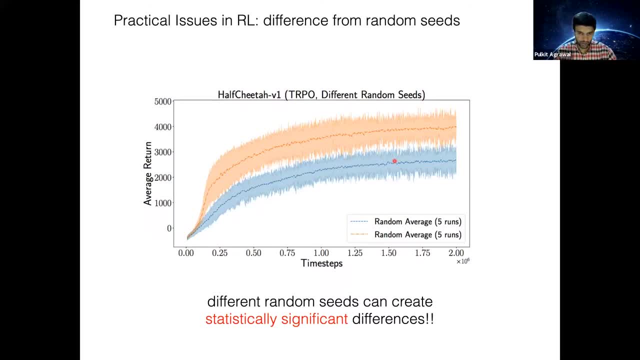 just by luck, because they only ran like two seats or three seats or five seats. So this, you know, raised a concern and this really shows that, why if you run an algorithm with one seat, Okay, And if you get some mean performance, that cannot really be trusted. you really need 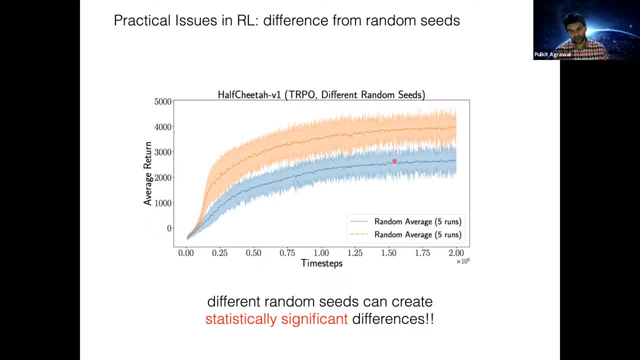 to run a large number of seats to trust the performance Right. So if you look at, if you look at the PPO paper, then they were reporting this as they were averaging it across 21 seats. So what this figure is showing you is that even averaging across five seats is not sufficient. 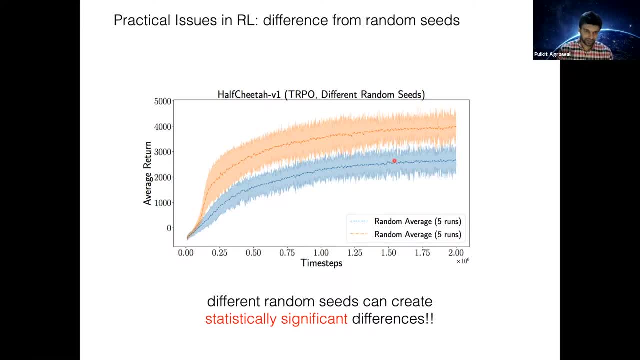 So if you were to, for example, write a reinforcement learning paper And you want it to get accepted at some of the top venues, And if you only ran, say, three seats or five seats, you know it's, it's very plausible. 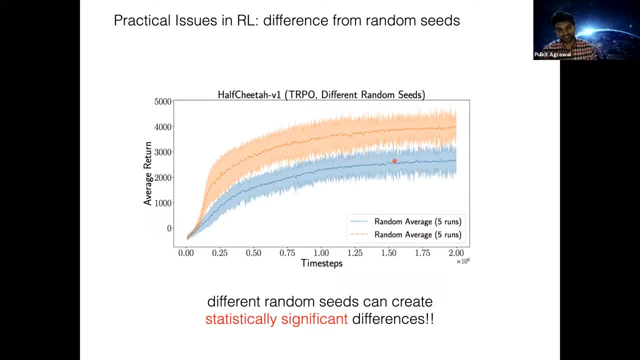 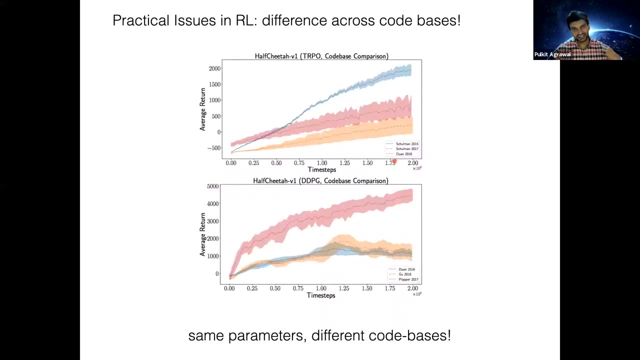 that the reviews are going to ask you to run more seats, because you know three to five seats might not give us enough confidence on the results And, to you know, make things even worse. Right, If I ran the same algorithm but across different code bases, one would end up getting different. 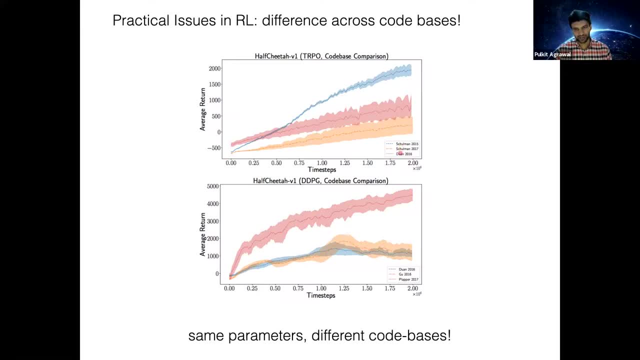 performances right. So this is showing you know, even from the same authors, you know two code bases in red and orange having different performance, and so the red and the blue and the orange having a different performance, which is different from other implementation. 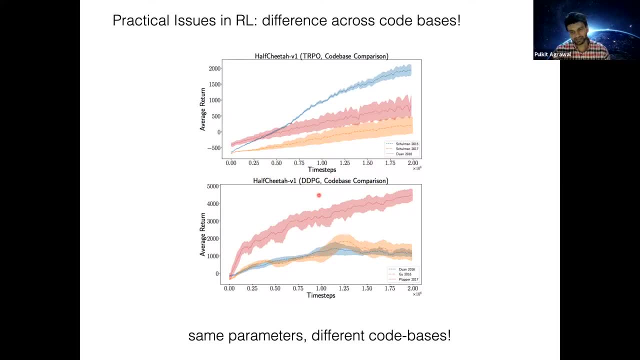 This was a TRPO, Okay. So similarly, in DDPG, you know, depending on the code base, there were differences. Now, you know, some of these differences were because, you know, one was in PyTorch there. 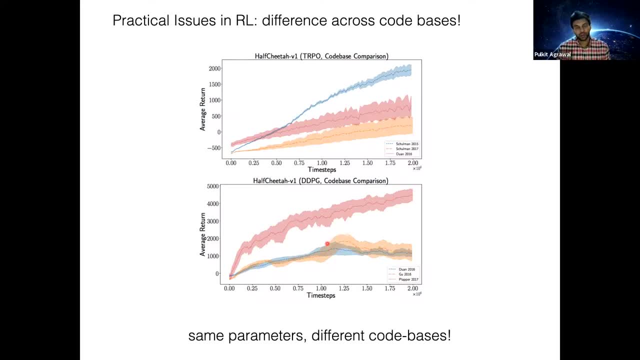 was in TensorFlow. So there were small changes which led to these differences. and you know other things. people were, you know still, you know, having a hard time trying to explain. you know what is causing differences in these. 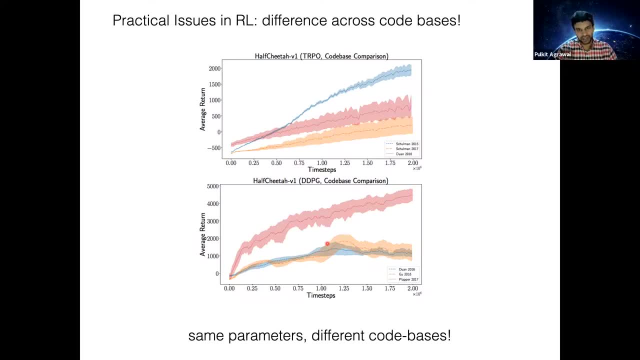 Code bases, Right? So, luckily, you know, we are not in 2017, you know any more, Right, I mean, we have now more stable code bases, which have resolved some of the issues. But what this tells you is that, if you're working on your problem and if you download, 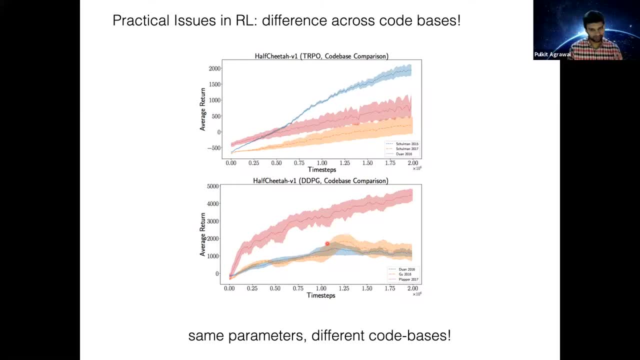 you know a code base, you know you, you know better. make sure that you trust the code base, Right? I mean just run it across a set of standard benchmarks and see if it can actually replicate the state of the art on those benchmarks. 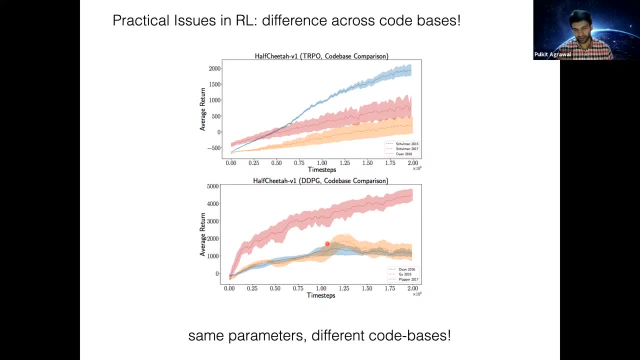 Because if you cannot, it means that you might be working with a bad code base to begin with. So it's important to have the right code base. It's, you know, almost critical if you're doing, you know research and you know some. 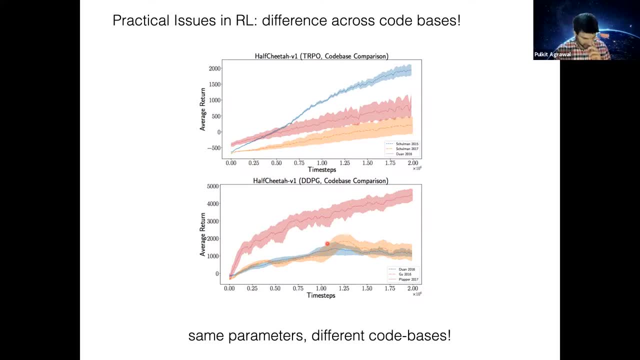 of the good code bases. I think we have it in lecture, I think four or five. you know the lecture on which was discussing about benchmarks. So if you go into the slides you know we have some references to what code bases you. 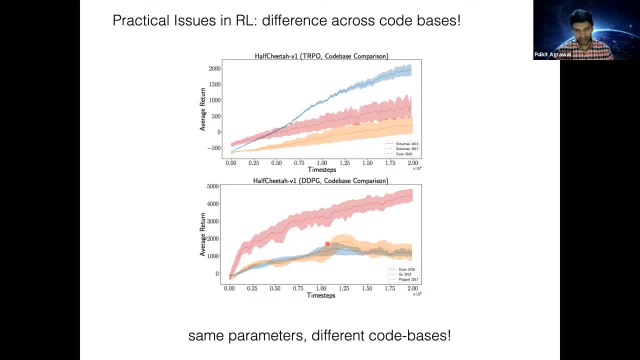 know we found to work well at at the present Right. So you know, before I move ahead. so now what I'm going to do is I'm going to look at, you know, these many different choices, Right? 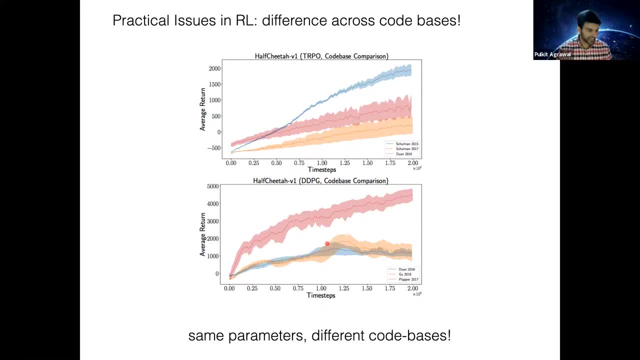 About network architecture, non-linearity and network architectures, optimization and so on with respect to PPO, and you know see what the recommendations are and what hyper parameter choices should we be using. But before you know we go into that, I'll take a pause and see if there are any questions. 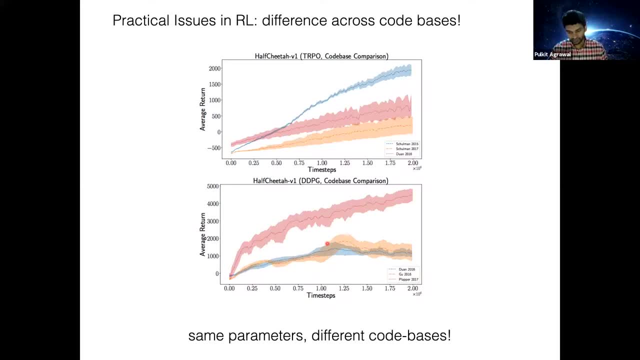 people might have. So I do see one question coming from Siddharth. you know how many seeds are generally recommended. So yes, I think you know some papers- I mean papers- still get in with, you know. 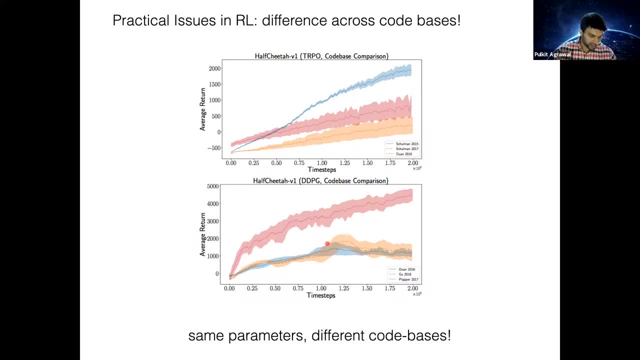 three to five seeds, but I think that should make you wary about the paper at least. So what you know, I typically recommend is you know once you are running your experiments. you know, maybe do you know five seeds, because doing more becomes problematic, but once you, 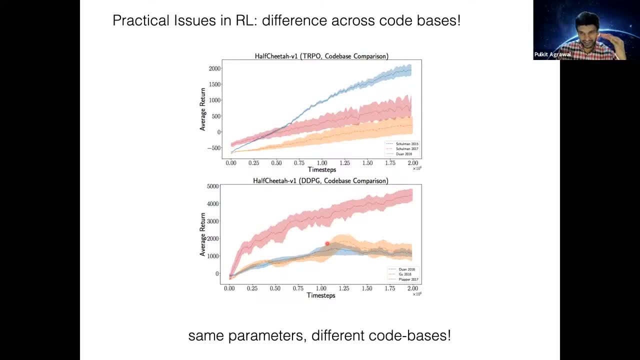 have to report in the paper. you know maybe do 10 or 12 seeds. you know when you actually have to report your curves in the final version of your paper. But you know, unfortunately there is no clear consensus on this at this point. 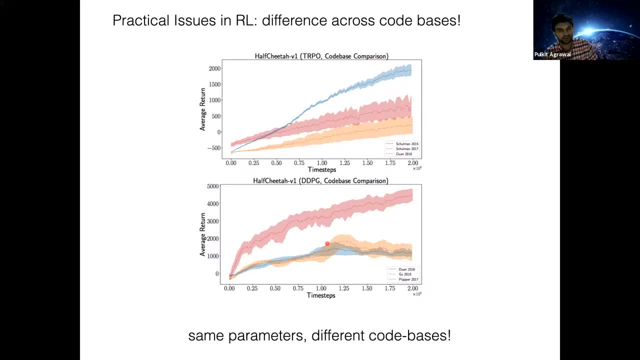 So I'm getting you know more questions about you know, is there a way to choose an architecture? I think we'll come to it, But you know any questions on the previous part? No, So I think you know this is the situation. 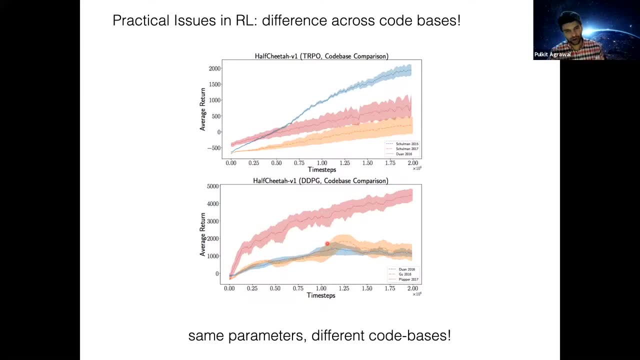 Okay, So this is the situation of a glass half full of water, Right? So in some ways, you know you could be, you know, optimistic, that you know these algorithms work and that they have, you know, achieved good results on a bunch of benchmarks and 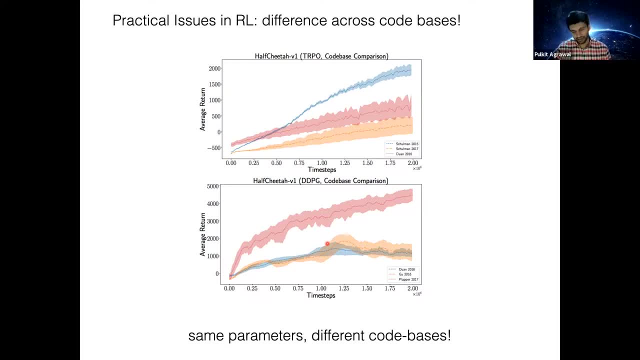 even exceeded human performance. On the other side, you might be very sad that these algorithms are very sensitive to the hyperparameters, So it's really unclear. You know how to use these algorithms for your own task or how to, you know, innovate? 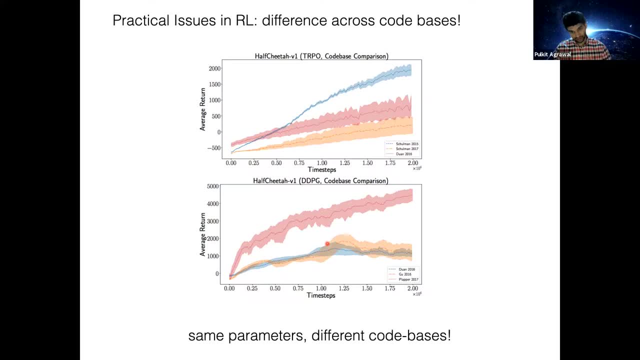 further. But I mean, I guess the good news is that you know there's a lot to be done. So there is, you know, some hope that reinforcement learning algorithms can solve, you know, really challenging tasks from high dimensional state spaces. 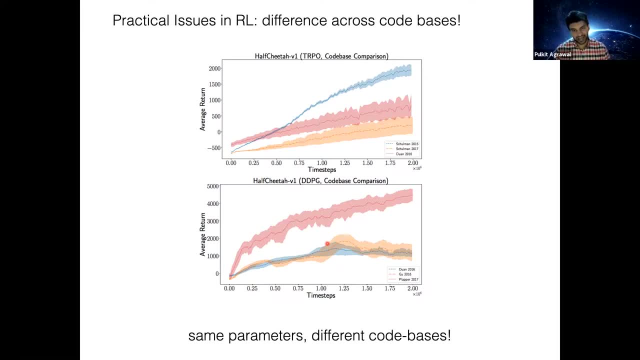 And there's enough work to be done, or a lot of work to be done, Right, To analyze, you know, why are they unstable, to make them more stable, to improve upon them. Right, So you can think of, you know a large part, or maybe, as you know, maybe, like you know, 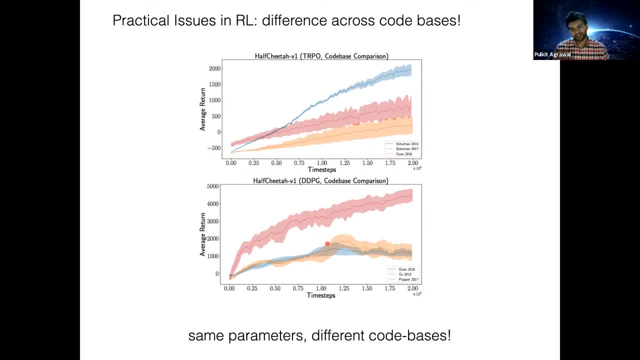 five to six lectures of what we'll be discussing is: you know different ways which can help reinforcement learning Right? I mean maybe by making use of demonstrations, By learning models, and you know doing things like domain randomization. you know how can? 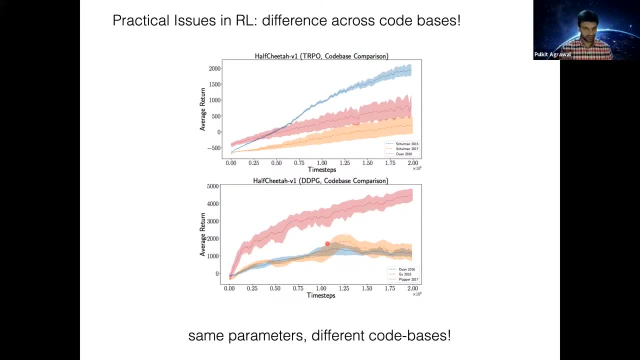 we leverage large amounts of data which may not be available in the real world, but you know, maybe in simulation, and how we could, you know, by turning in simulation, then transfer to the real world. So we will, you know, look at multiple ways in which some of these 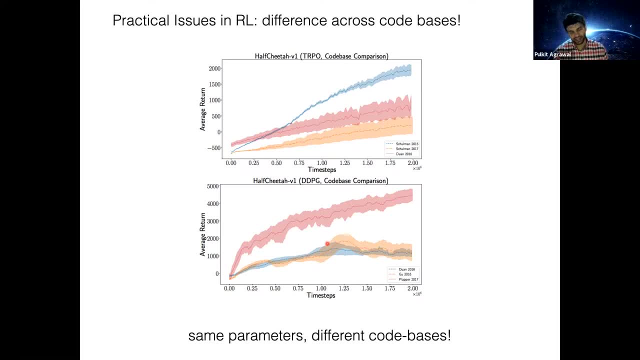 Some of these issues can be resolved by modifying reinforcement learning with some more supervision. And obviously there is another line of work, which is how do we look at algorithms themselves and try to improve them? Right, So that would be, you know, for example, starting with policy gradients, then realizing that 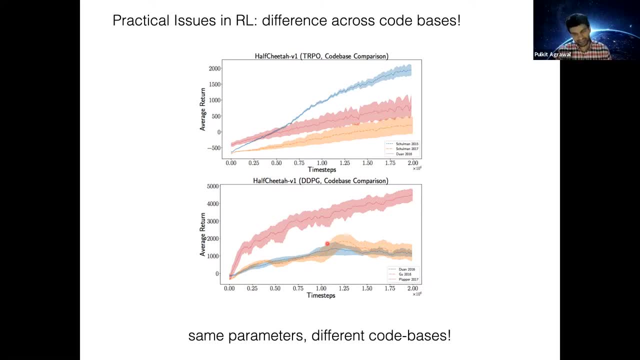 causality can reduce variance, Then realizing that baselines can reduce variance, Right, And then you know building up in that particular way or with the choice of, you know, parameter alpha, which was a learning rate. you know how do we choose it. 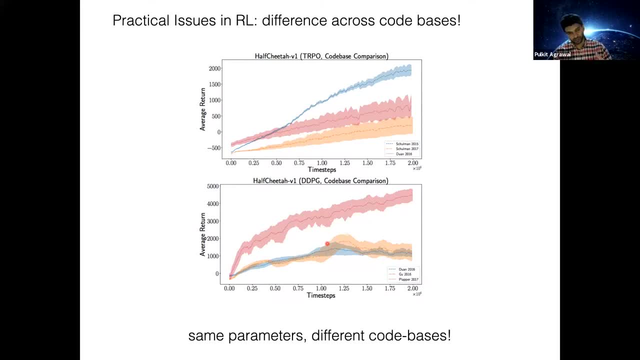 And you know that led from policy gradients to. you know TRPO and PPO. So the good news is that TRPO and PPO are actually much better than doing reinforce or just doing policy gradients without them, Right. But you know, maybe the difference between TRPO and PPO is not that significant in itself. 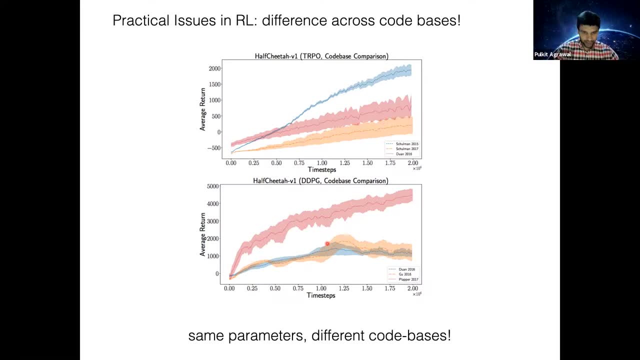 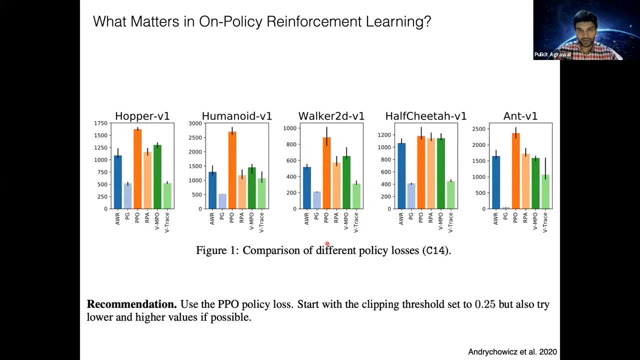 Right. So you know, with that pollute, let's look at. you know what actually matters in on policy reinforcement, learning. So it's an excellent paper by you know. it came out last year and they did, you know. 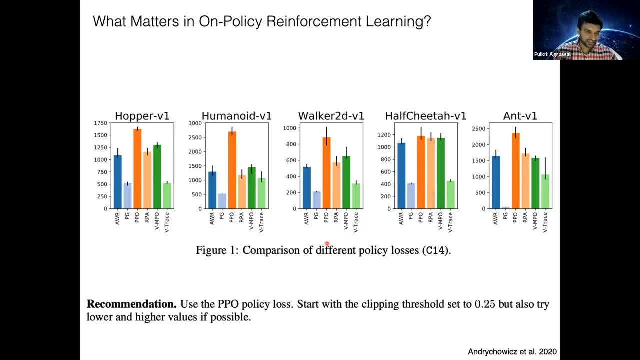 large scale experiments, Analyzing what is the best on policy algorithm, And you know what are different design choices which are critical. So there's a disclaimer: you know all these evaluations are done on these control tasks which do not require high dimensional observations coming, for example, images. 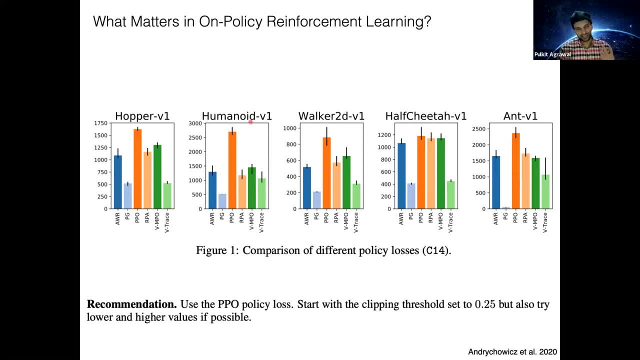 Right, And these, the dimensionality over there is, you know, still not super low. It's, like you know, some tens to 30 dimensions, but not, like you know, having a hundred plus hundred image. So you know, that's a grain of salt that you should take all of these results with. 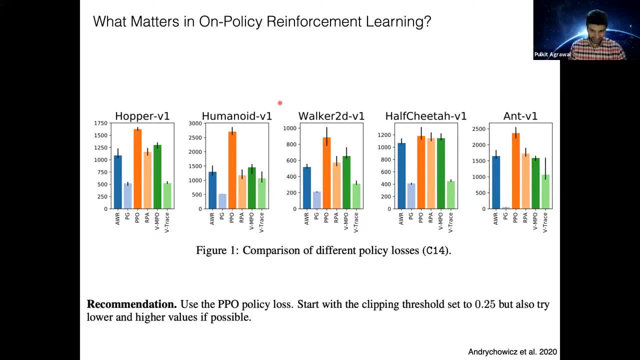 But I still think there are some useful insights to be gathered from this work. So one thing you know, that you see across the board, Is that PPO is doing much better than which is an orange is doing much better than you. 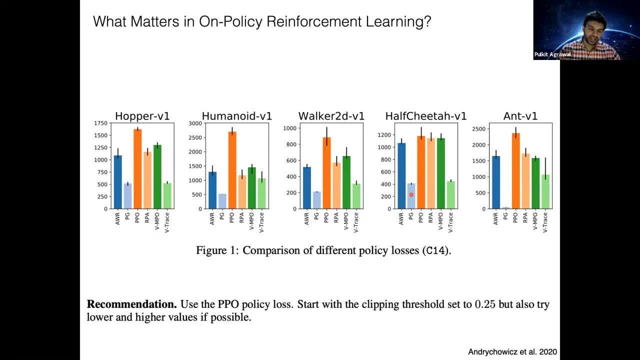 know this light blue, which is policy gradients Right, And PPO in general is doing better than most other variants of on policy RL algorithms, Right. So if you were to blindly, you know, pick up an on policy RL algorithm, you know PPO. 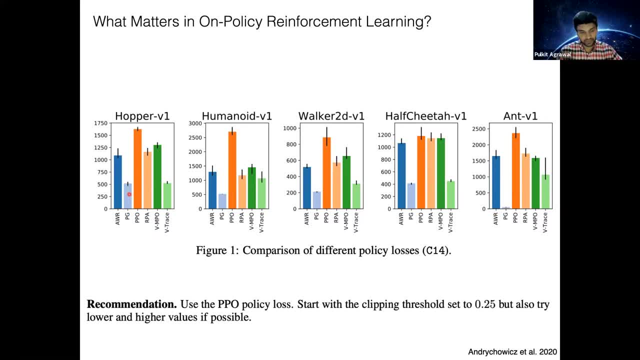 is a safe bet To pick up Right. So the concrete recommendation is: you know, use the PPO policy loss. you know, start with the clipping threshold of 0.25, but it's a hyper parameter that you can vary and see. 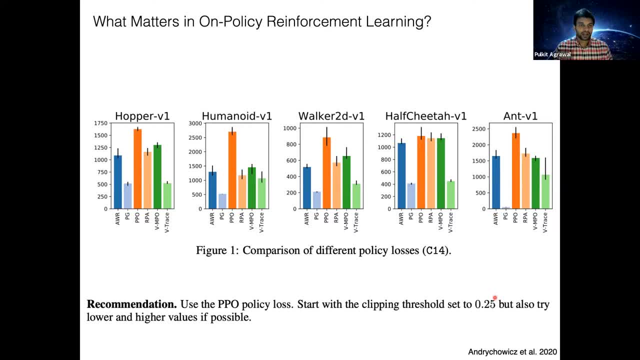 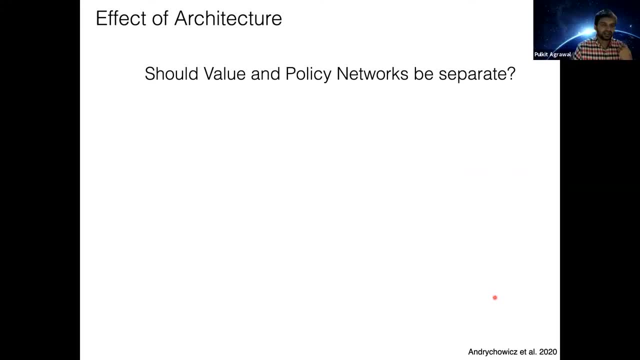 how it affects performance, Right. So a second question you can ask is: you know, should I have the same network to represent value and policy, Right? For example, you know I can have my state coming as input, I can have some layers which process my state and then I can have two heads, one a policy. 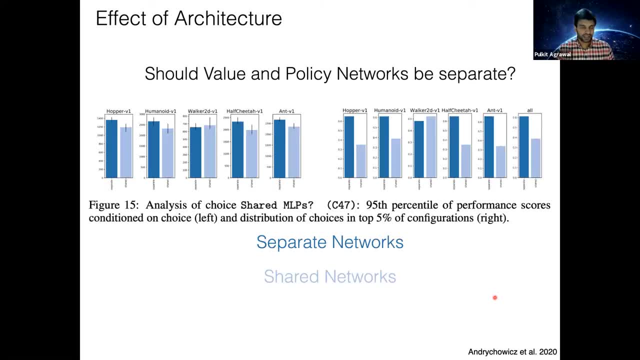 head and a one a value head, Right, And you know, on the left. what I'm showing is the performance which is for: dark blue is separate networks and light blue is shared networks, Right. So it's pretty clear that separate networks is leading to better performance. 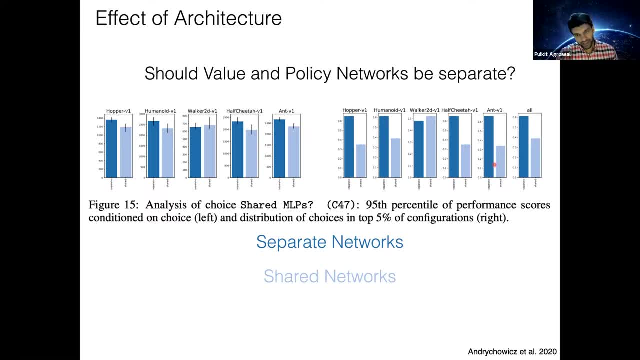 On the right. I'm showing the same thing but in a slightly different way. So instead of plotting performance, what we are plotting over here is that if I just take, if I ran, say, 100 experiments, if I just pick the top five experiments, then in those top 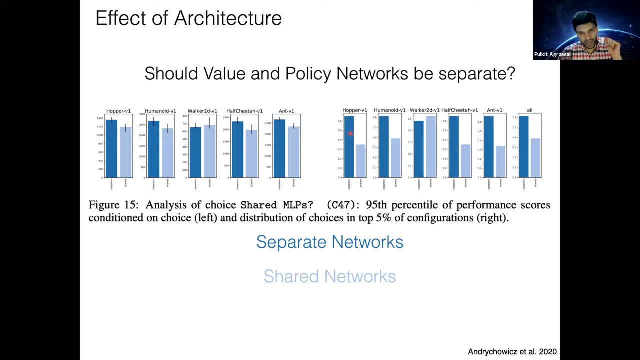 five, how many of those had separate networks and how many of them had shared networks? Right, So what is the fraction of you know, the top five percent performing setting of hyperparameters? You know what is the ratio of separate and shared networks. 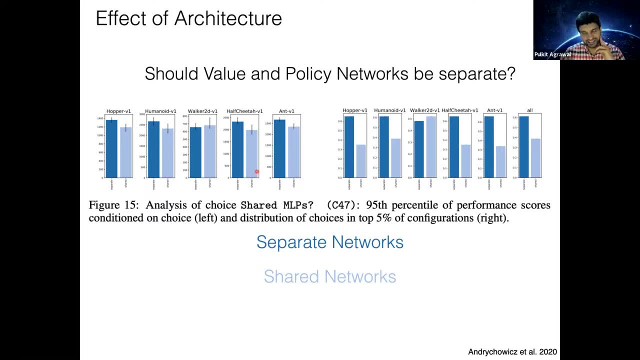 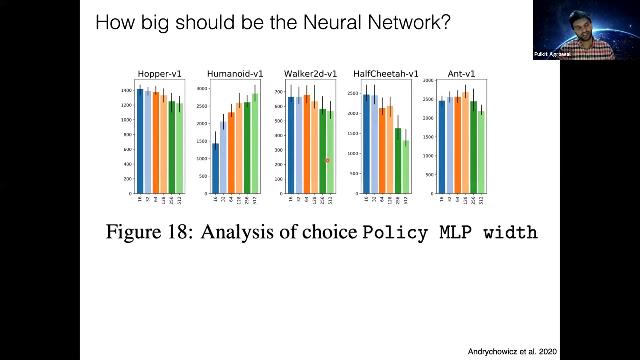 Right? So is this a different way of looking at the same thing, Right? And so the concrete recommendation is: you know you should be using separate networks for the value function and the policy network, Right? So, similarly, a question comes up: is you know how big should my new network be? 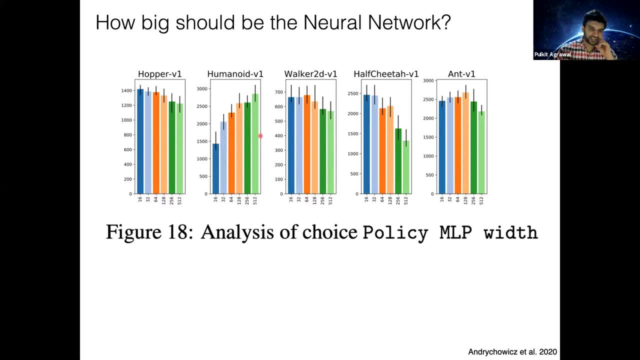 Now, you know, if you look at these different tasks, so all of these are feed forward networks, And what we are varying is the width of each layer, And turns out that, you know, there is no clear consensus Right On what is the optimal network size. 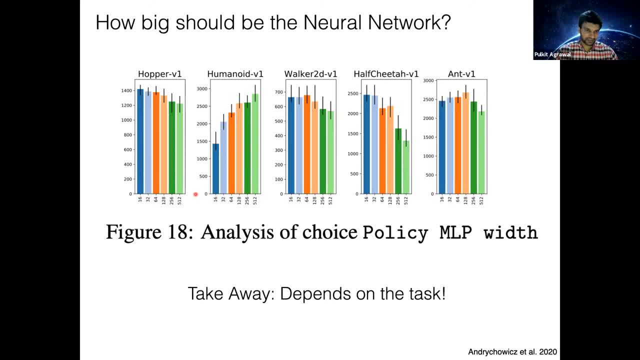 Right In some ways. you know it depends on the task. And the sad thing is, you know, maybe something which works, you know very bad or not, or is worse for Hopper, ends up being the best for humanoid. 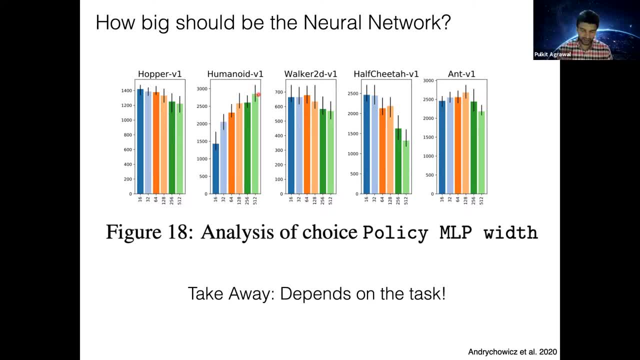 Right. So the takeaway? I mean there is no clear consensus on what is the right neural network. Right now, the neural network is very, very limited, Right. So you know, if you look at this, you can see that the architecture does affect performance. 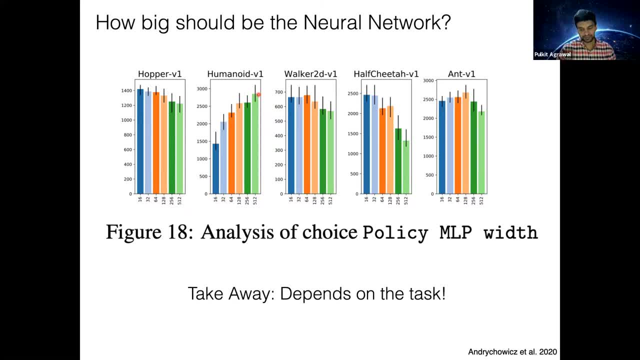 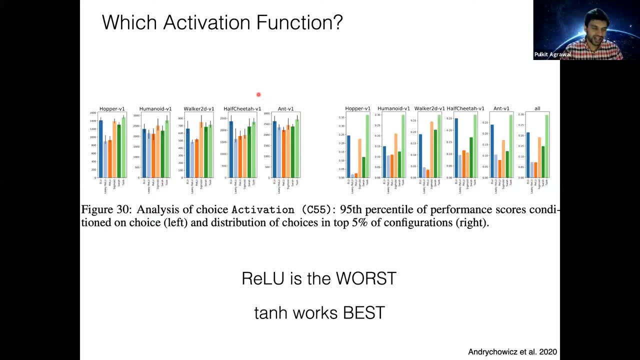 and you will probably have to tweak the architecture for your task. Now, a second question you know you can ask is: what is the activation function that we should be using? So you know, you can look at these plots, And I'm going to concentrate more on the plots on the right, which were showing the fraction. 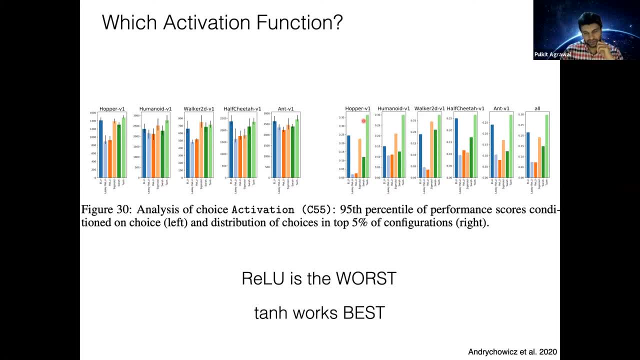 of the different activation functions end up being the best. So you can see, tanh ends up being a very good activation function and relu actually is much worse than tanh Right. So that so, if you are, you know, working with, you know working with the state space. 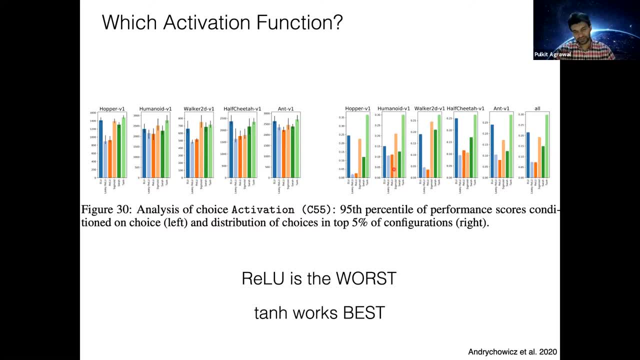 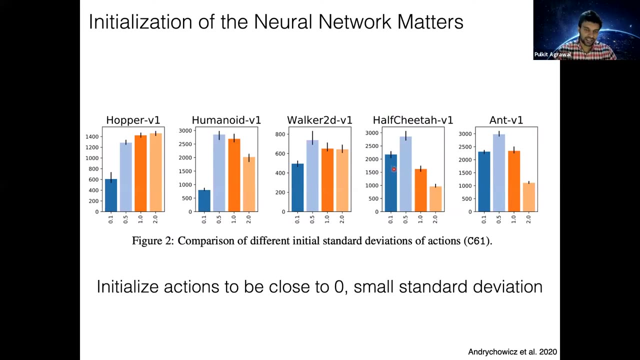 which is not you know, say, vision, inputs and so on, banished non-linearity is, you know, it's the first thing to start with and it's probably going to work the best, Right. And the other question you can ask is: well, I have set up. 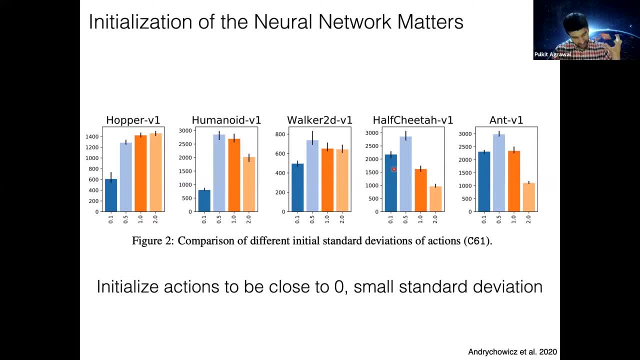 my architecture. you know I chose a number of layers. you know there's something on the activation function, but now I'm going. I need to initialize my new network. So how important is the initialization, You know? so I think you know it's pretty clear looking at these curves. 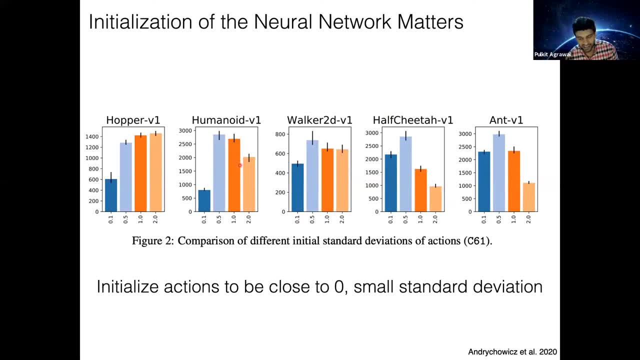 that initialization is important, And the concrete recommendation is, you know, initialize the actions to be close to zero and have a small standard deviation, And that you know pretty much works quite well, Right So, which you know corresponds. 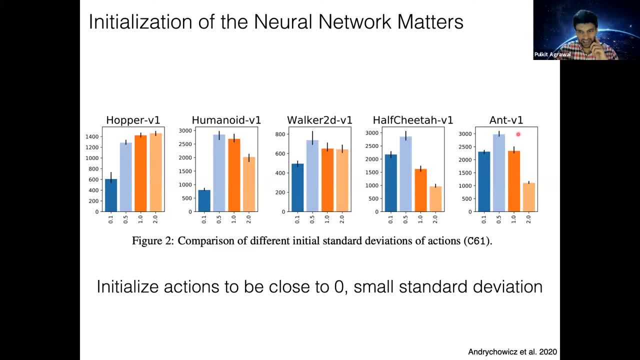 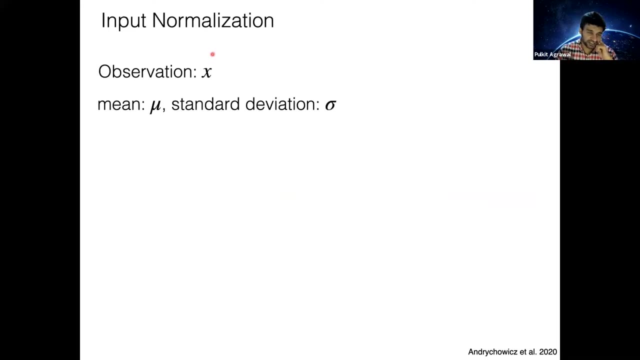 you know, maybe 0.5 in these you know plots over here. Then the other question you can ask is: well, okay, I've initialized my new network, but what about my observation? Right, So suppose my inputs are X and suppose my mean observation is mu and the standard deviation is sigma. 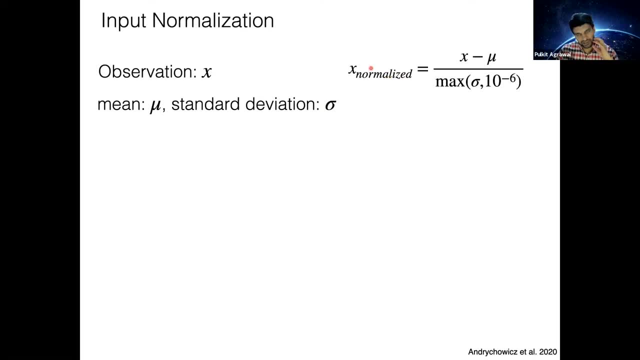 then I can normalize my observation in the following way: right where I subtract the mean and divide the mean by the standard deviation. So I can normalize my observation in the following way: right where I subtract the mean and divide the mean and divide the standard deviation. 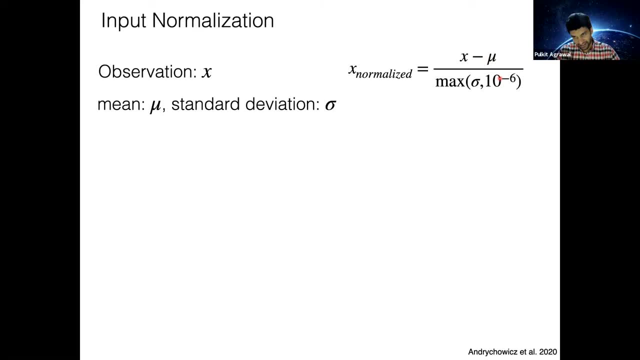 Now you might realize there's a funny number: 10 to the power minus six over here. Now this is for numerical stability, Right? For example, if some observation or some feature does not change, then sigma is going to become zero, which is going to create numerical instability. 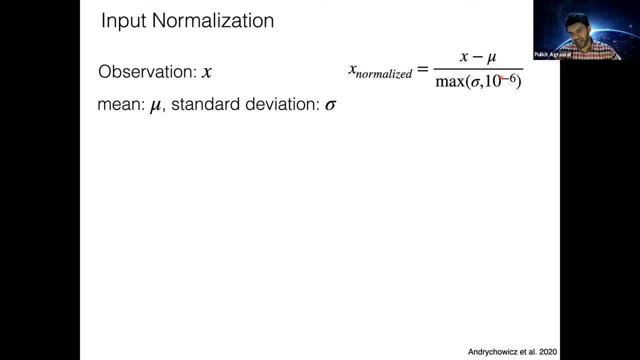 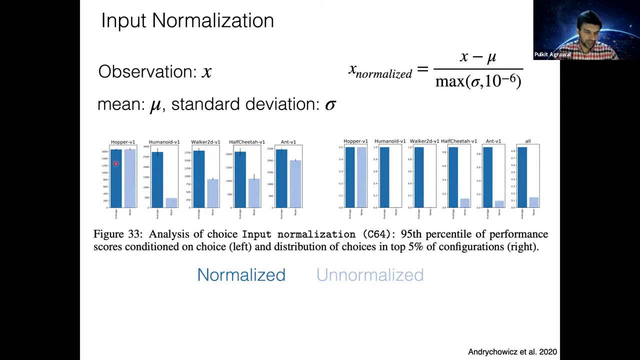 So, therefore, whenever you're dividing, you know these terms are a good practice for numerical stability reasons, Right? So it turns out that you know such normalization is quite important, Right? So if you see, the dark blue curves are normalized ones and the light blue are the unnormalized, 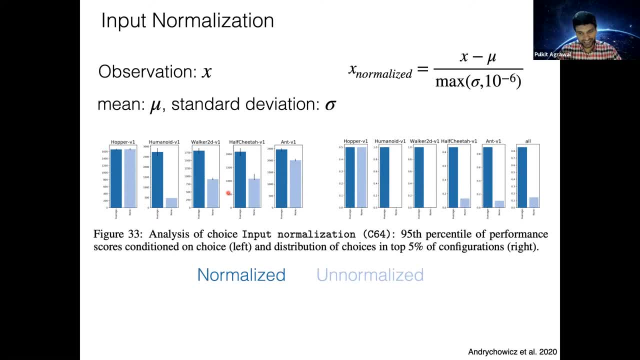 For most environments it is a significant factor, whether you normalize your observations or not. So you know. when I said you know the difference between TRPO and PPO goes away because of you know code length. So you know the difference between TRPO and PPO goes away because of you know code length. 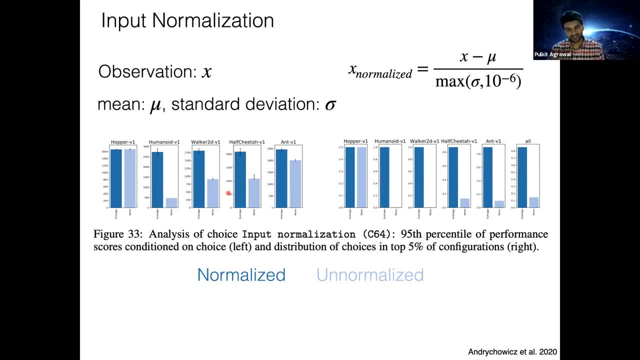 Level optimizations. This is exactly the kind of things you know I was mentioning or I was referring to, which is, you know these choices Right? I mean, do I normalize my observations or not, You know? or how do I normalize it, How do I normalize my reward function, So on and so forth. 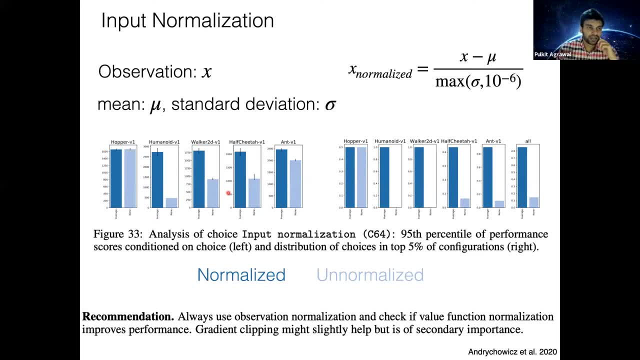 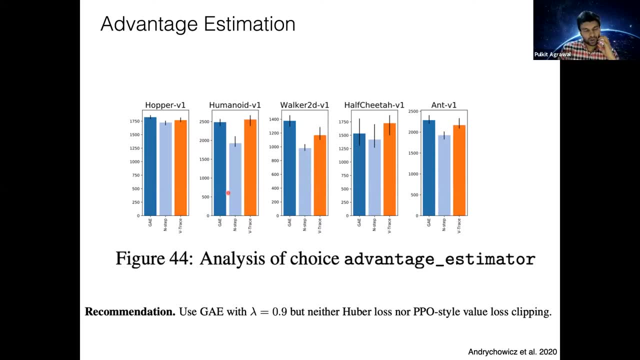 So yeah, Now the other question you know you can ask is: when I'm doing my advantage estimation, how should I estimate my advantage, Right? So remember, we could estimate the advantage directly. We could estimate the advantage by using generalized advantage estimation of GAE. 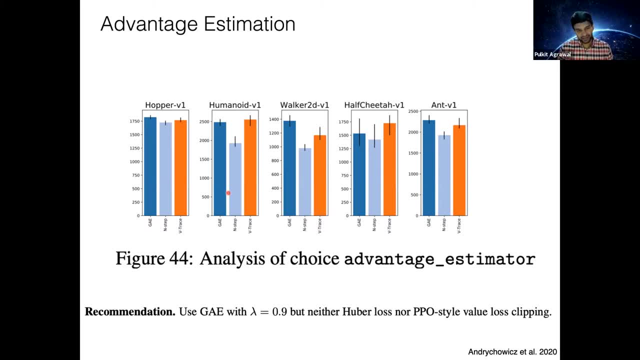 that we covered Right. There's also N-step that we can do. So what is N-step? N-step is, if I take the sum for N-steps, for example, it's like R1 plus R2 plus RN, And then I bootstrap from the value function, So it will be gamma to the power N plus one. 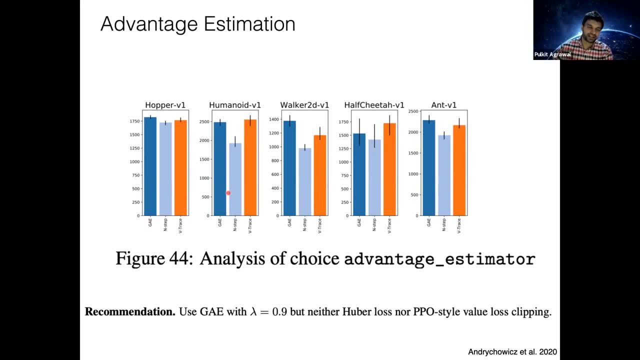 V of ST plus N plus one Right. That was N-step. So one step is when I do V of ST plus one is RT plus gamma times V of ST Right. So and then we saw that generalized advantage estimation does a good tradeoff of bias and variance Right. 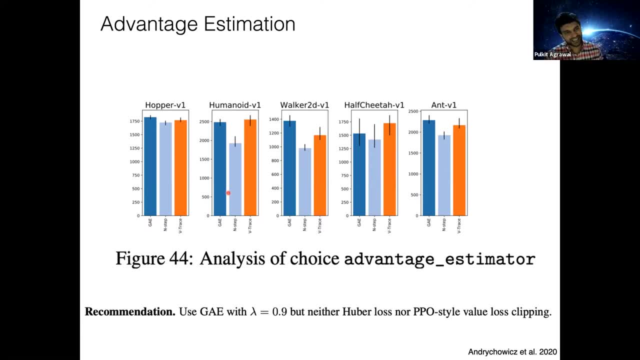 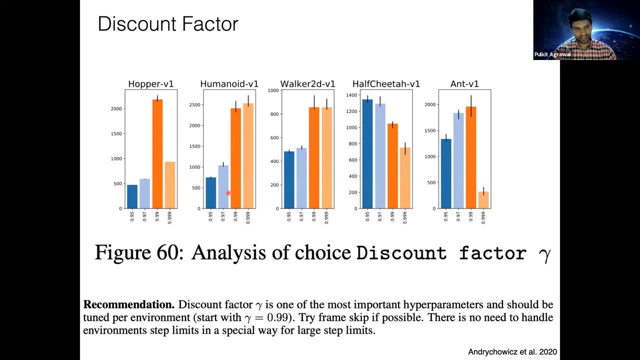 So it turns out that you know, using GAE is indeed one of the best ways to estimate the advantage function, And you know you should be doing that. You know similarly, the other factor which becomes important is defining the discount factor. 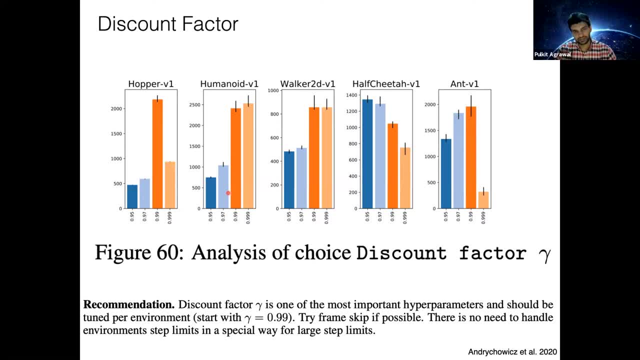 Right, So you know it turns out that the discount factor choice depends on the task. Right, So you know it turns out that the discount factor choice depends on the task. So you know, such it's not so surprising because 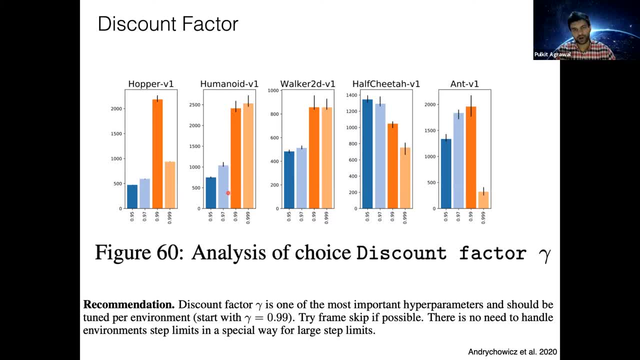 this discount factor really depends on how long horizon, of how short horizon your task is. So this does end up being task specific, Right, And this is one of the most important other parameters If You know you're implementing your agent. so something to note. 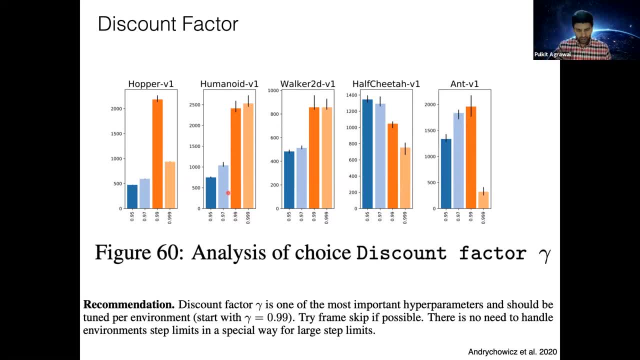 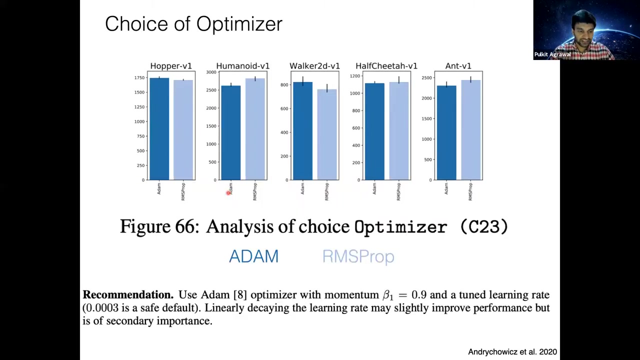 and also something to realize: that that you know there is no concrete guideline on what discount factor should you be using is something that you will have to vary and then figure out right. then you know. other question which comes up is: you know what is the optimizer that one should be using. so the recommendation you know again is to use ADAM, and you know they. 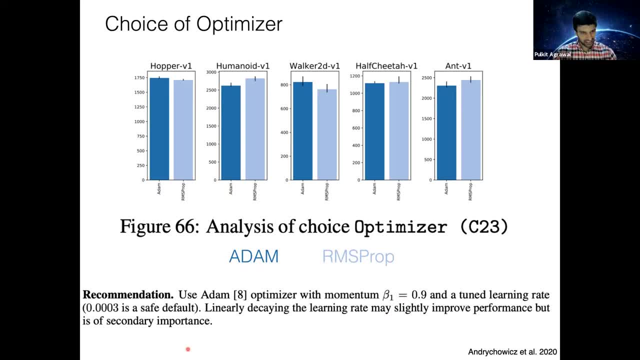 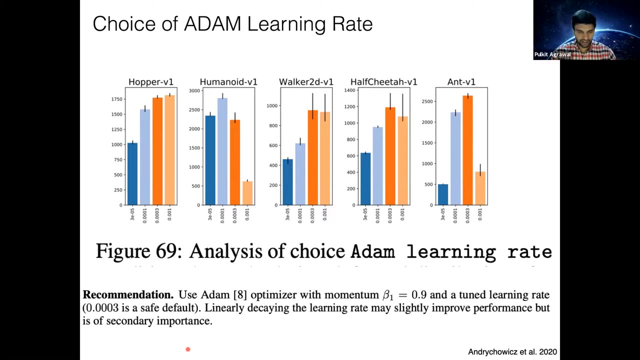 have some recommendations on some parameters of ADAM, which I mentioned in the bottom. so if you're using ADAM, you are pretty much good. if you're also using PPO, right then you know. the other question was about what is the learning rate that I should. 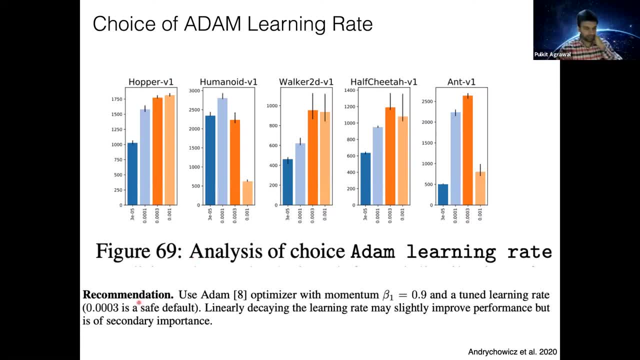 be using. so the one is item okay, item okay, item okay, you know. the other question was about what is the learning rate that I should be using. so the one is item okay, item, okay, item. using an atom. And you know, they point out a value which is 0.003, which is seems to be a 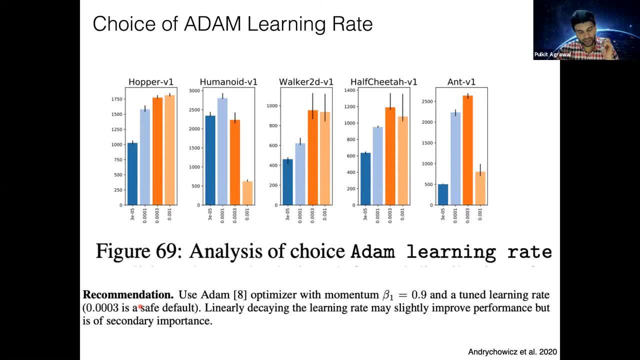 safe default value. But note, you know I mean these. all of these things are interdependent. For example, if you scale a reward in a particular way, that's going to affect how you choose a learning rate, right, Because if you make your reward be 10 times, then it means that you now 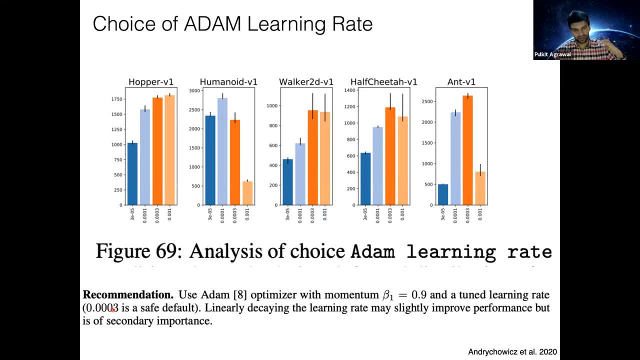 need to make a learning rate be 10 times lower. you know, like in a ballpark way. So all these choices are intertwined with each other, right? So these you know recommendations kind of go together in a bunch, right? You cannot just, you know, apply some of them and not apply the other. 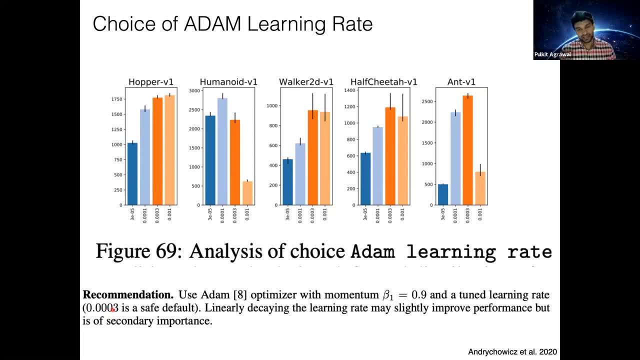 ones, Or if you are going to change them, then you know you should think about. you know how things are going to get affected. You know, for example, if you're scaling up the rewards for some reason, you know you need to. you know have, you know, have something in the back of. 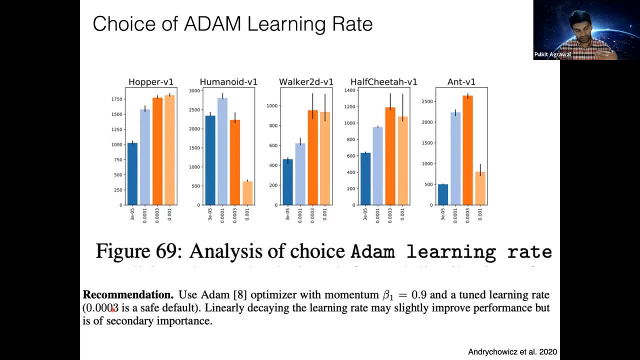 your mind that is going to change. You know, maybe if I found some optimal learning rate for a particular reward scaling, that learning rate may not work if I change the reward scale, for instance. You know. then you know there is some you know guidelines on. 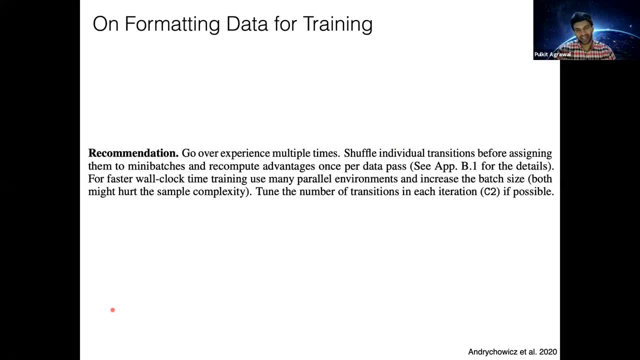 you know how to format training data and how we can, you know, get you know faster wall clock time. Now, these didn't end up being so significant But, you know, I would recommend the interested user or the student to go and you know, look, you know at the paper in more detail. 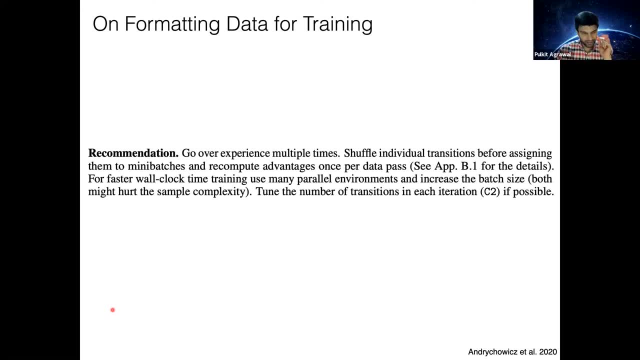 So some of these things are now, you know, have been implemented in the latest and greatest code bases. So you, you know, pretty much don't have to worry about how the training data is formatted. But you know, if you're doing research in the field, you know it makes sense to, you know, look at it. so 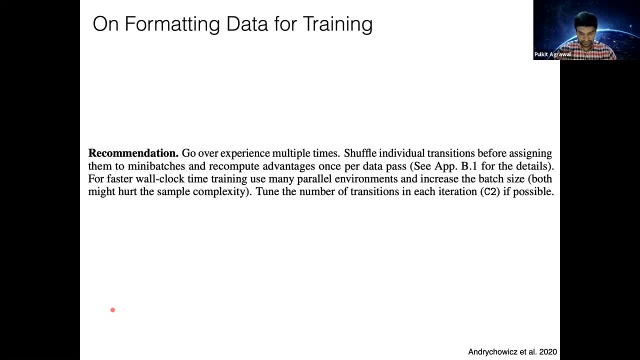 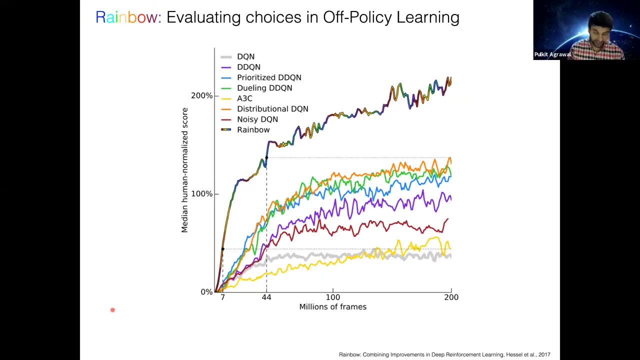 that you understand what's happening below the hood. So, similarly, I mean, just like you know, as we saw, the different, you know improvements or different recommendations that were made for on policy stuff. you know rainbow, So that we saw a couple of lectures before. also, you know, provided how different choices in Q 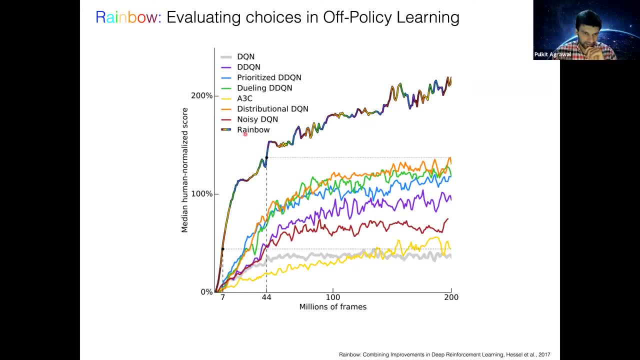 learning affect performance, right. So you know we saw how adding double DQN, how adding prioritization, how adding dueling was helping and how combining them leads to overall improved performance, Right? So yeah, so you know that's what I had on. you know, choosing hyper parameters in on. 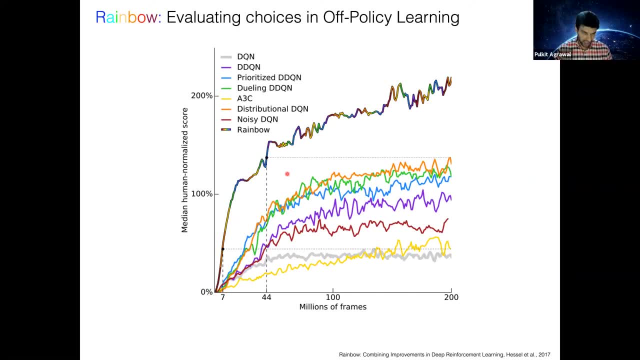 policy RL, And you know what things are, you know, important when you are doing off policy learning and what choices can help you improve performance. So now, with that, you know, I'll take a pause and see if there's anything else that you'd like to add to that. 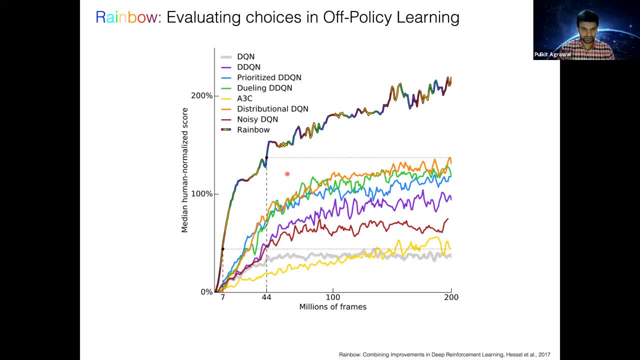 So yeah, so that's what I had on, you know, choosing hyper parameters in on policy RL, And you know I'll take a pause and see if there are any questions that people might have. So, Siddharth, you have a question. How are the means and standard deviations evaluated? 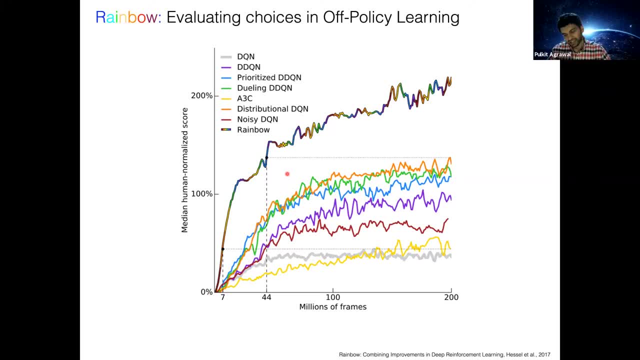 So you can evaluate them. you know for the batch, Or you know you could collect some random exploration data and use those values to calculate the mean in the standard deviation. You know both of them end up working. But even if you do batch level, if your batch is large enough, which typically is the case, 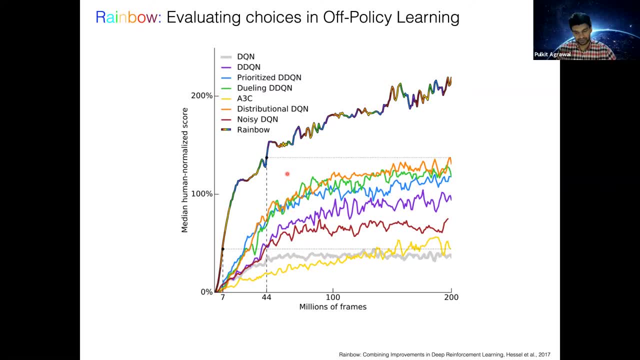 when you're using PPO. you should be fine. Any questions or any comments? No questions? Yes, I was wondering if, for example, if we are working in an area where the interpretability is prerequisite, why do we want to use a neural network? 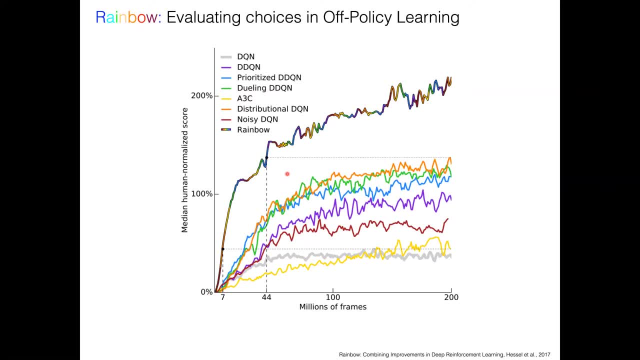 For example, why would that be possible to use, I would say, simple linear regression or simpler model like trees that could be interpretable to understand the model behind the? Because I feel it could be really efficient, but on the other way it could be. 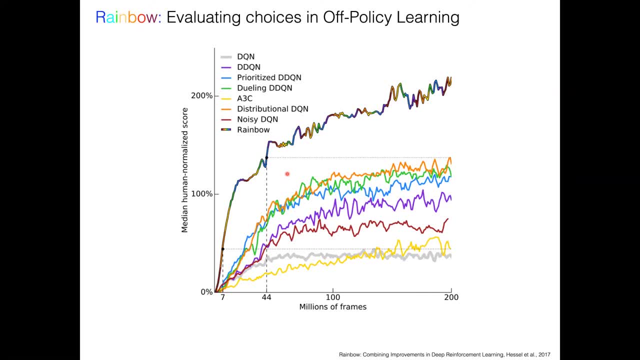 Also black box. I think the main reason for using neural networks is that decision trees or linear regression is just not as powerful as neural networks are, and so there are some functions you will not be able to approximate And in terms of Maybe, I think. 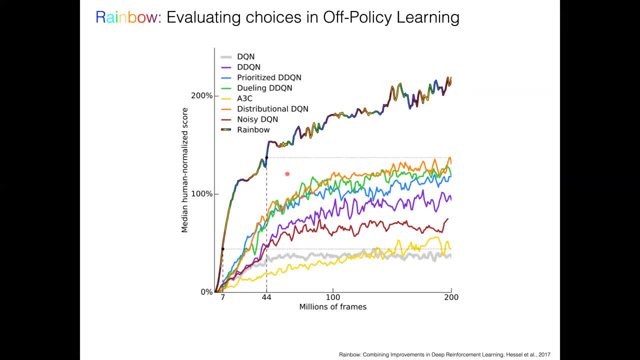 Is there a trade-off between? I would say, for example, if I need to be faster, Yeah, Go on, Yeah. If I want to be faster or I don't have access to a GPU, would that be possible to use a? 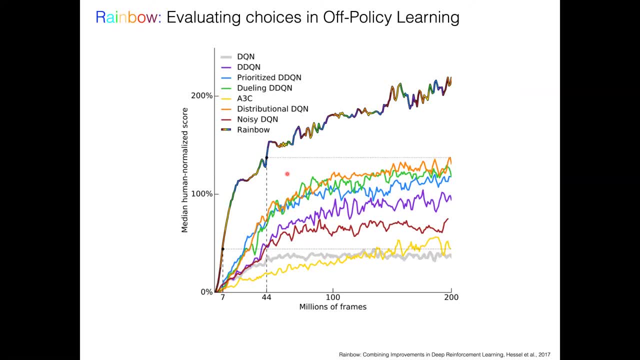 simpler model or neural network is a prerequisite here. So if you don't have access to compute, you could try to use a simpler model, but that might also mean that you may not get as good of performance. Yeah, Yeah, Okay. 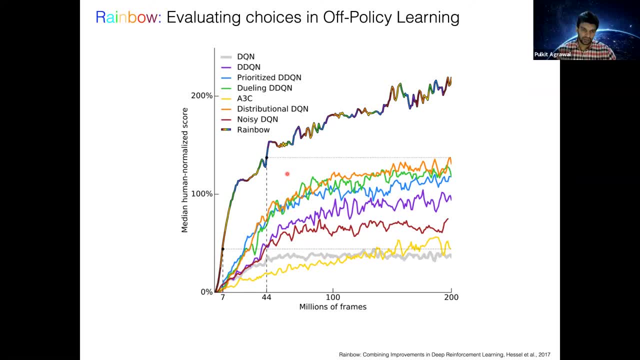 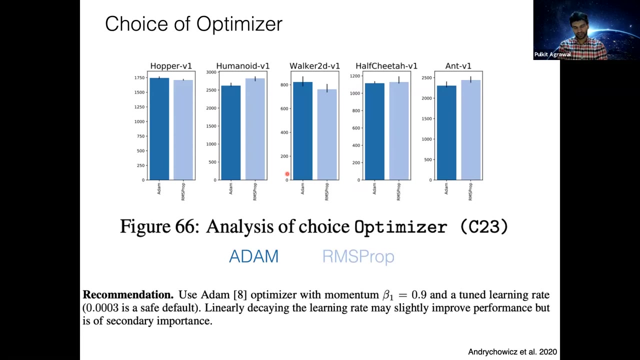 Okay, Thank you. So that's a trade-off. So I think the takeaway that you should have from this lecture is that we have come to an exciting point in reinforcement learning where things are starting to work. This is analogous to how deep learning was, maybe in 1980s and 1990s, where people could 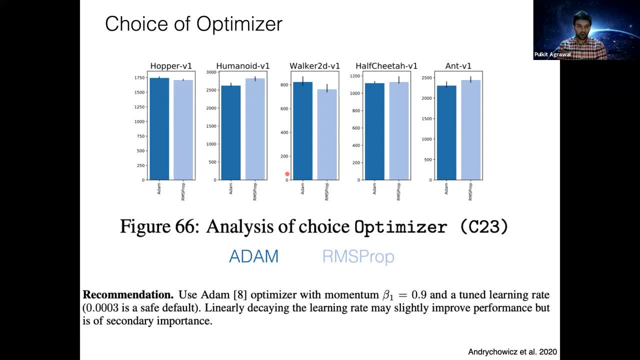 get things to work to some extent, But large parts of what is important, what is not important, was unknown. So I think reinforcement learning is undergoing that transition right now, where every day, every month, every year, our knowledge about what makes RL work and what doesn't make RL- 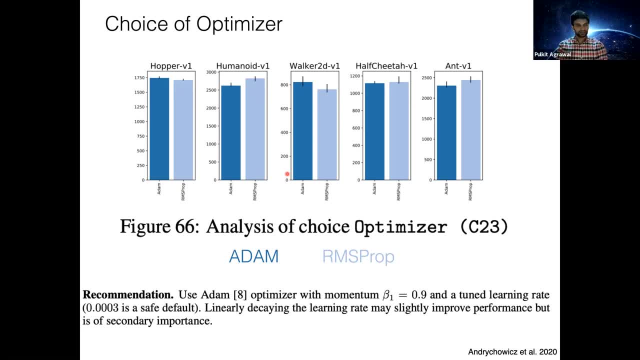 work is increasing. So if you want to do research in AI and you are excited to do research and you're excited to do RL work, then you have to understand that your knowledge is not only about RL but it's about the RL. 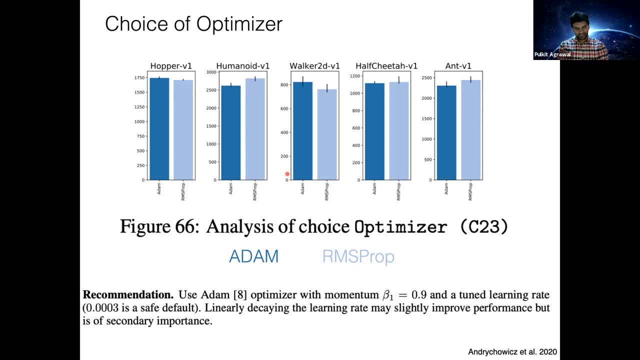 Because if you don't have the knowledge about RL, then your knowledge about RL is not going to work, And that's why our knowledge about RL isn't going to work. Right, Right, Right, Exactly. So I think reinforcement learning is a transition.